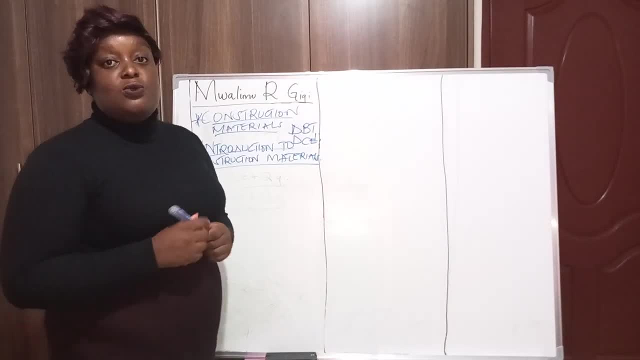 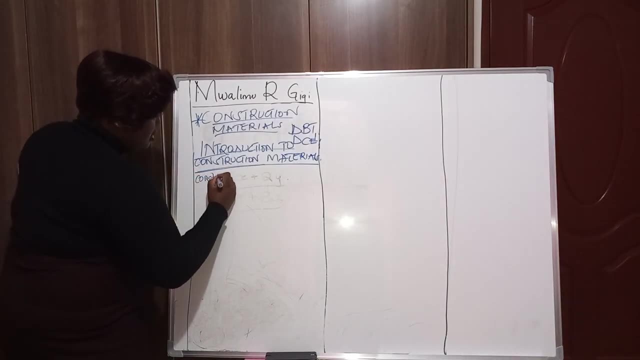 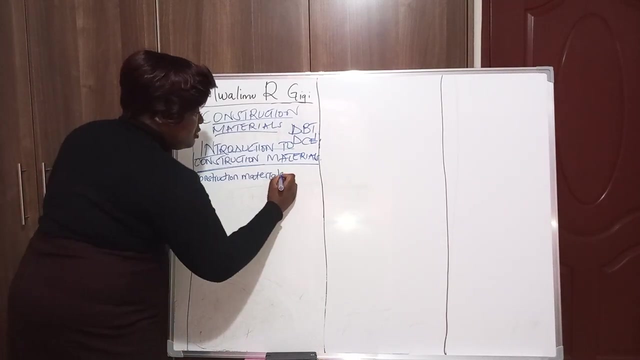 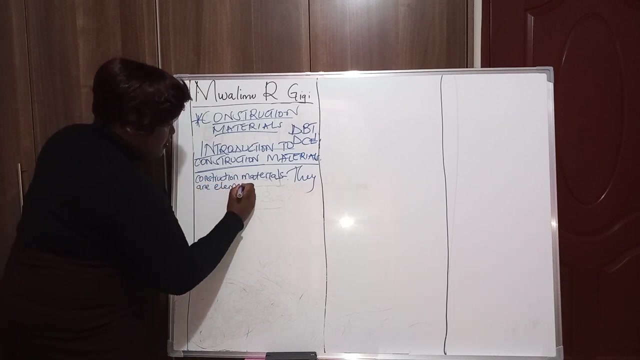 So introduction to construction material. First of all we need to know what is a construction material. So a construction material, construction material, a construction material materials, you can say construction materials. they are elements. they are elements, elements used in the. 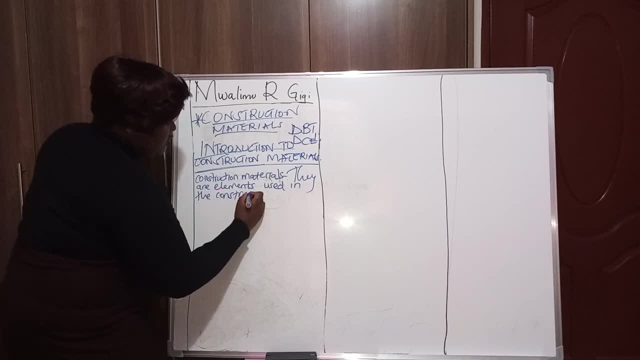 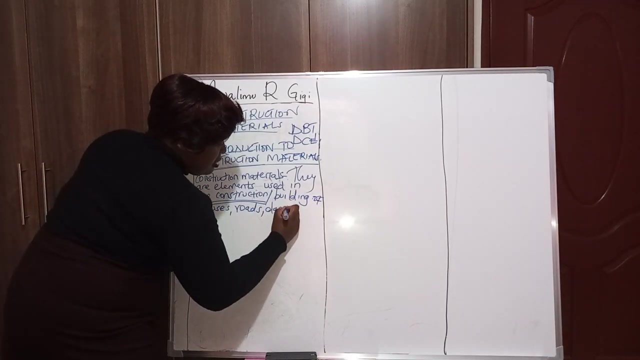 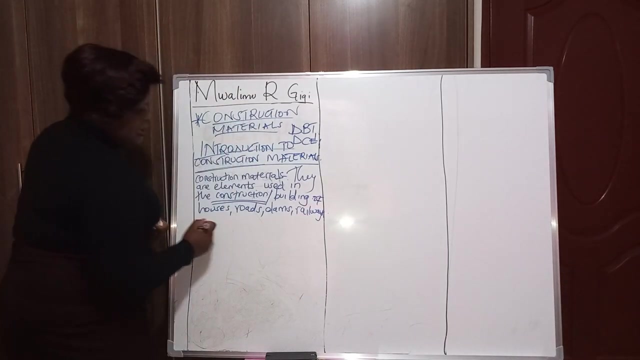 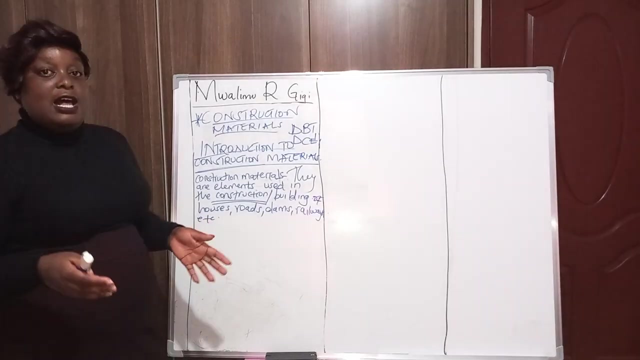 We can avoid the word construction, We can use in the building, So you can avoid this word construction In the building of, maybe houses, We have roads, We have dams, Maybe railways, So the elements, and we have ETC and many more others, So elements that may be used in the building of houses, roads, dams, railways and canals. We have tunnels and ETC. They are all construction materials. 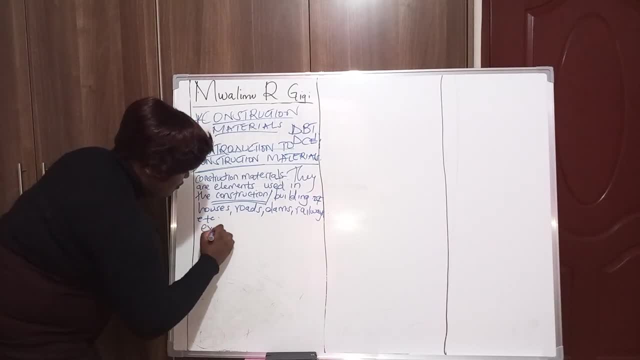 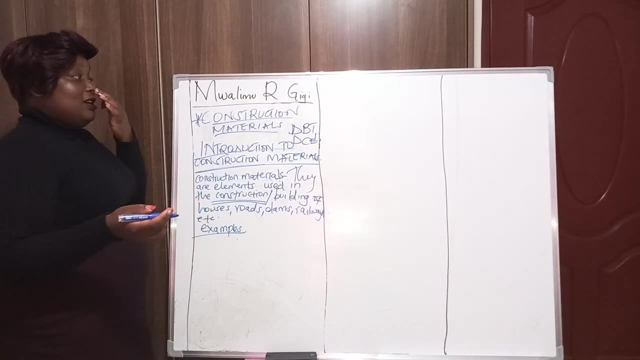 So what are these construction materials? You can see examples of construction materials or types of construction materials. They are just the common ones that we know. We have stones, Stones. These are just examples of some of the construction material that we know in the construction industry. 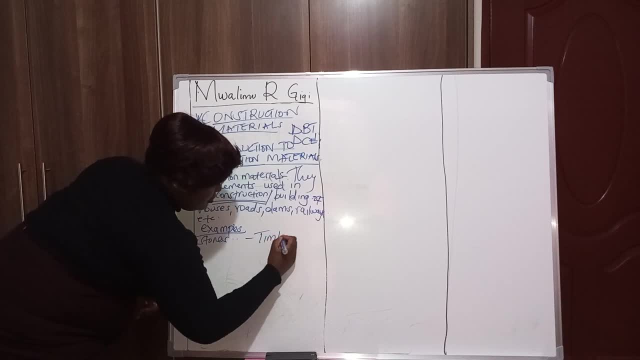 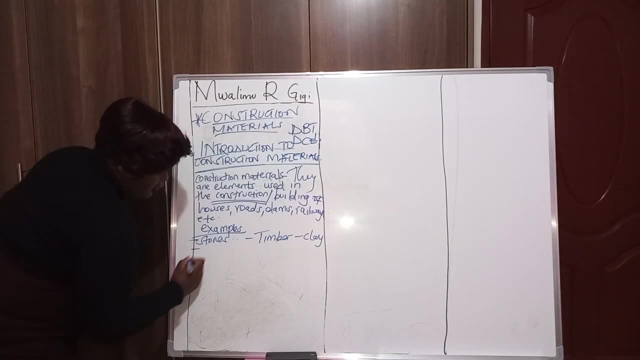 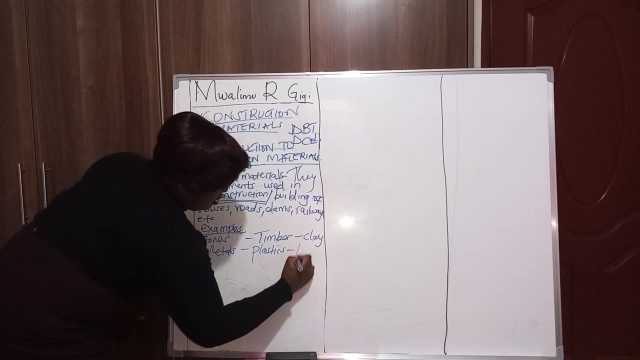 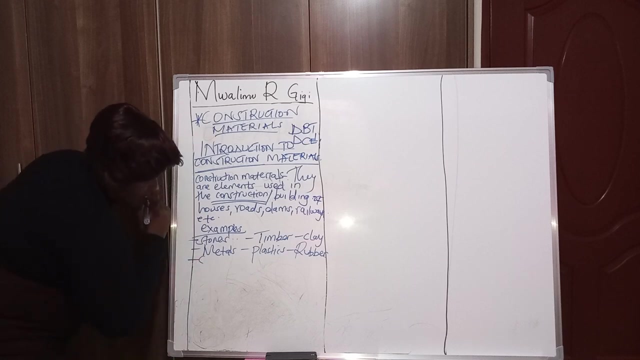 We have timber, We have clay, We can also say metals. We can also add plastics. Plastics, Rubber, All of these, they are construction materials. We can also add glasses: Glasses for glazing, doors and windows. We can have glasses. We also have paints, Paints and varnishes. 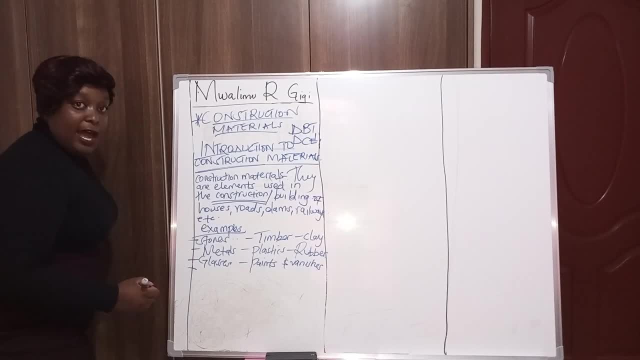 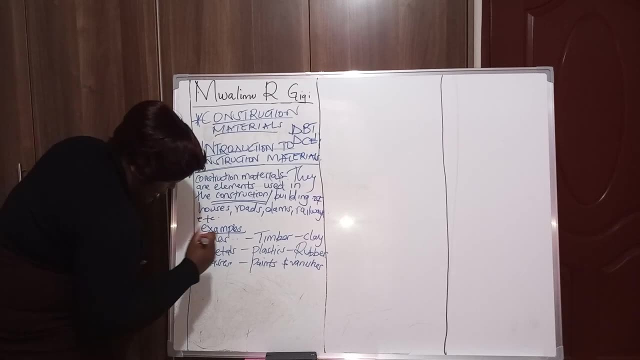 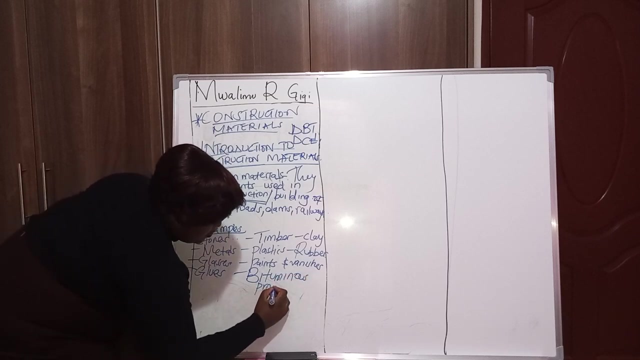 We can add more. We can add glue glues. We can also add bituminas, bituminas products, Bituminas products. These are like for laying In the church. These are different models of this picture, beautifully trampling. 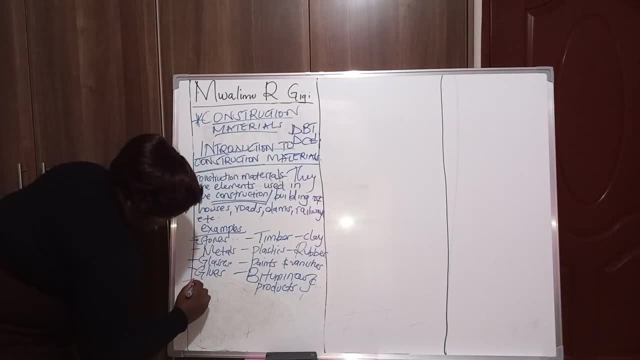 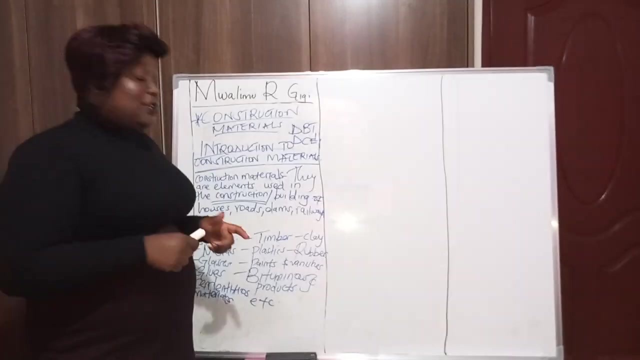 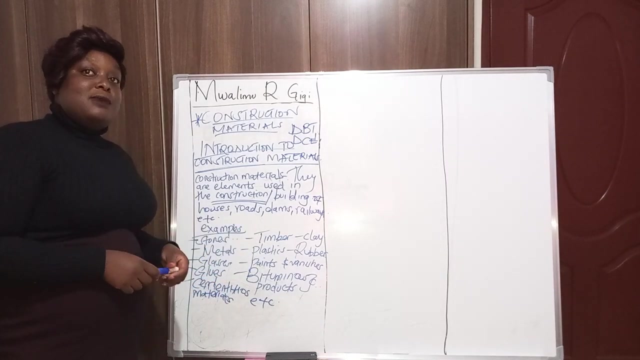 We can also add cementias, cementias, cementias, materials and many more others and ETC. So these are just some of the construction materials. We have seen buildings that have stones. We have seen stone buildings. We have seen timber being used in the construction material as a construction material. We have seen plastics. We have seen metals and many and many more. So you can add. The list is long, So you can add- and ETC. You can add as many as you know. 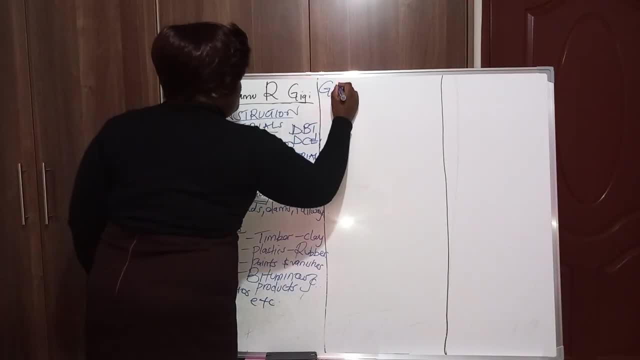 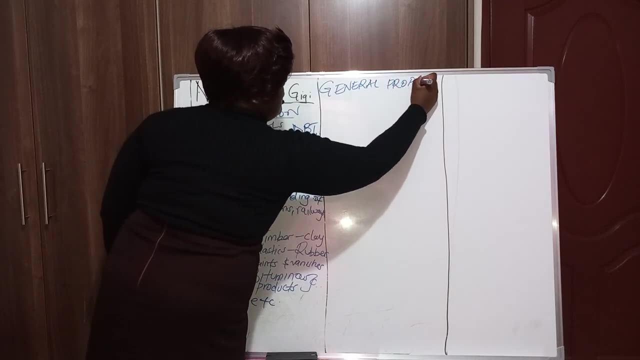 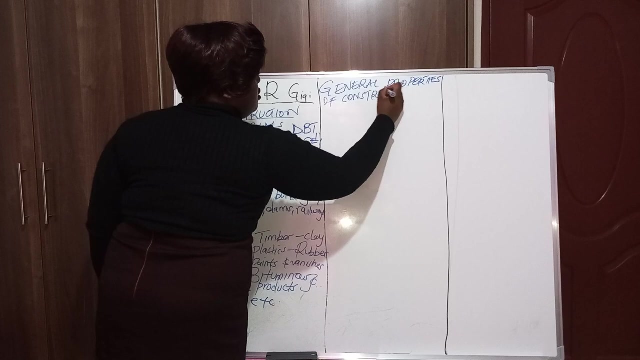 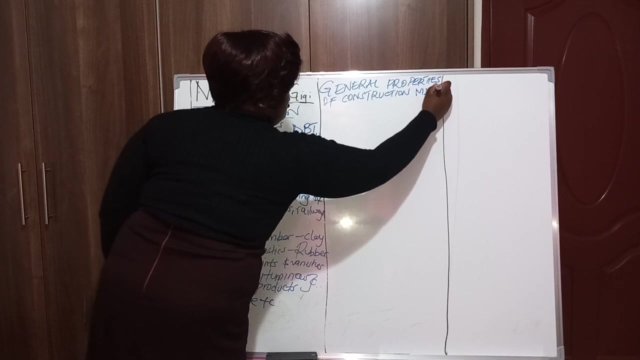 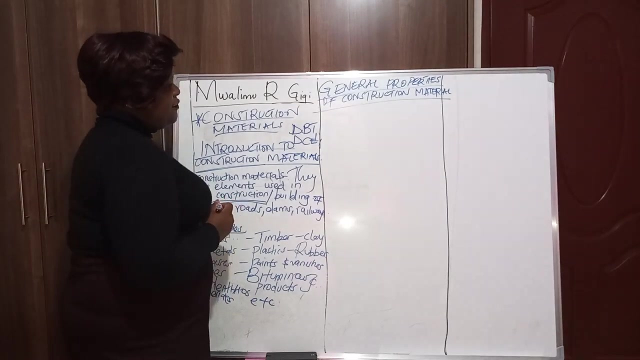 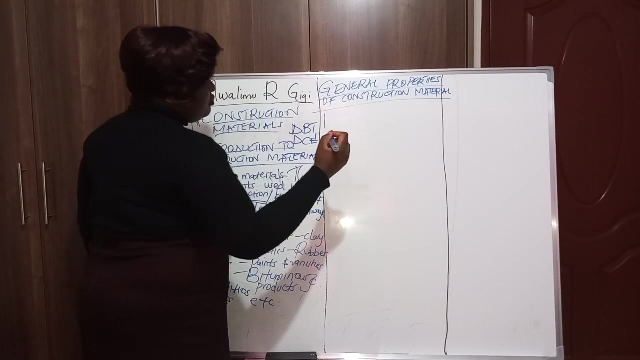 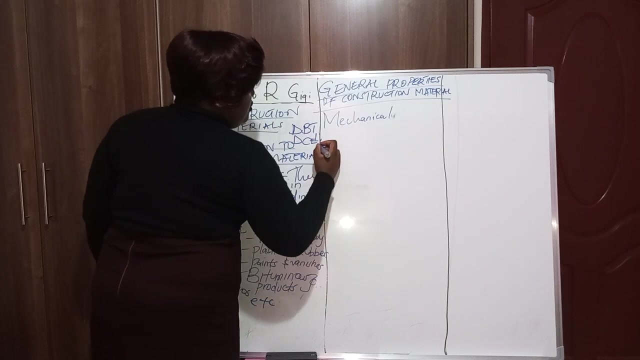 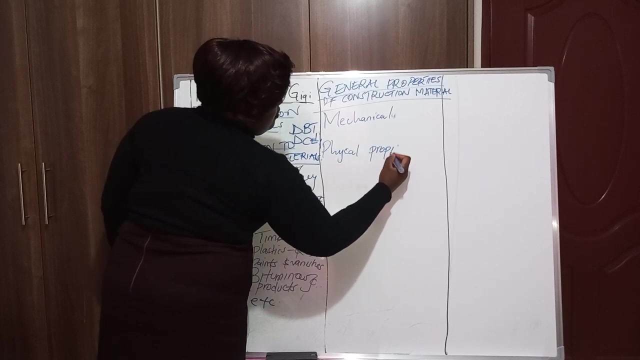 So the next one: we have subtopic. let us see the general general properties properties and the general properties of construction material, general properties of construction material. so we have two uh, two classification. we have, uh, we have mechanical properties, we have mechanical properties and we also have physical, physical properties proper. 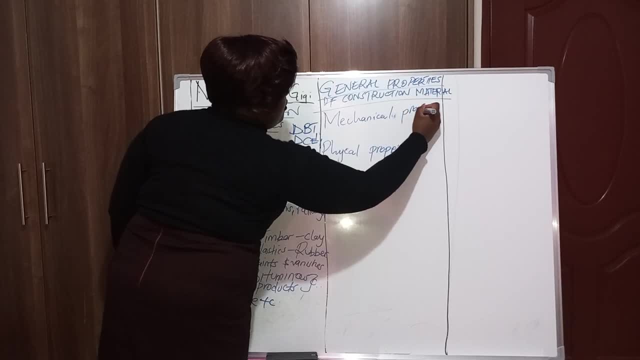 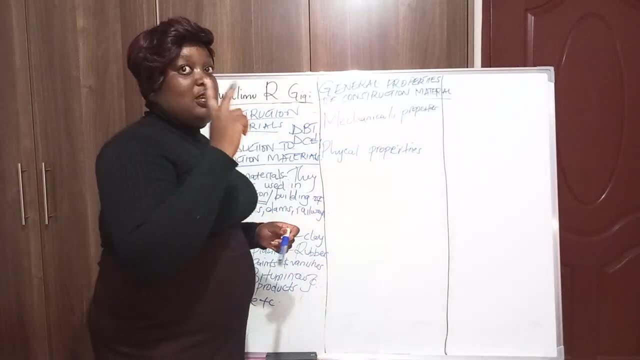 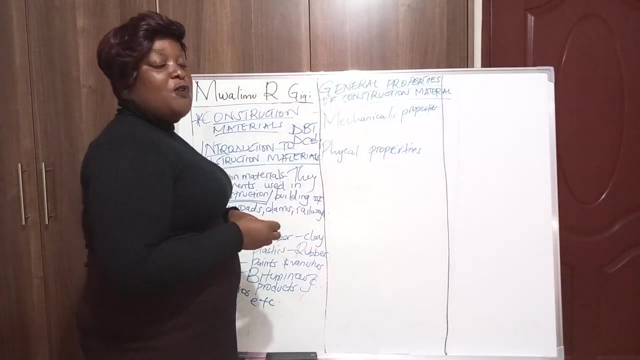 it is, and mechanical properties. so just to explain something, so, uh, properties of material, they are classified into two major groups: we have mechanical properties and we have physical properties. so for mechanical properties, they're just, uh, the action, or we can say the behavior of construction material under the influence of external forces. 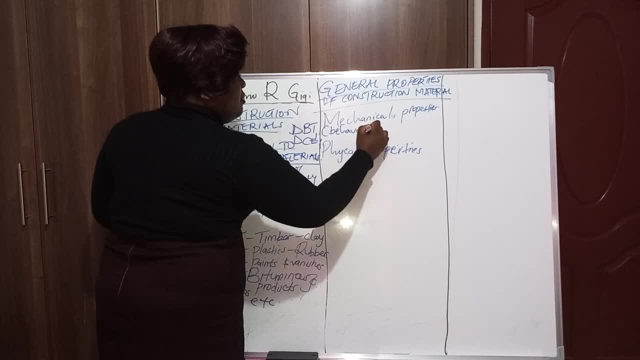 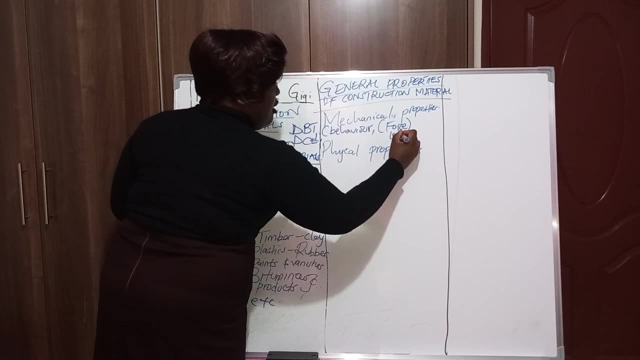 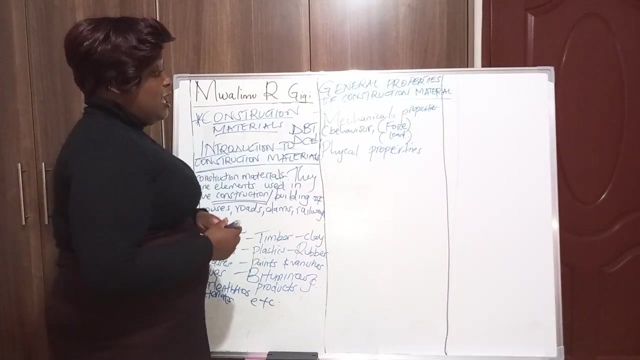 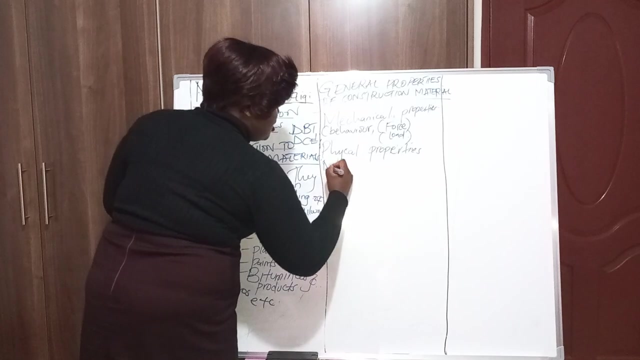 this is the behavior, behavior of construction materials under the influence of external forces, or we can say lord. so this we can see: the behavior of construction material under the influence of forces. and then physical properties. they are just properties of material that can be measured. so these are measurable, measurable properties. 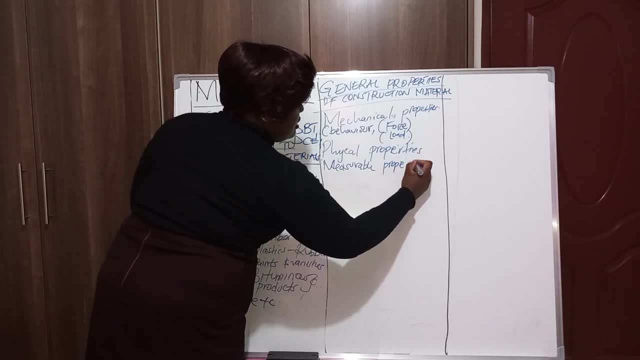 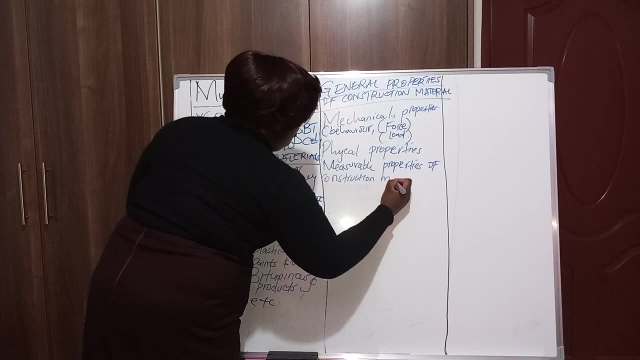 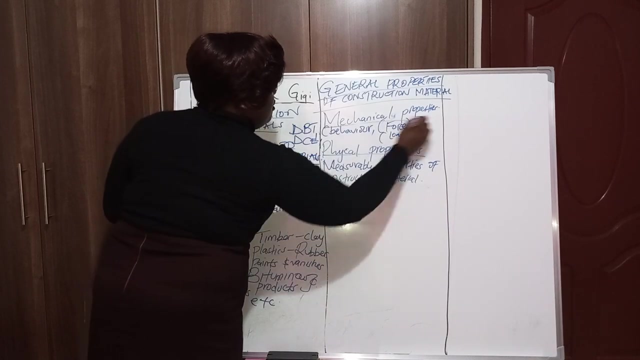 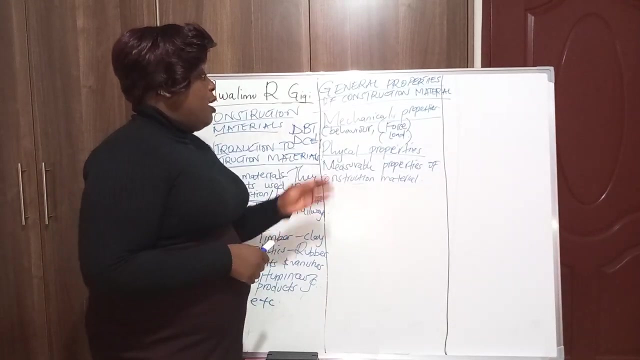 Xing-Fu made on earth. physical properties, they are properties of materials that can be measured. when mechanical properties, they add the behavior of a material act. almost yes, use these match more easily. material can be measured withstroming techniques, for example, shrimp factory in Fred Ahmet school of agriculture. these, uh, these um properties of construction material employment. 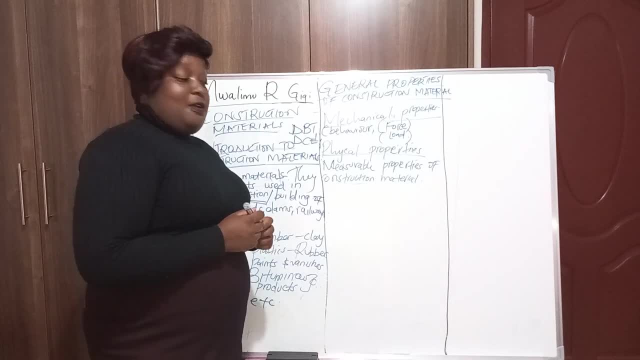 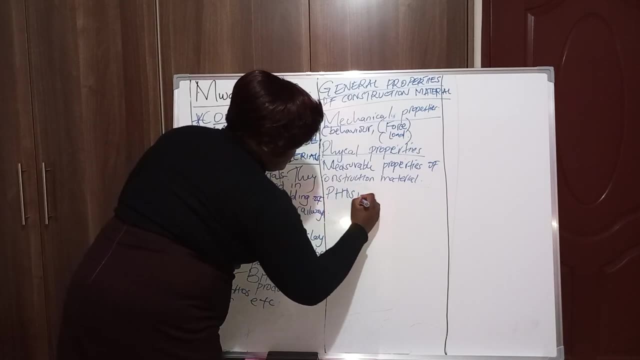 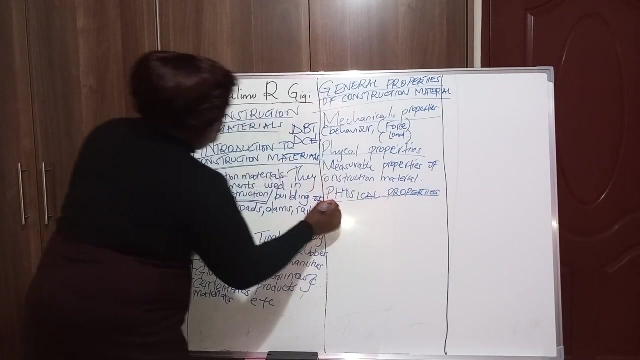 actions. so soon, physical physical properties. there are properties of construction materials that can be mentioned when mechanical properties. they are the behavior of a material act, the influence of external forces. so we can start with the physical physical properties, physical properties. so the first physical property we are going to. 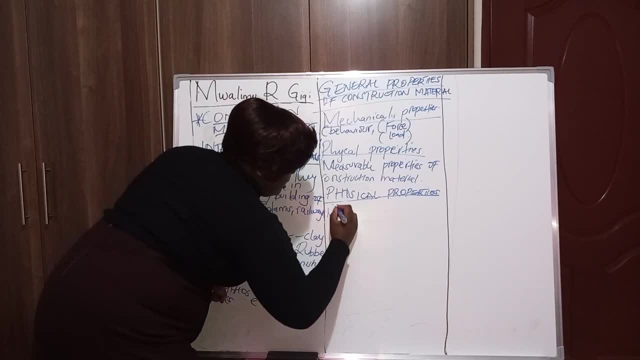 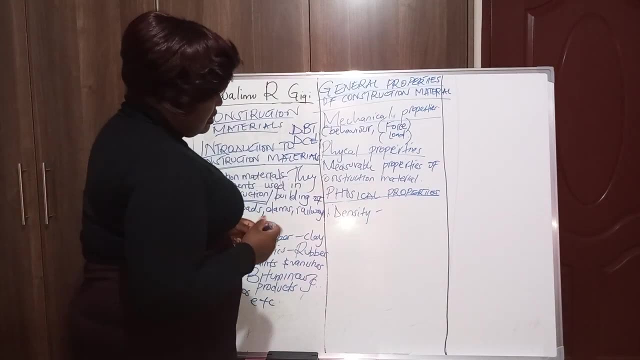 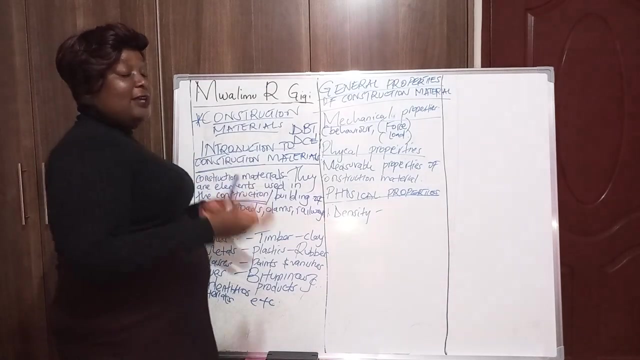 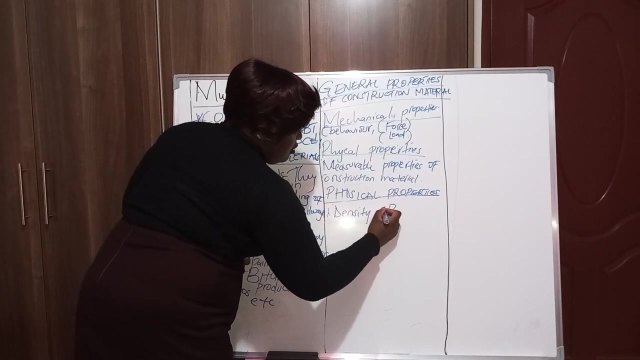 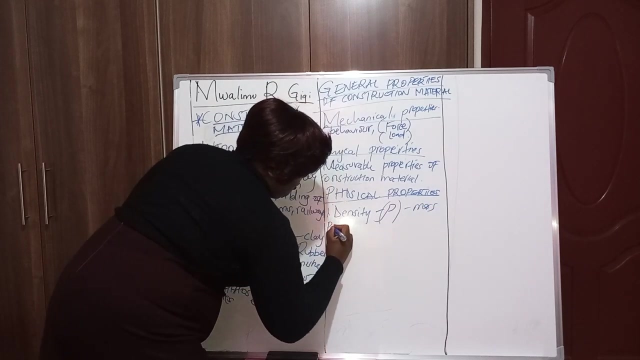 look at is density density. so density, density, as the first physical property of construction material. so as we have we learned in your high school, density is wrong, you know wrong, so we can. we can say that density is mass per unit volume of a construction material. so I know everybody is familiar. 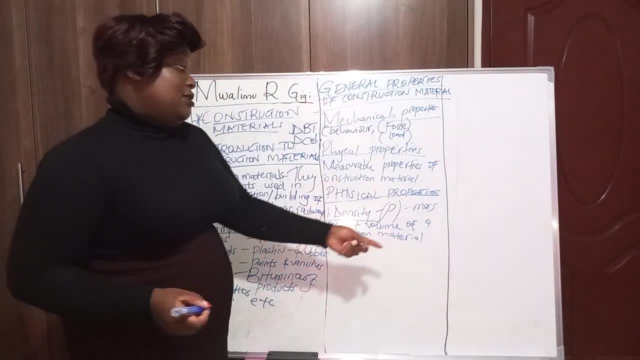 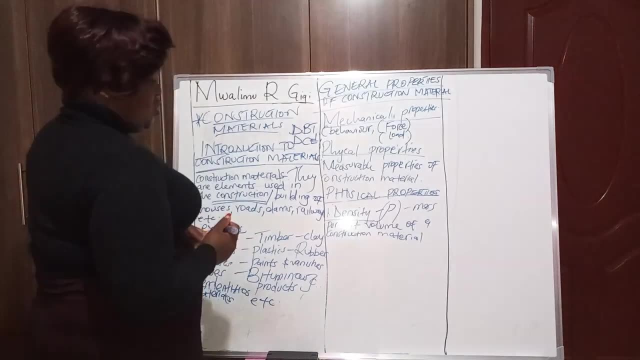 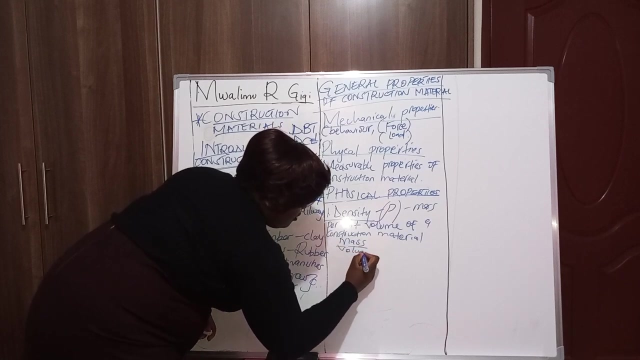 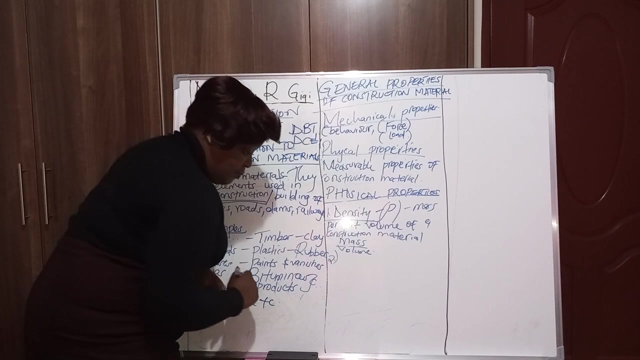 with with this, because it's something that we have learned. you know, density is mass per unit volume of a construction material, so it is mass per unit volume of a construction material. so it is mass per unit volume of a construction material. so another property, another physical property is: 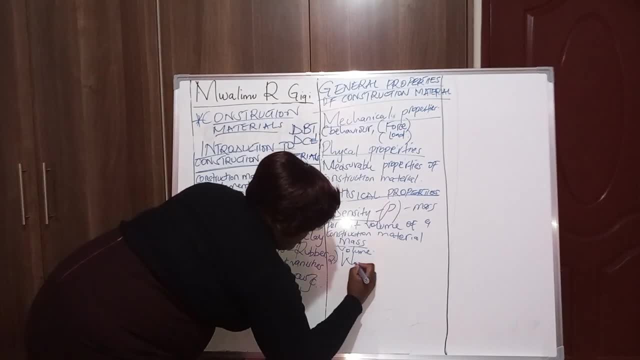 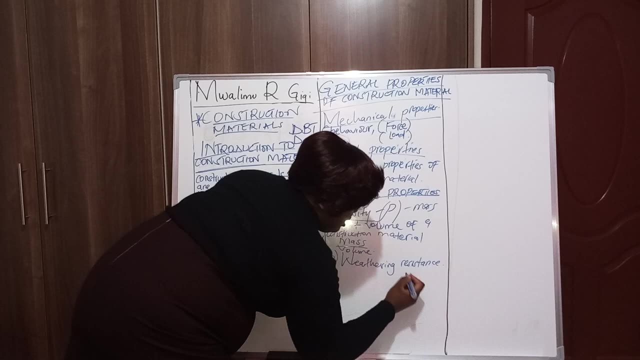 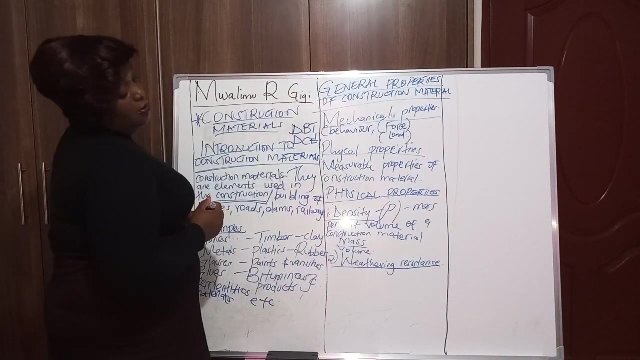 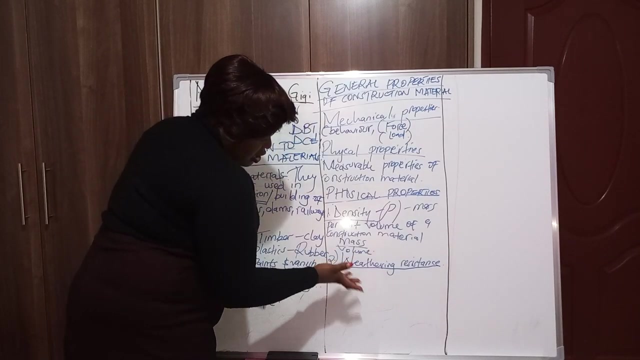 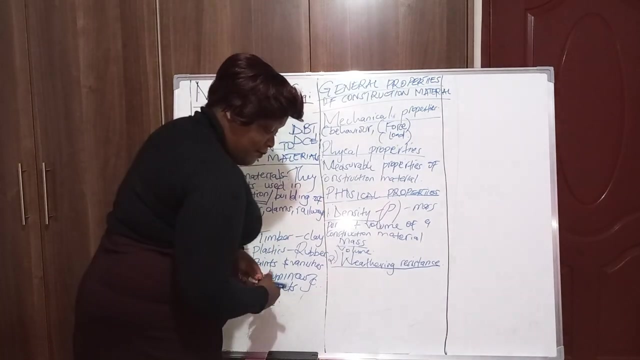 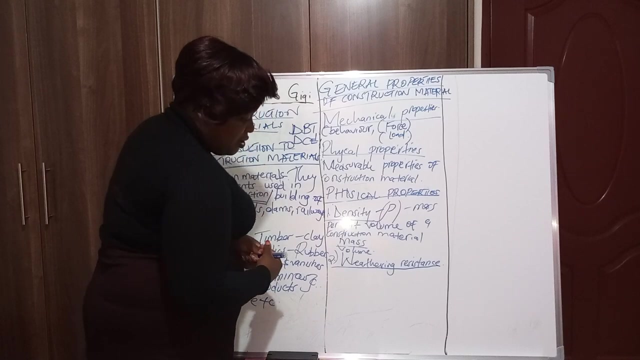 weathering resistance or weathering resistance. weathering resistance, weathering resistance, the second property, of course, of the second physical property of construction material. so weathering resistance, or well, weathering resistance, is the ability, is the ability of materials to endure wet and dry condition for a long period of time without deformation. so the ability. 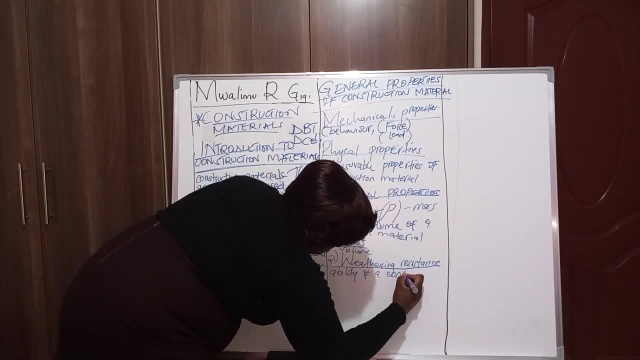 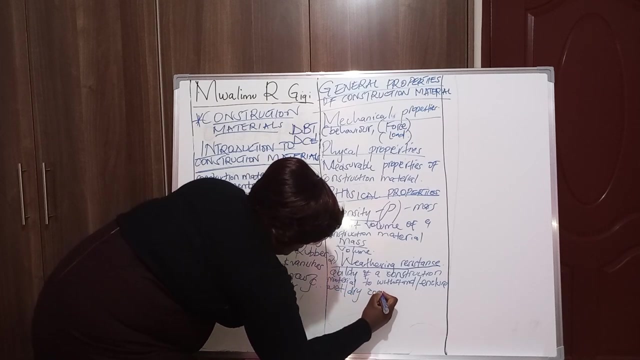 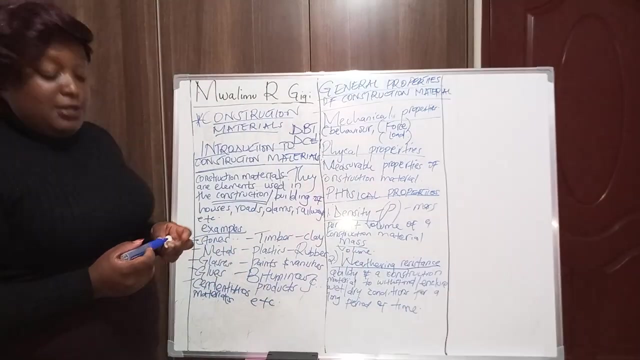 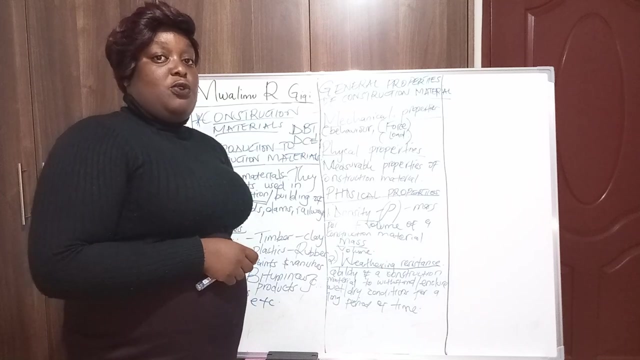 the ability of a construction material to withstand, to withstand or to endure a wet or dry conditions, conditions, conditions for a long, for a long period of time. so withering resistance is the ability of a construction material to endure with a wet or dry condition for a long period of time. 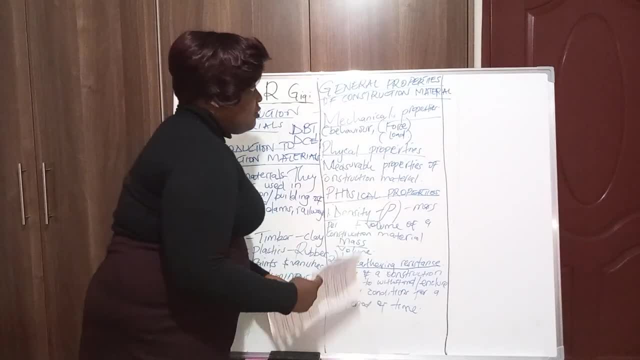 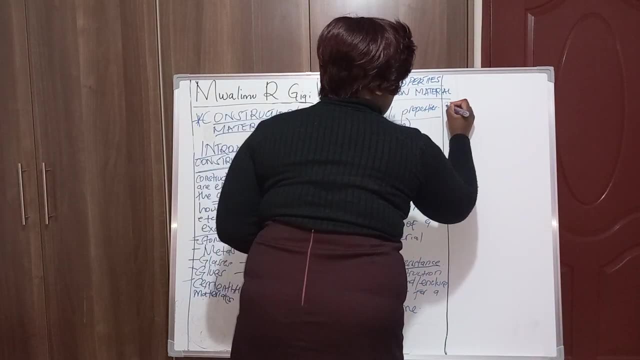 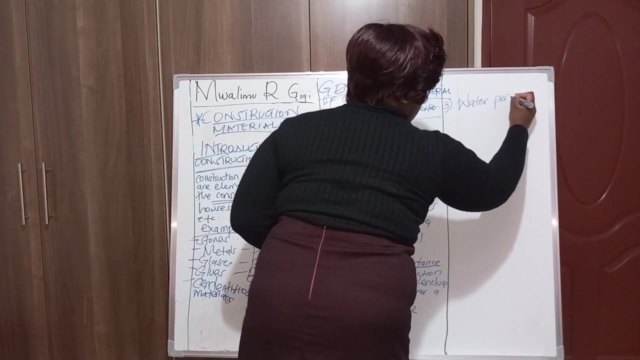 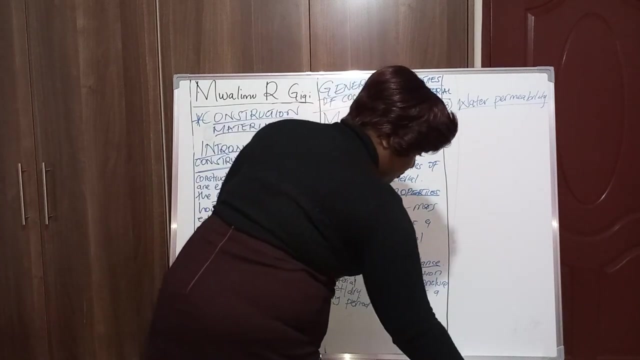 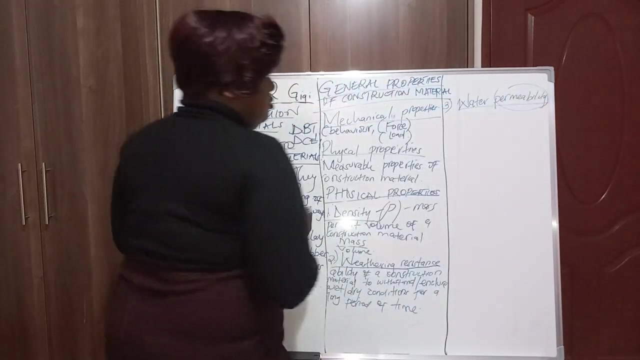 you can continue. i hope you are writing notes or i hope you are running something. so, number three: we can say: we can say water, water permeability, water permeability, water permeability, uh-huh as uh for permeability, permeable is uh to allow water to penetrate. 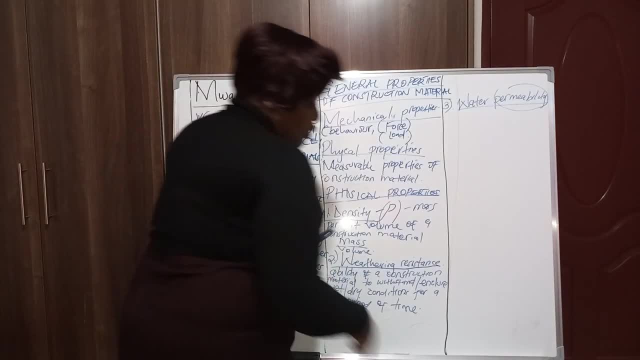 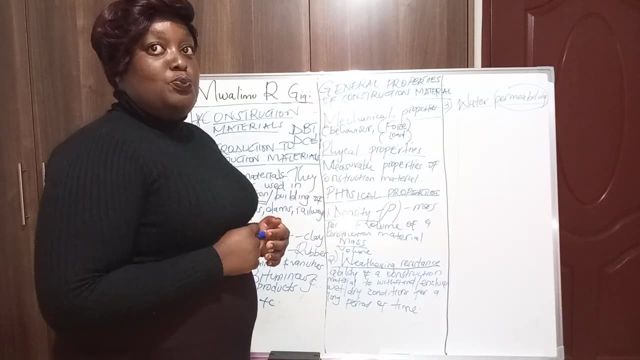 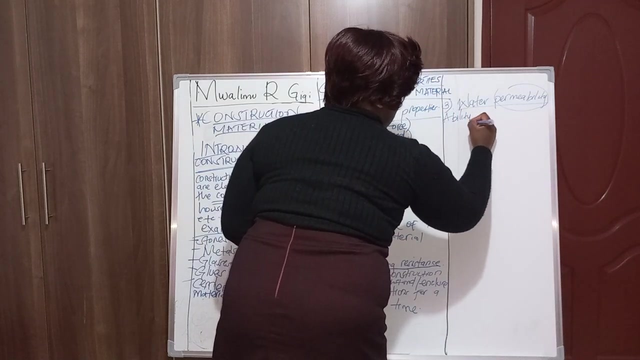 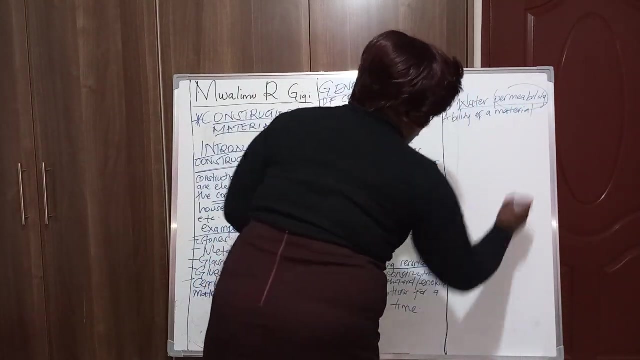 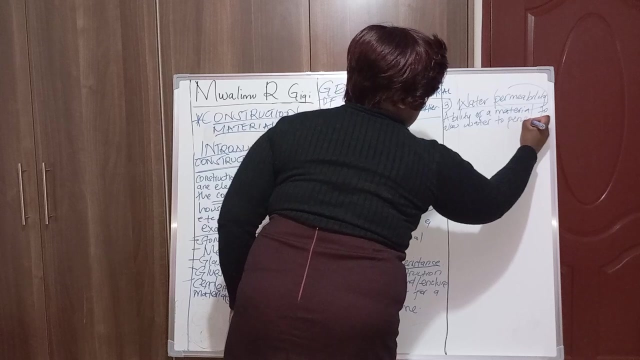 to penetrate a construction material. so our water permeability is the ability of a material, uh to allow water to penetrate under pressure. so it's the ability ability of a material. a construction material is the ability of a material to allow water to penetrate under pressure. so when you put pressure, when you, when you put pressure in a 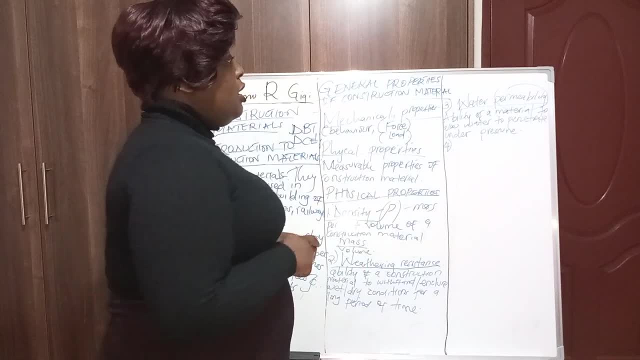 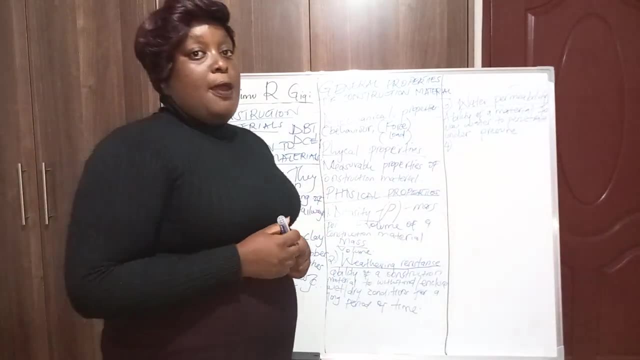 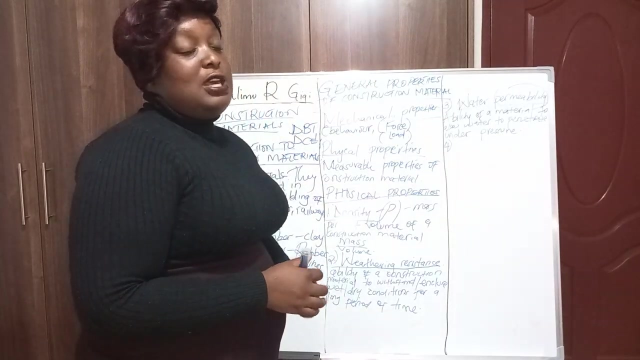 construction material, so the ability of it to be Sacrificed. pass method", Similar method to the essay to allow the water to penetrate. we can say that is water permeability property. so the next property is heat conductivity. heat conductivity is just the ability of a material to conduct heat, so heat. 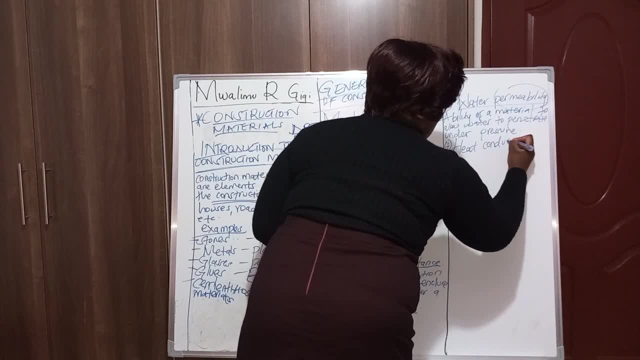 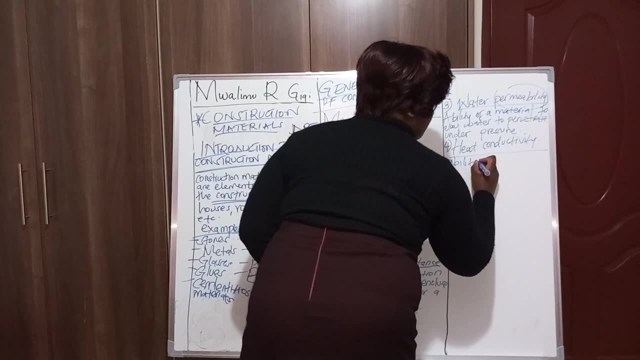 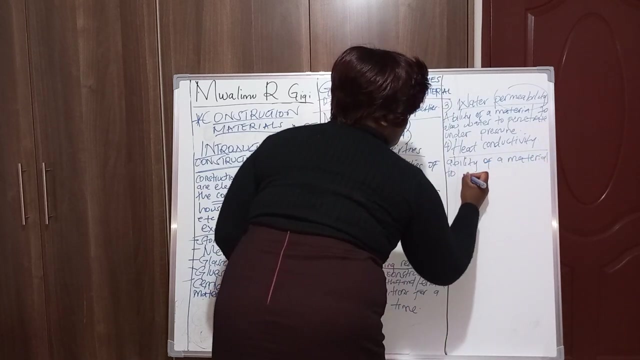 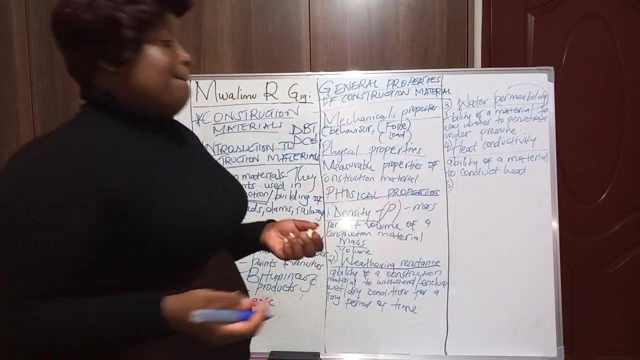 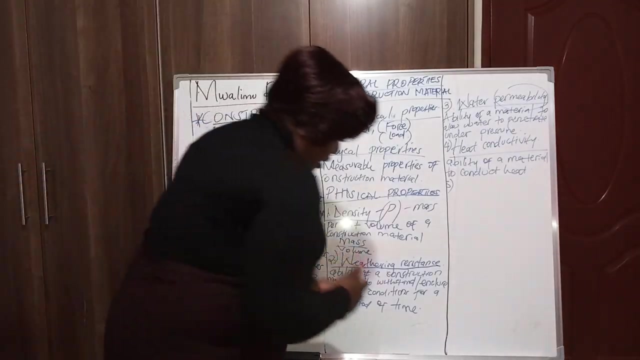 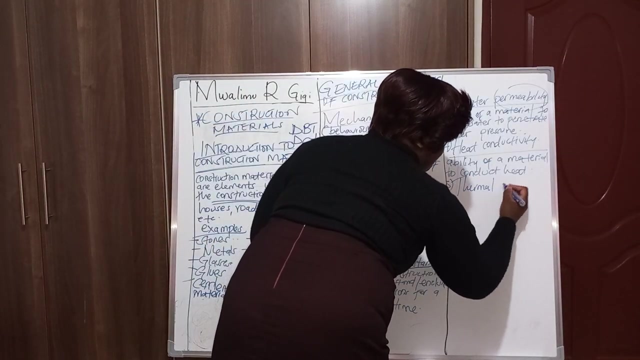 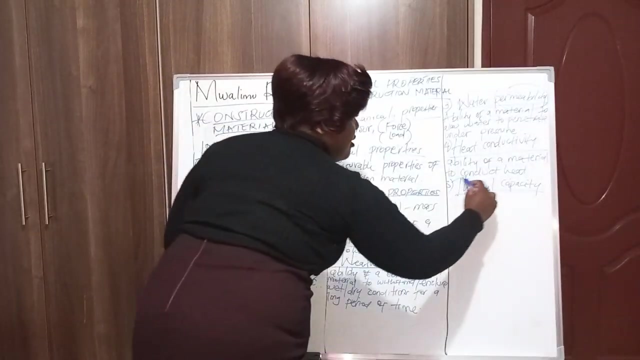 heat conductivity. heat conductivity is the ability of a material to conduct heat, the ability of a material to conduct heat, heat. number five: we can have a thermal capacity, thermal thermal capacity. thermal capacity, we are dealing with thermal, so it is. we also dealing with heat, so this is. 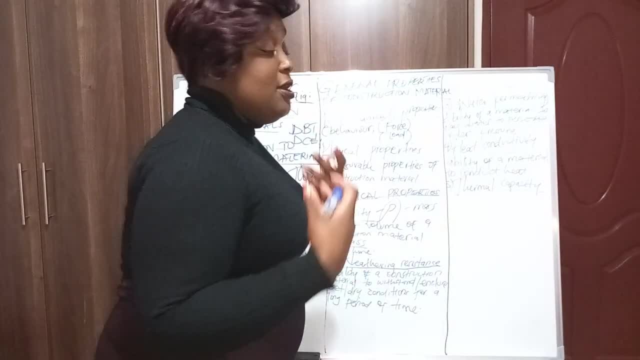 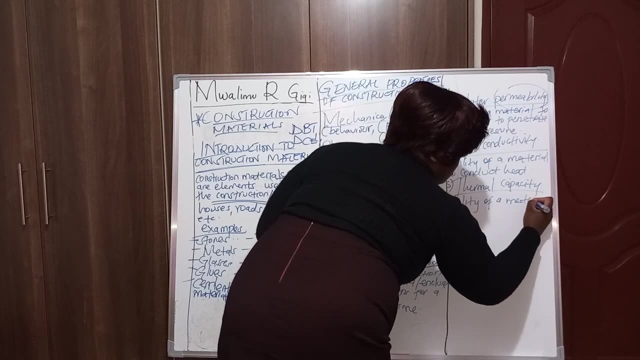 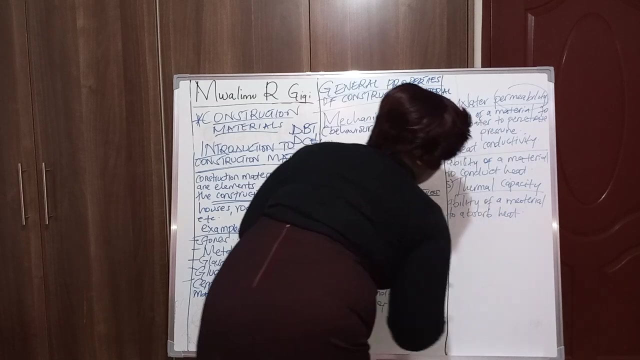 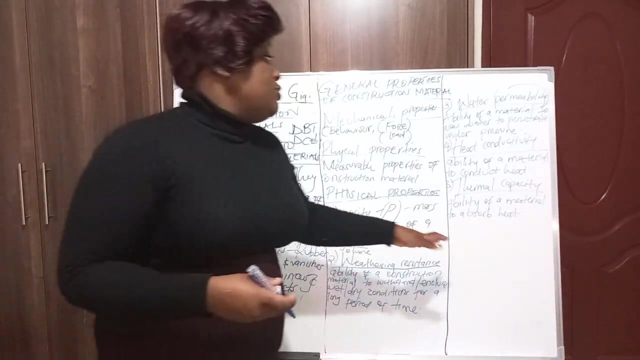 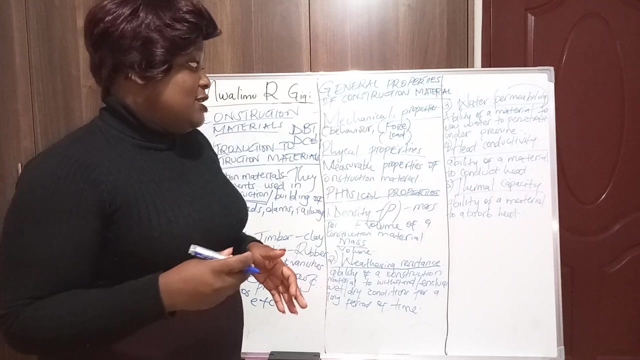 the ability of a material to absorb heat. so it's the ability of a material to absorb heat. so here we have heat conductivity, the ability of a material to conduct heat. and we also have a thermal capacity is the ability of a material to absorb heat. here we are dealing with construction. 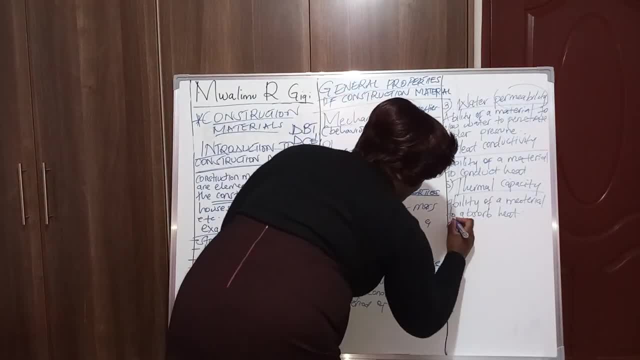 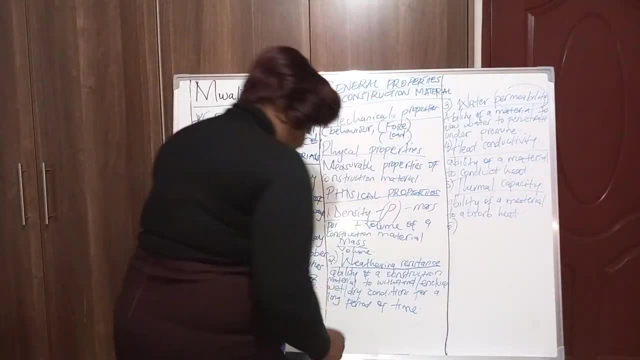 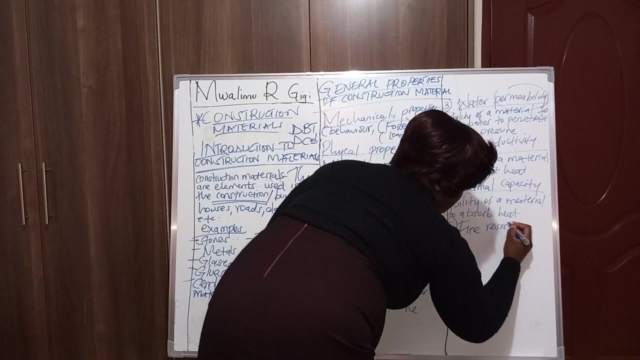 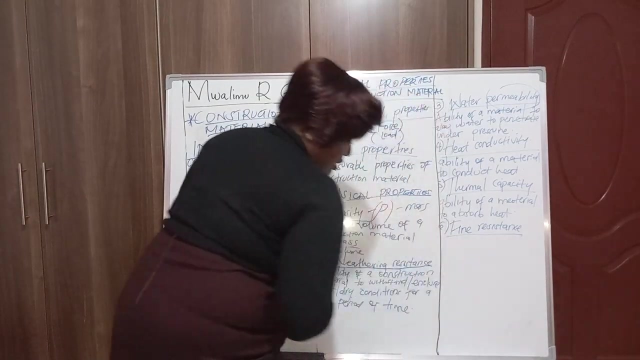 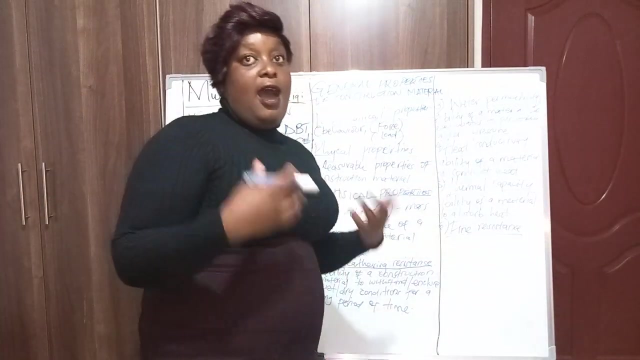 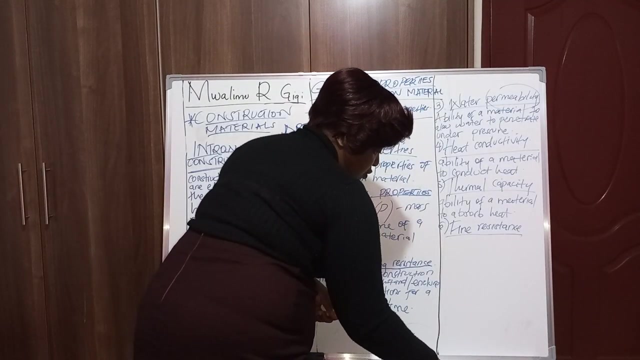 materials. number six, the sixth physical property of a construction material. we have fire resistance. we have fire resistance. fire resistance, we have four fire fire resistance. so for fire resistance is the ability of material to withstand high, high temperatures so we can strike, is the ability of materials to resist. 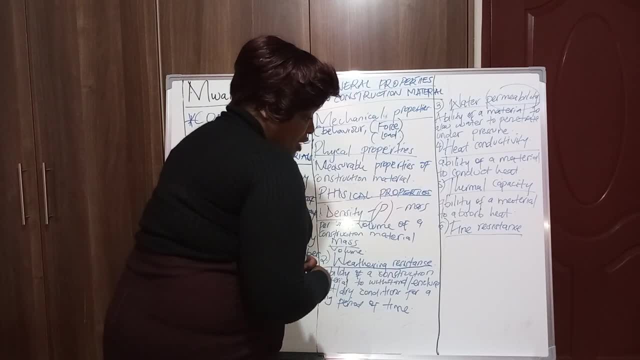 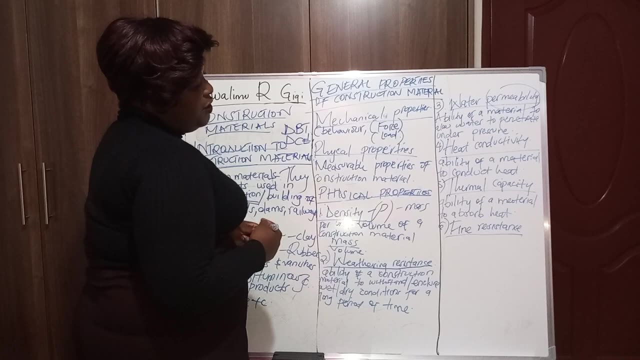 the action of high temperatures without deformation. there is a pleasant feel in voyezve��i on live on a fire-resistant. this is the ability of a material with high temperatures to withstand without deformation or substantial loss of strength. so we can, we can write the ability. 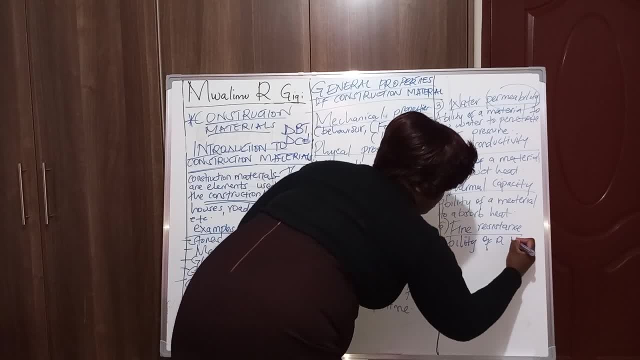 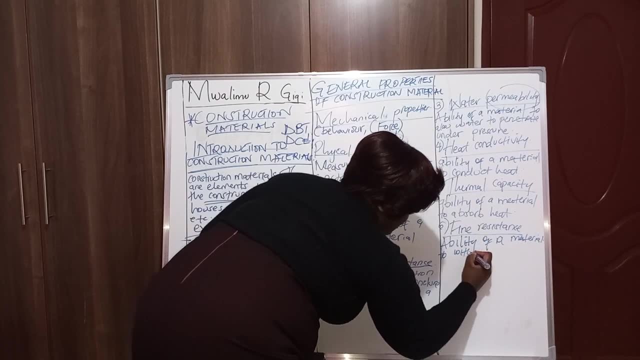 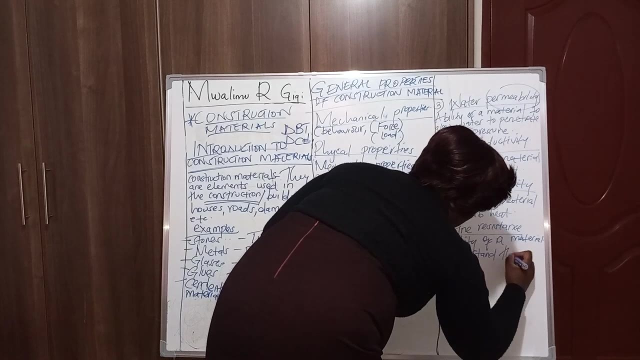 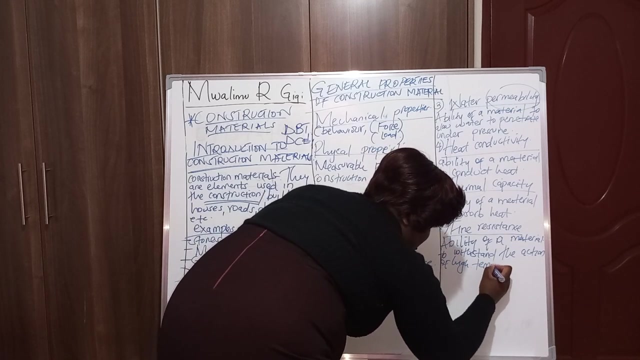 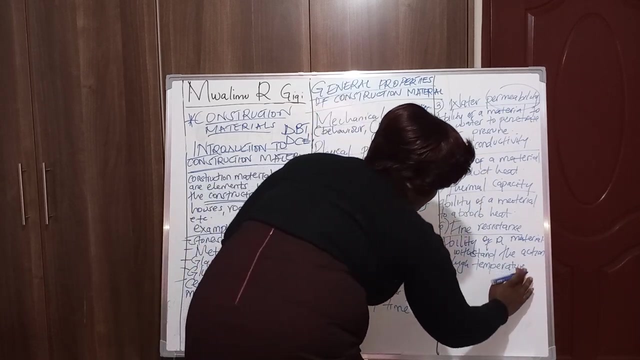 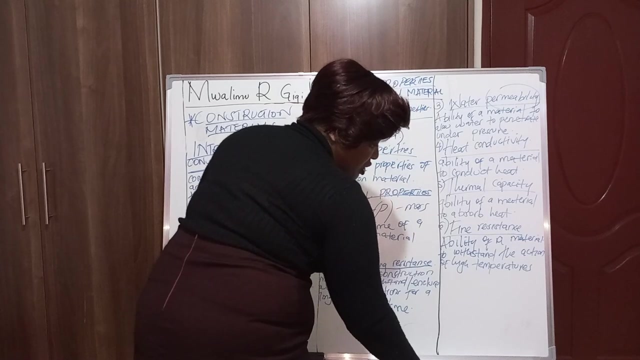 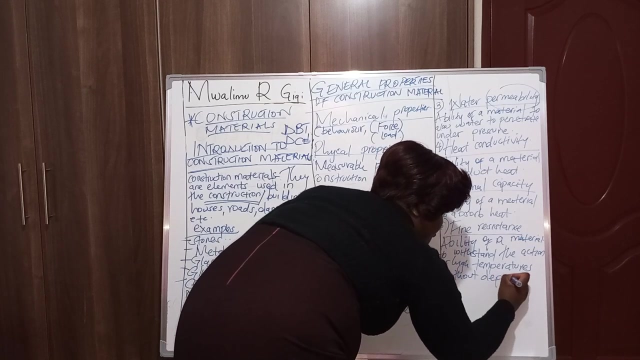 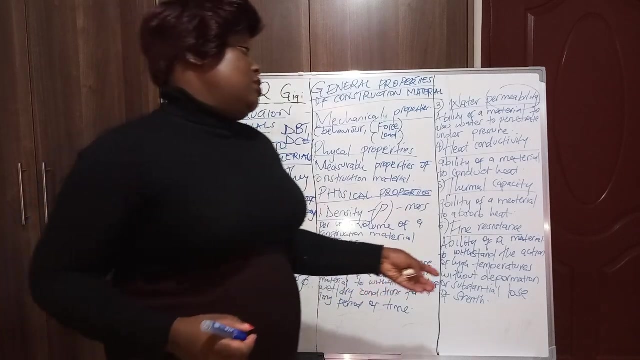 of a material is the ability of a material to withstand, to withstand high, to withstand the action, the action of high temperatures, temperatures, temperatures. we stand high at the action of high temperatures without, without deformation or substantial loss. loss is loss of strength, for example- I can give one example for fire: 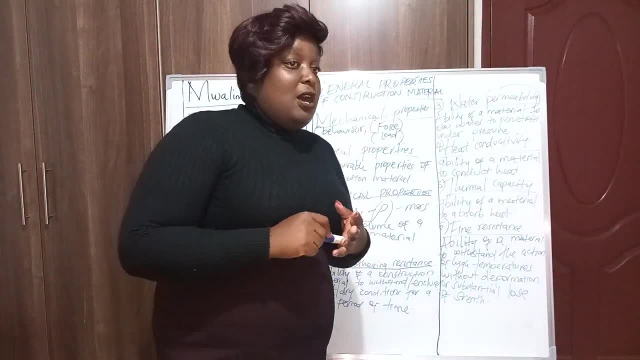 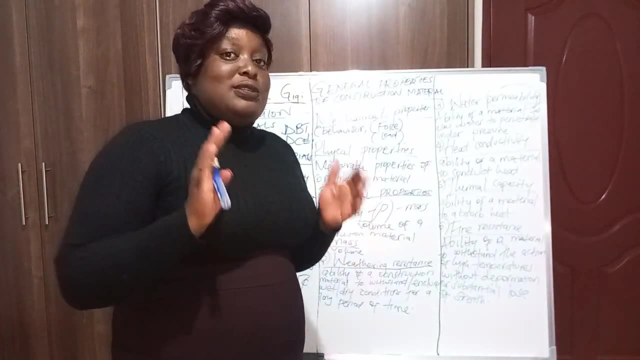 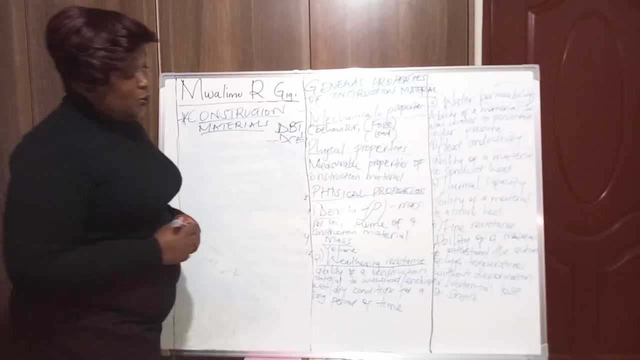 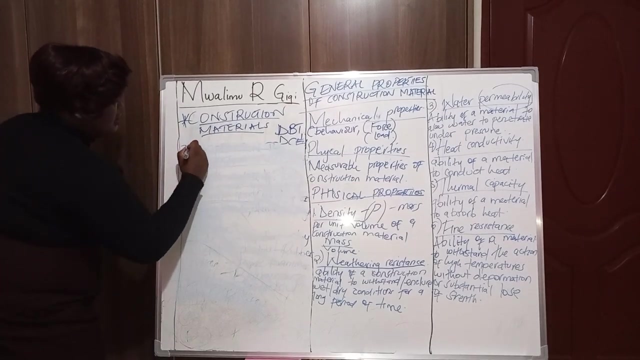 resistance is just for our bands, uh-huh. so when we are making our balls, we need to use a construction material that is able to withstand the action of high temperatures. uh-huh, so we can continue. so we were at a fire resistance, so we go to next. that one was number six, so number seven is chemical. 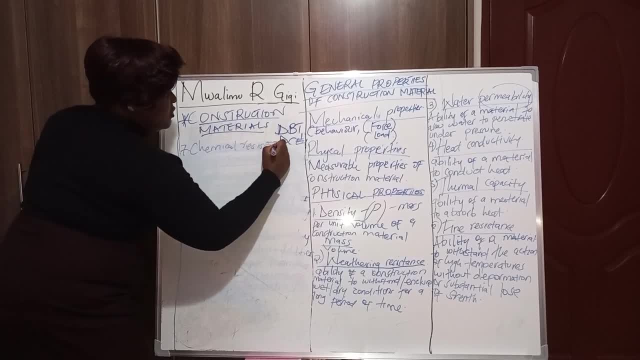 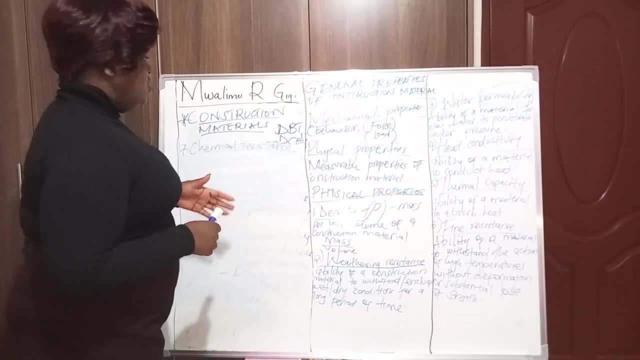 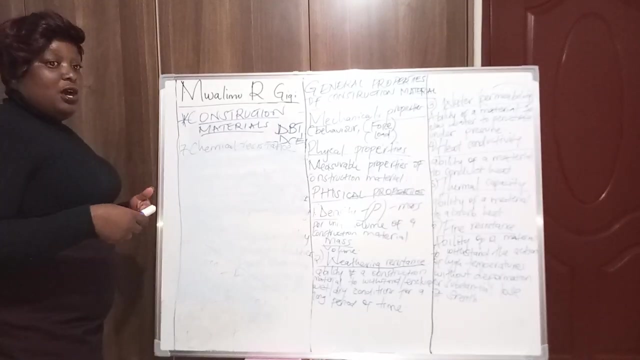 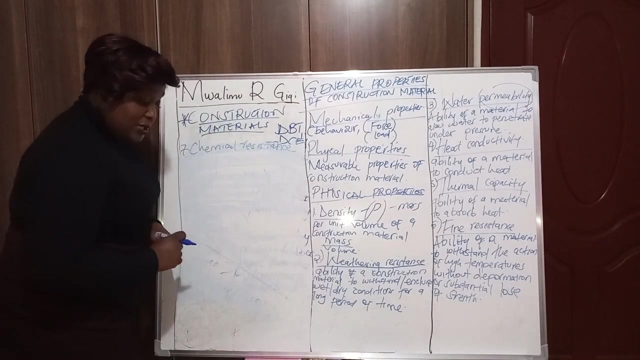 resistance, so resistance. so a construction material should be able to withstand the actions of chemicals like acids, bases, alkalines and uh, even uh sea water. so is the ability, the ability of a material to withstand the action of uh, the ability of a material, uh to withstand, withstand the action. 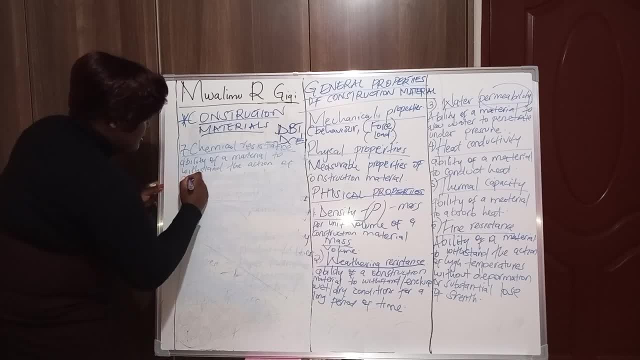 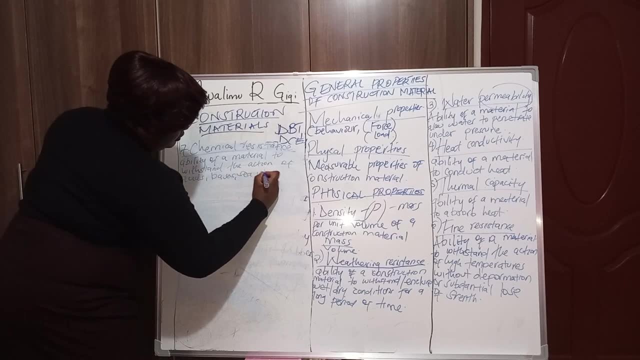 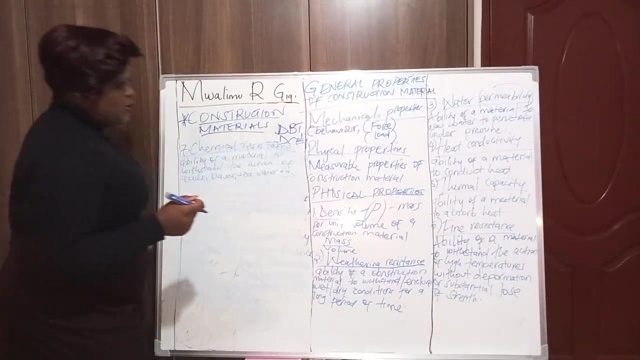 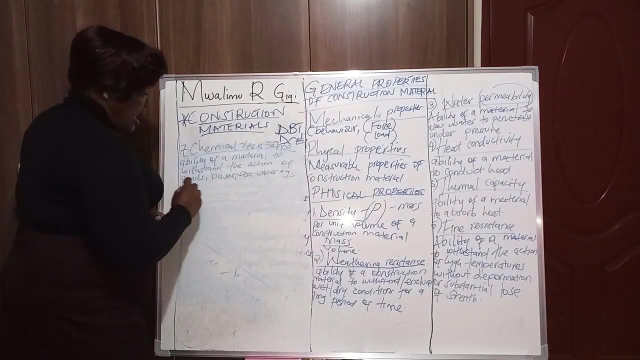 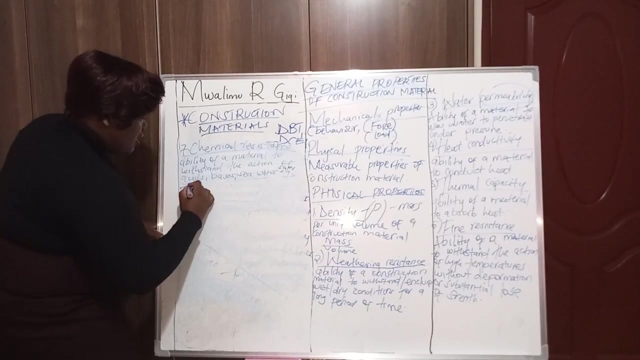 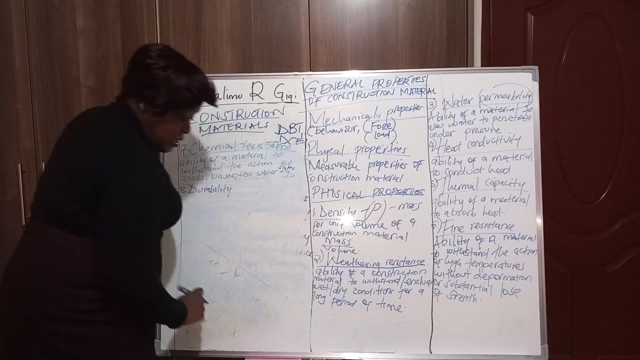 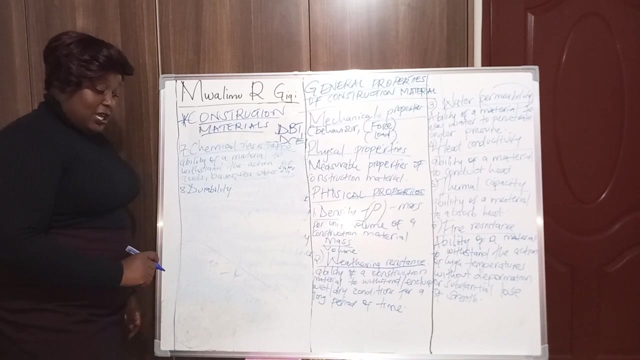 the action of acids, bases, uh uh, sea water, etc. we have the chemicals that, uh, they destroyed construction material. so a construction material should have the ability to withstand, uh, the action of of acids, bases, salts, sea water, even salt. So the last one we have durability, Durability. So durability is the ability of a material to resist combined effect of atmospheric and other factors. 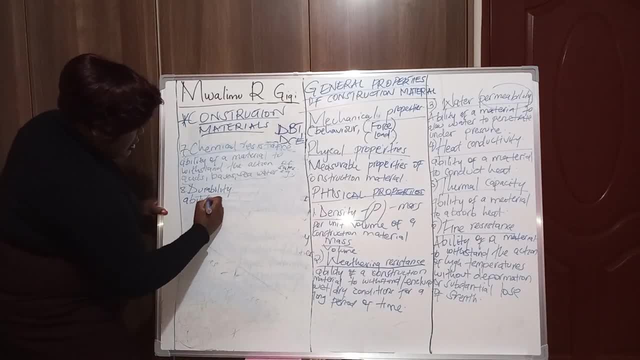 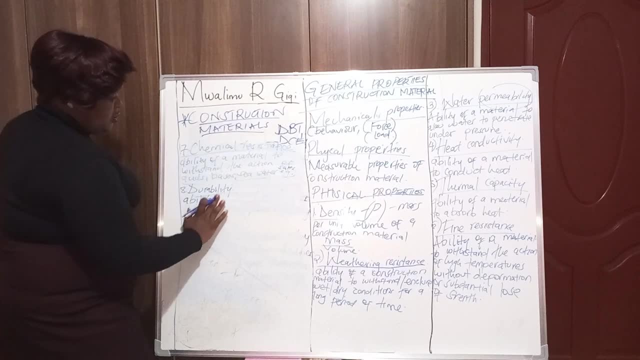 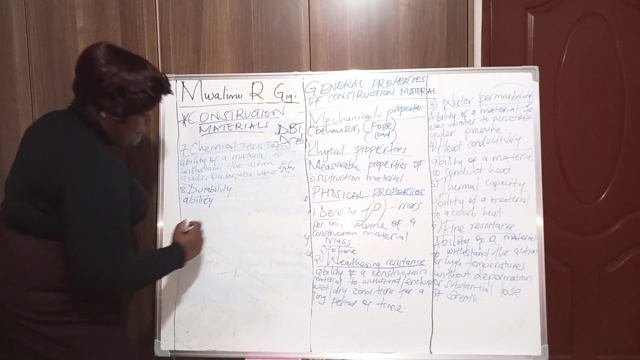 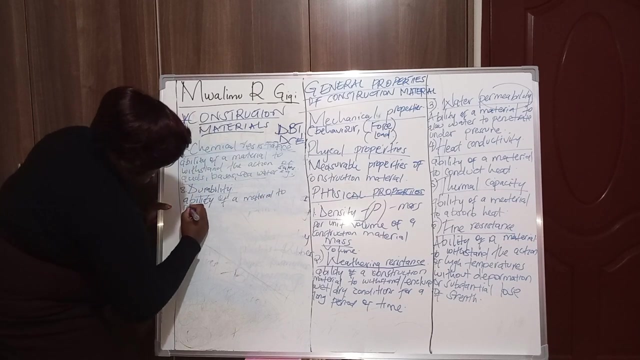 So the ability, So somebody can say the ability of a material to last longer. I think that's also correct. You can comment down on the comment section. The ability of a material to resist the combined effect of atmospheric and other factors. The ability of a material to resist the combined effect of atmospheric and other factors. 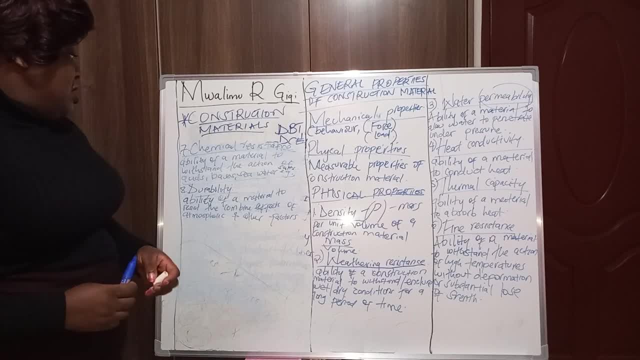 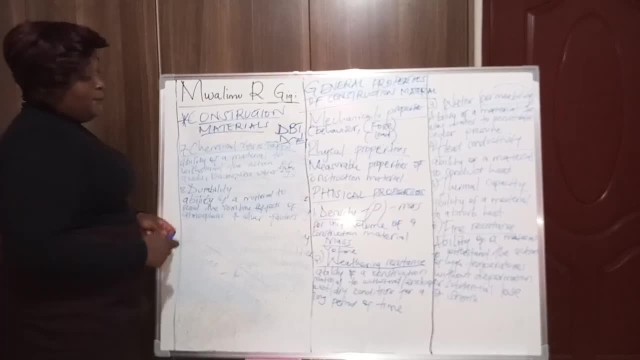 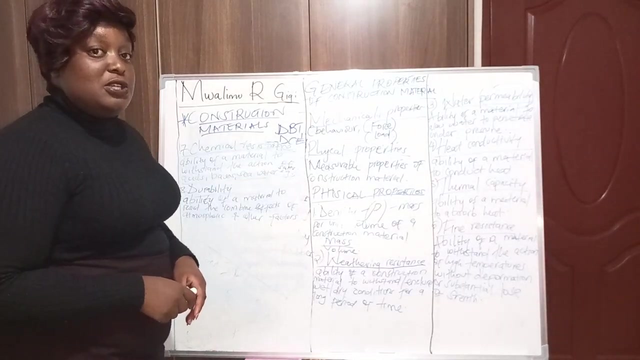 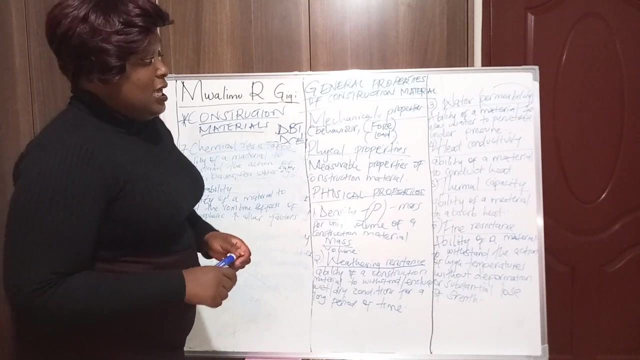 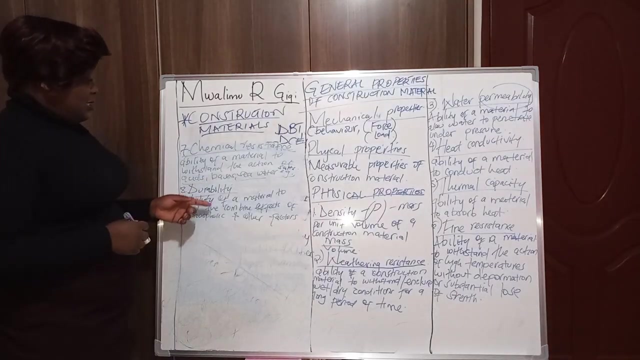 So the ability of a material to resist the combined effect of atmospheric and other factors is durability. So those eight properties, they are physical, Physical properties of construction materials. So we have density, We have weathering resistance, We have water permeability, heat conductivity, thermal capacity, fire resistance, chemical resistance and durability. 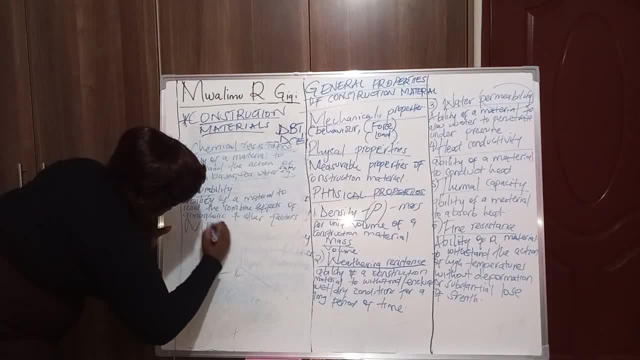 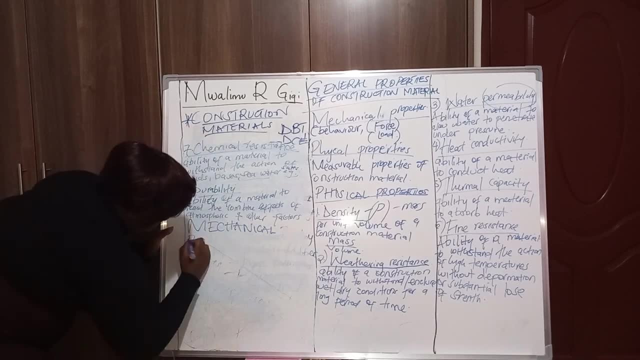 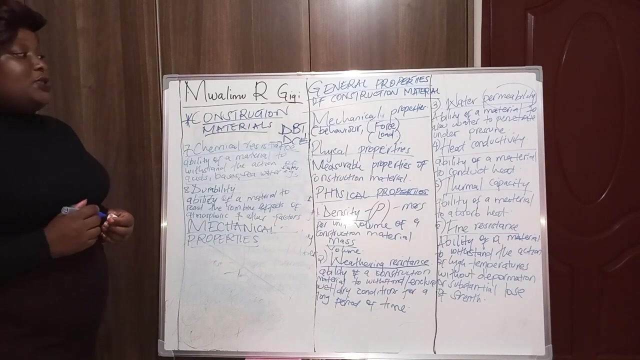 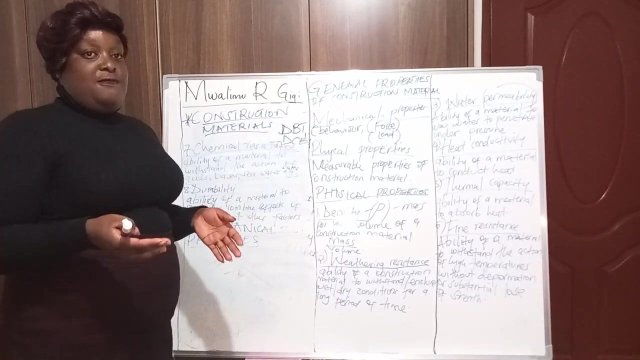 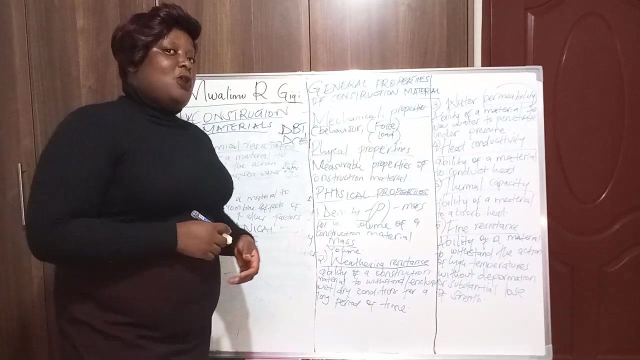 So we go to next mechanical Mechanical properties. So mechanical properties of construction materials. We have said here that the mechanical properties are just the behavior of the construction materials under the influence of force or under the influence of load. So we have: the first one is strength. 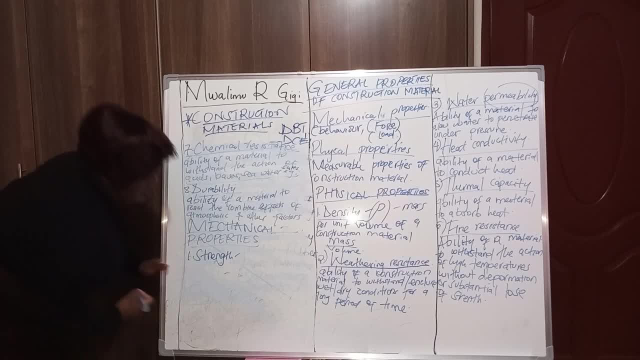 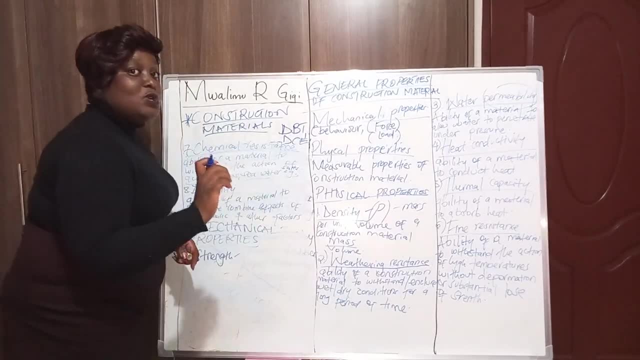 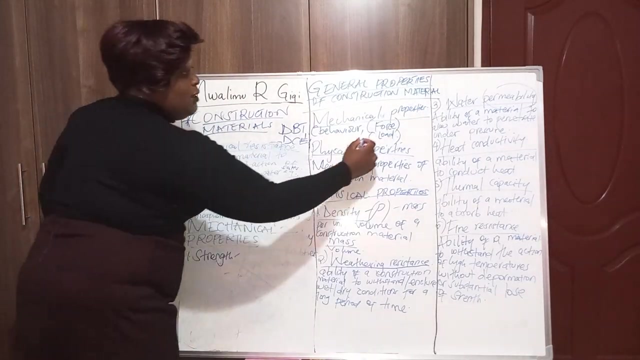 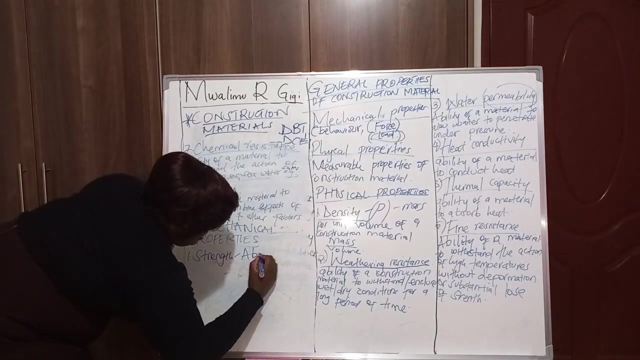 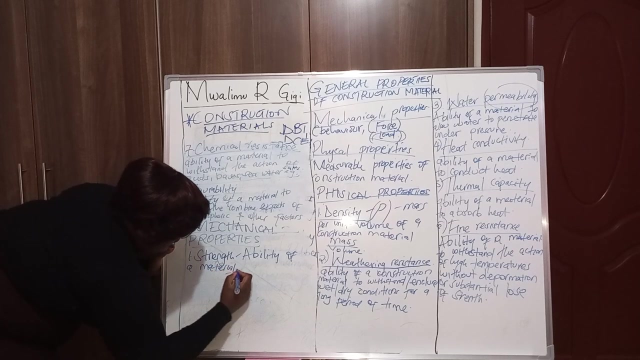 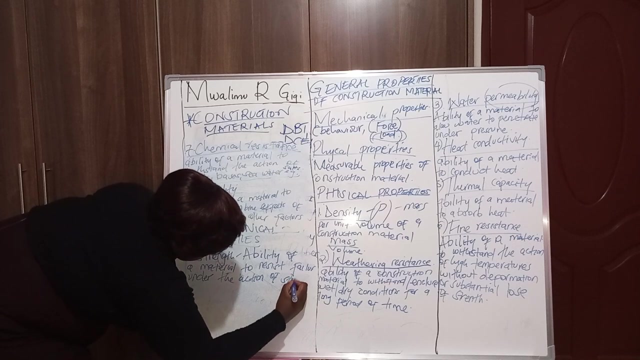 Strength, So strength is the ability of a material to resist failure. The ability of a material to resist failure under the action of stresses caused by loads, Under the action of stresses caused by loads. So the ability of a material To resist failure Under the action of stresses caused by loads. 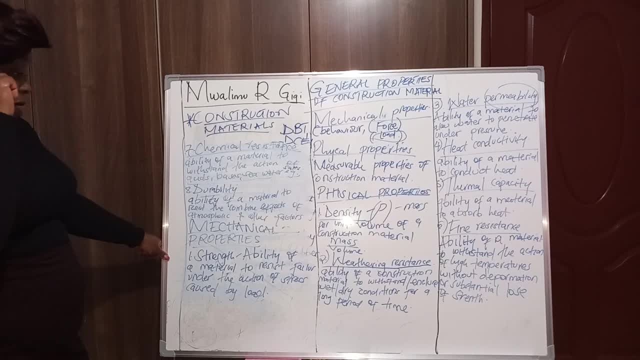 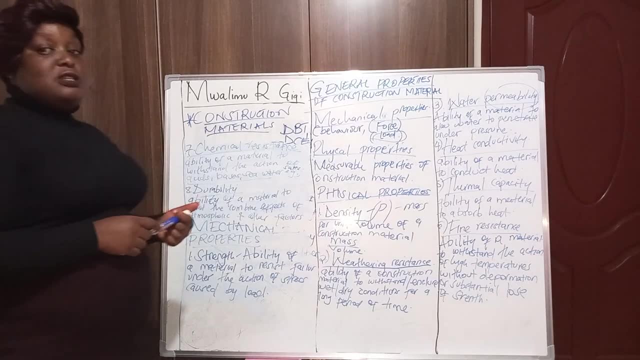 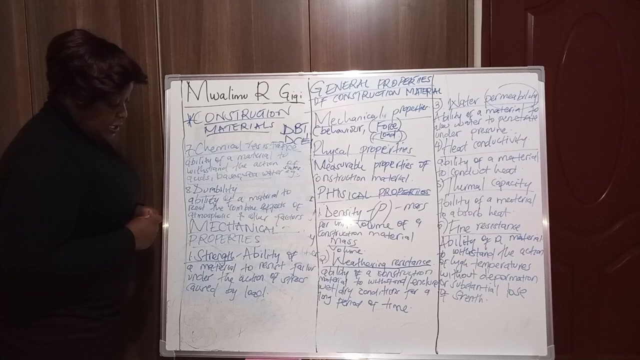 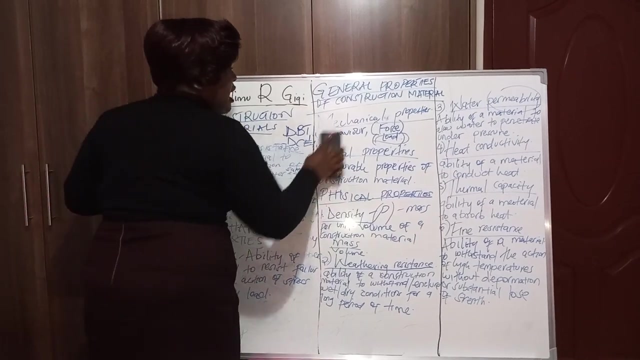 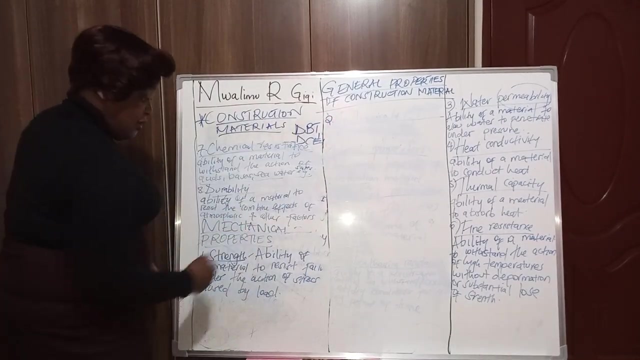 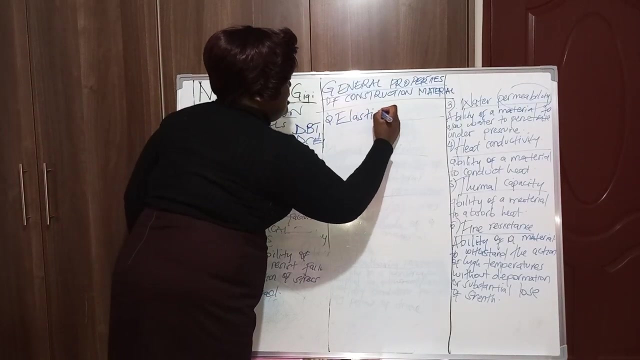 So the ability of a material to resist failure, To resist failure, failure under the action of stress caused by loads, that is strength. so the second one, second one- yes, we can drop this side. so the second one, the second mechanical property of a construction material: we have elasticity, elasticity. 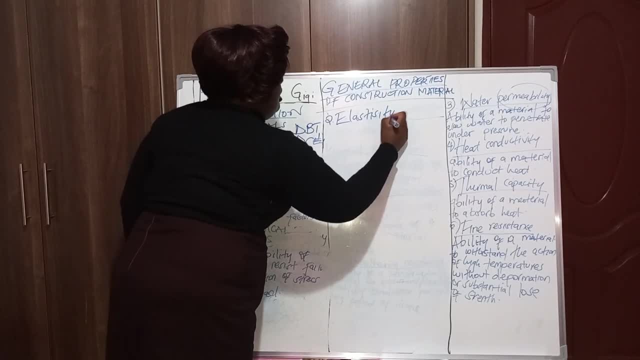 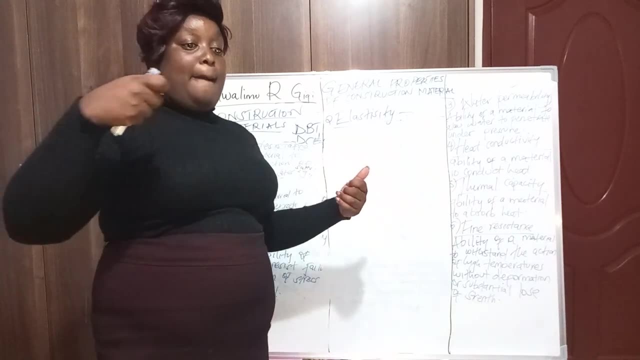 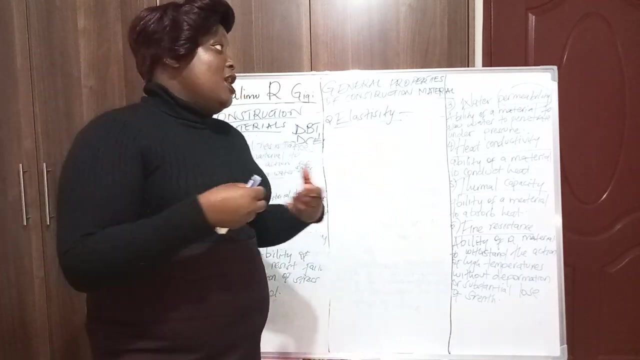 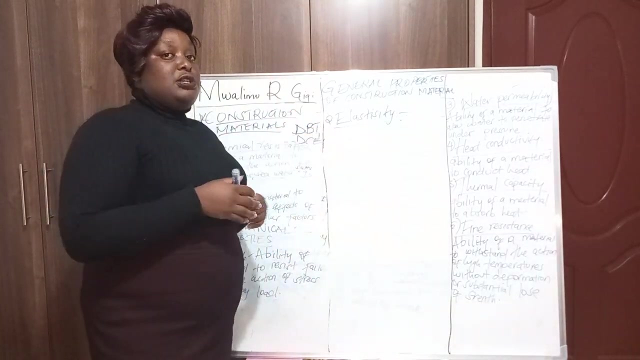 elasticity, ah, USB city, when you have a stream or a award, this neutral has a bladder rather, for example, a bladder give ruching, it stretches, and when you live here there will be resistance to a side bowl, ok, but the housing having a, it in a really back to its original shape or original size. so that is. 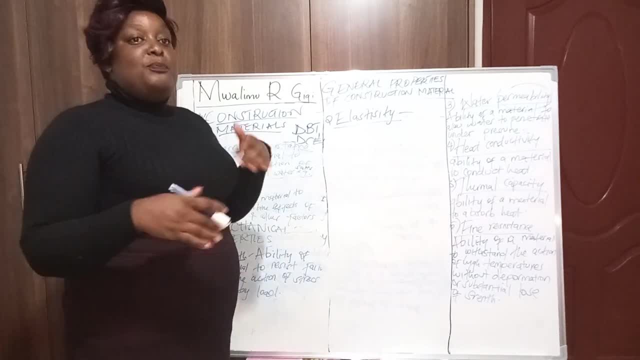 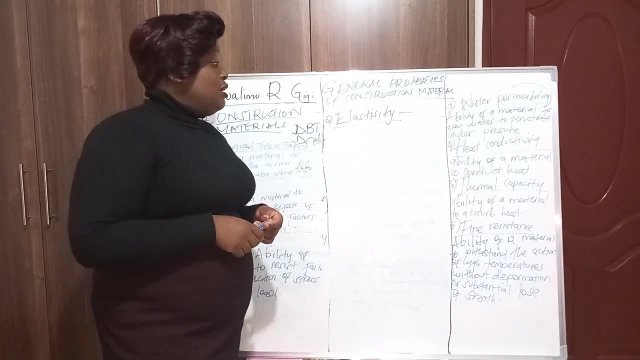 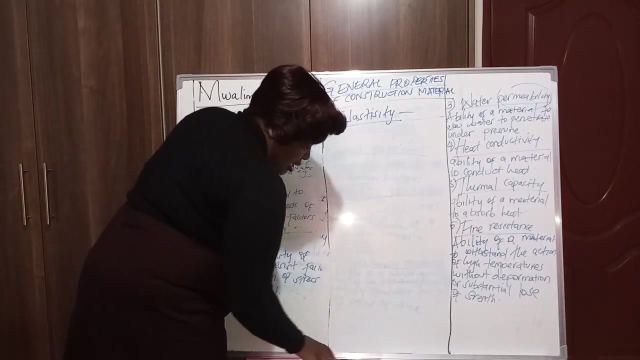 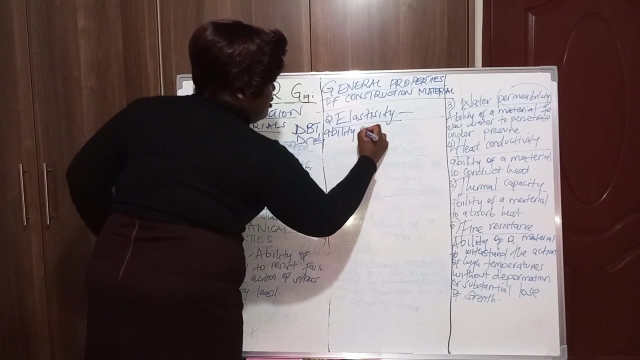 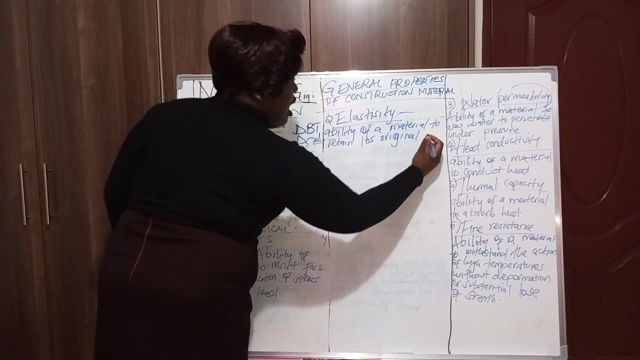 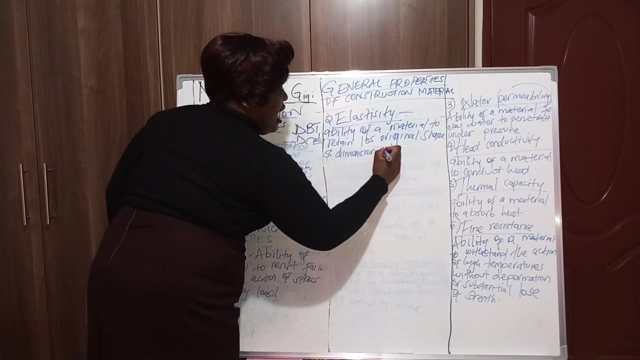 elasticity. so elasticity is just the ability of a material to regain or retain its original shape and dimension after the force causing the deformation is removed. so that is elasticity. elasticity, the ability of a material, ability of a material to retain its original, original, original shape and dimension after the force, after the force cozy, the deformation, and that the after the. 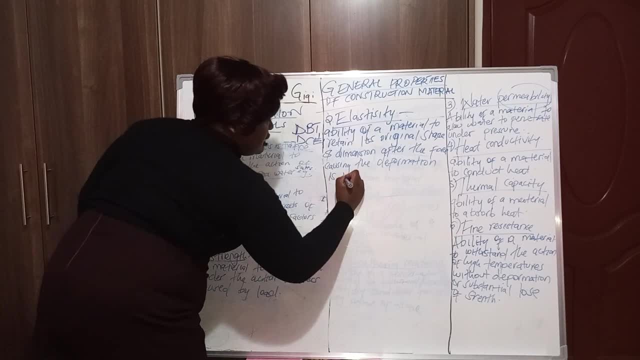 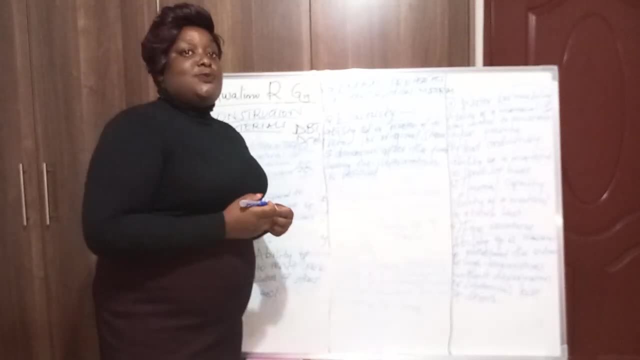 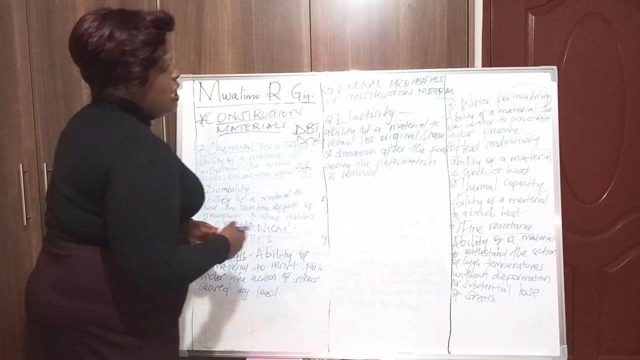 force causing the deformation is removed. I said, and a good example is I like a bladder or a stream. it's called a spring, a spring, a spring spring. So when you remove the external forces, it goes back to its original shape and dimension. So that is elasticity. 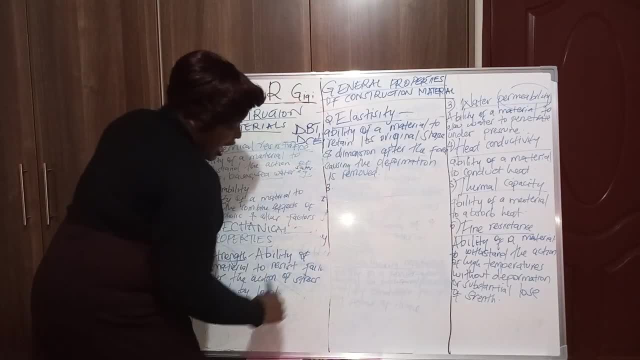 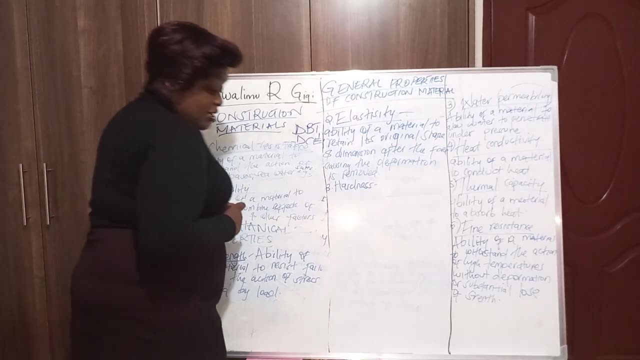 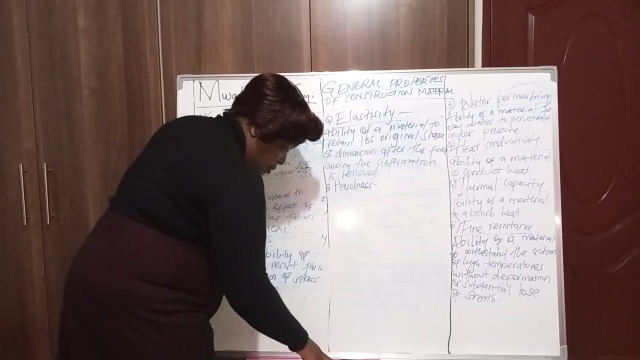 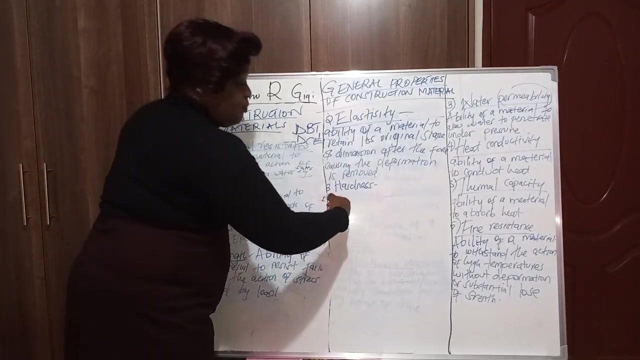 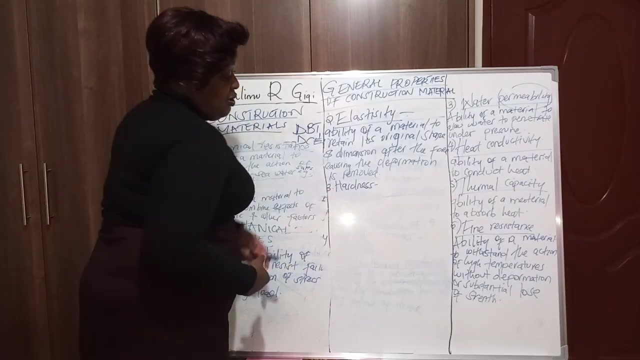 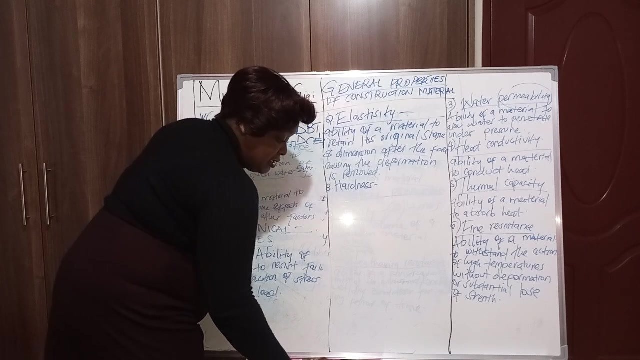 The third one we have hardness. Hardness is the ability of a material to resist penetration by a harder body, Like, for example, if I do this, this board I can say is hard because it is resistant Penetration of hard bodies. So it is the ability of a material to resist penetration by harder bodies. 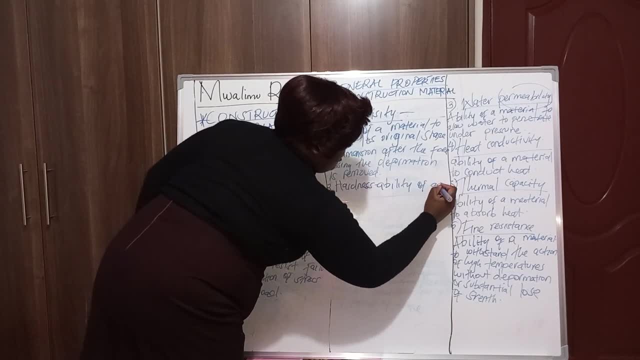 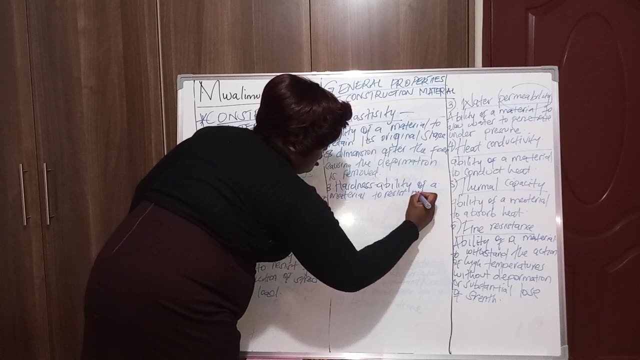 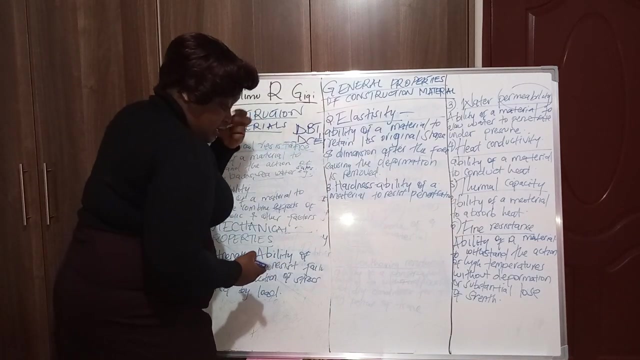 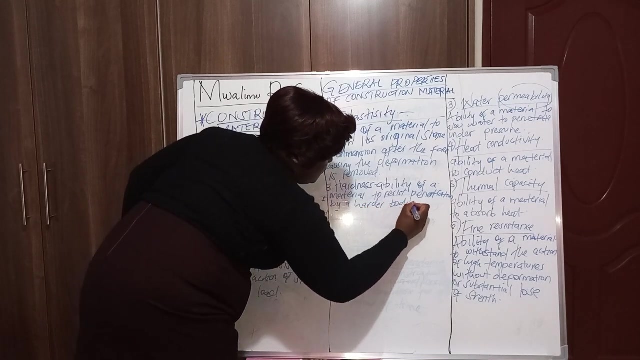 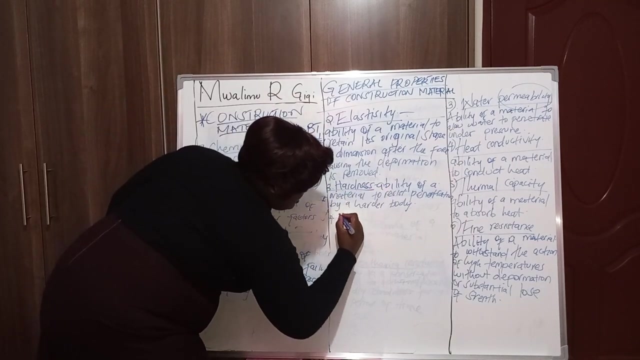 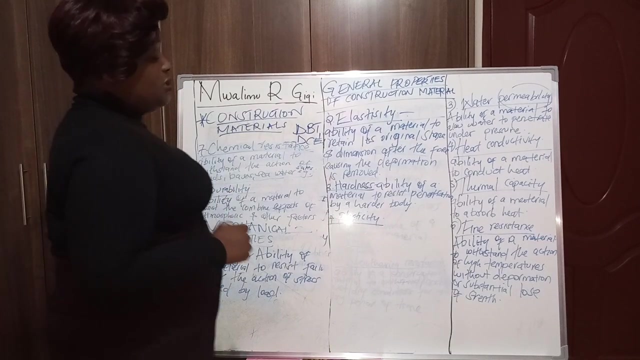 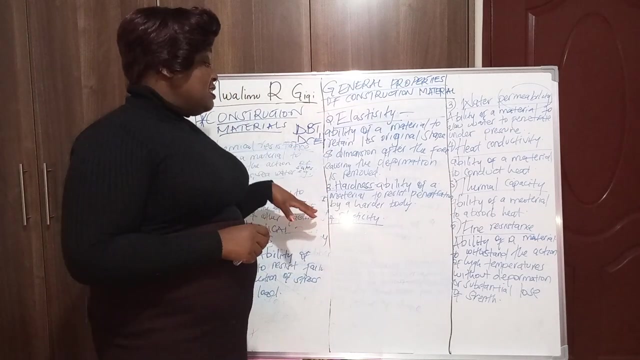 Ability of a material to resist penetration, To resist penetration, Penetration by a harder body. Number four: This is hardness, Elasticity. Number four: we have plasticity, Plasticity. So this one is when it's like not exactly the opposite of elasticity, but in this plasticity, 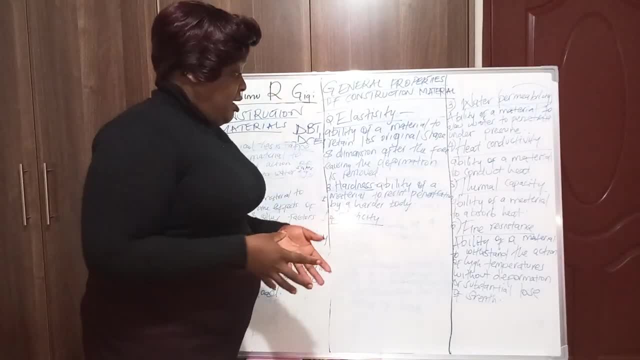 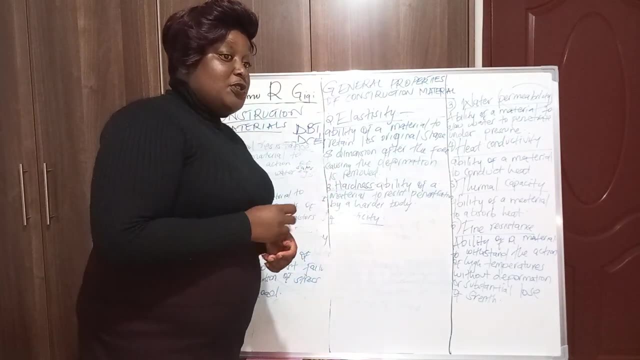 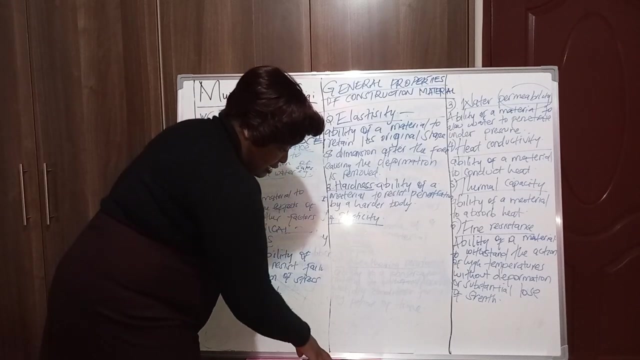 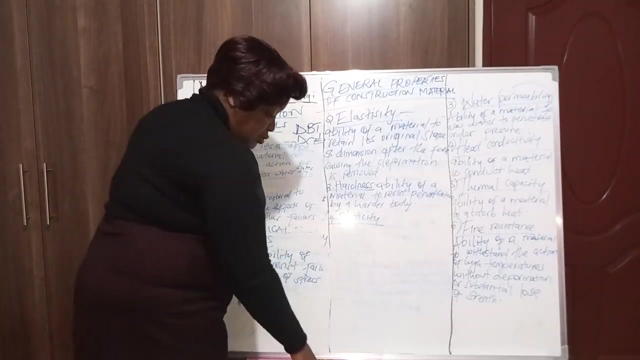 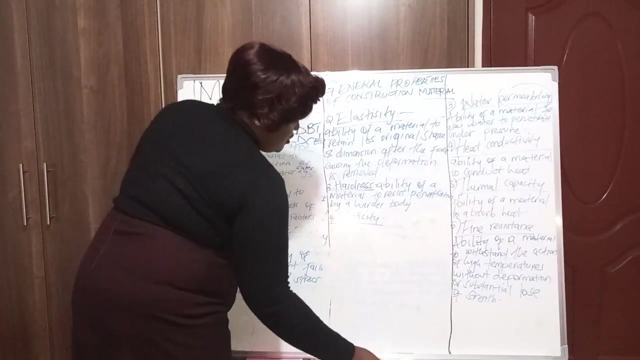 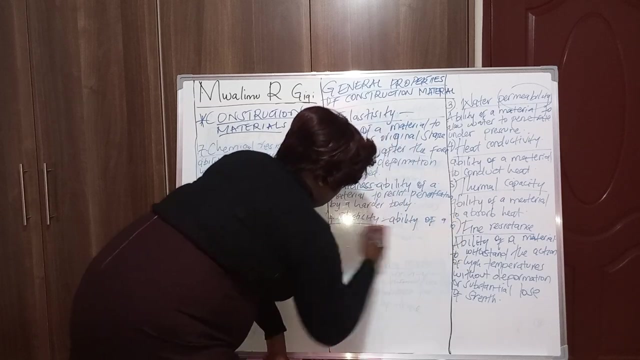 we can say that When a material will remain in that shape after the force causing the deformation is removed. So plasticity is the ability of a material to change its shape under load without cracking, And retain this shape after the load is removed. So we can write the ability of a material to change its shape. the ability of a material to change its shape. 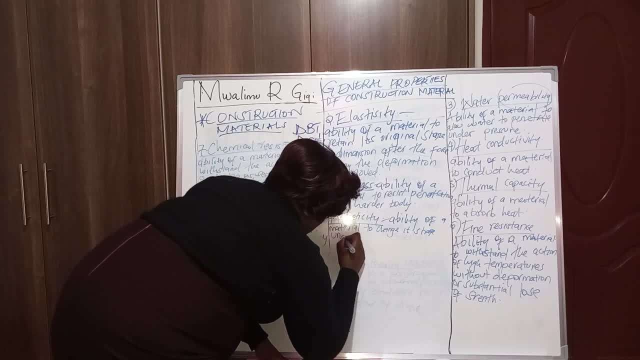 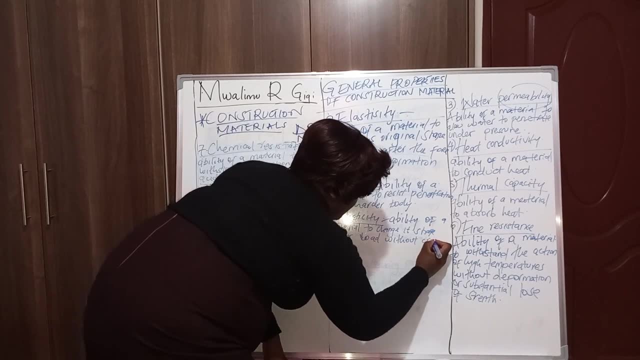 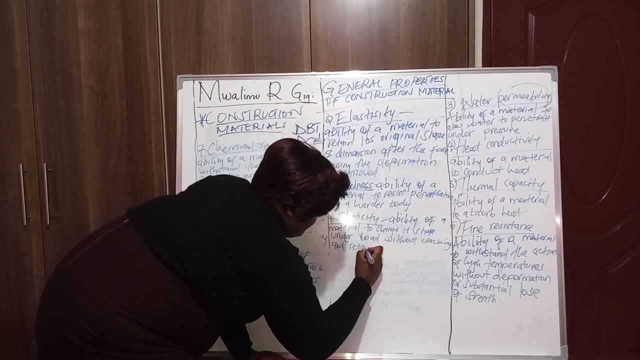 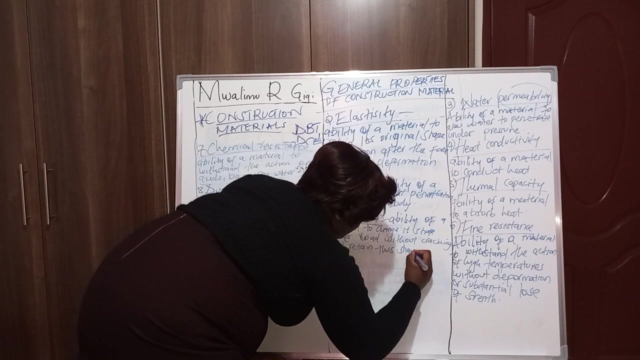 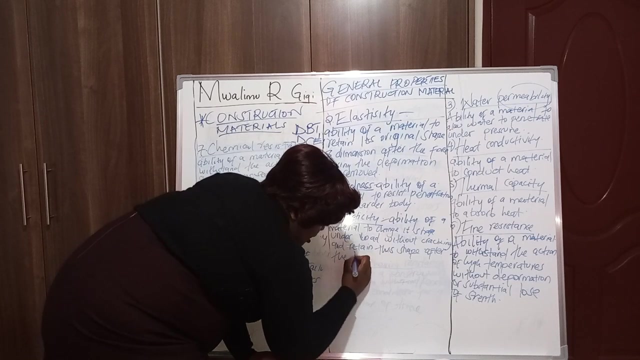 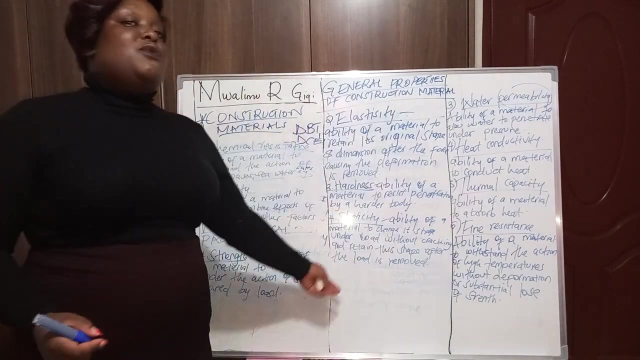 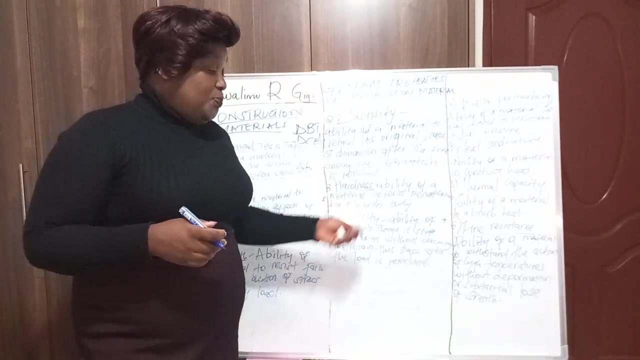 under load, without under load, without cracking, without cracking, and retain and retain this shape, this shape after, after the, after the load is removed. This one can be applied where For clay, When we want to make bricks out of clay. this property is a major 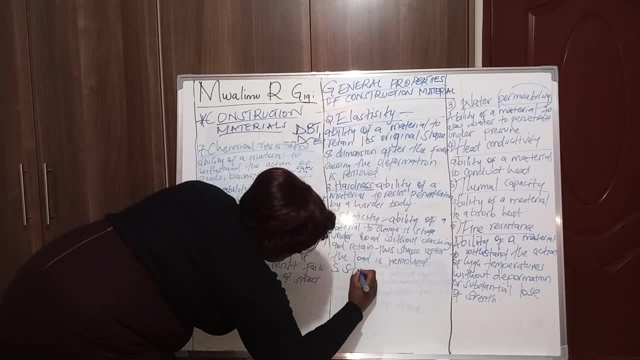 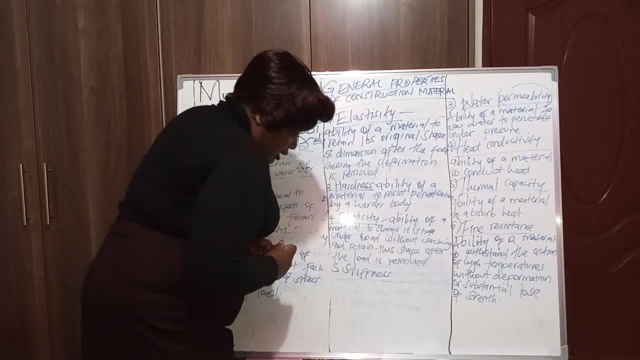 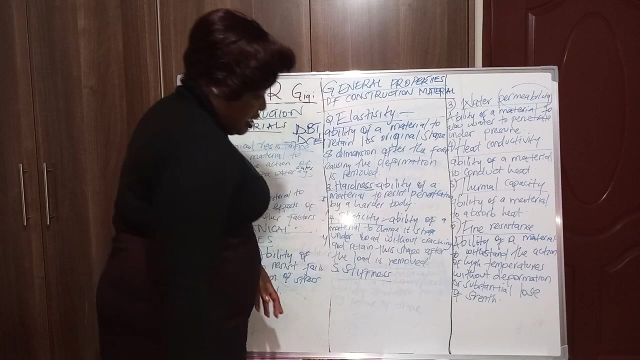 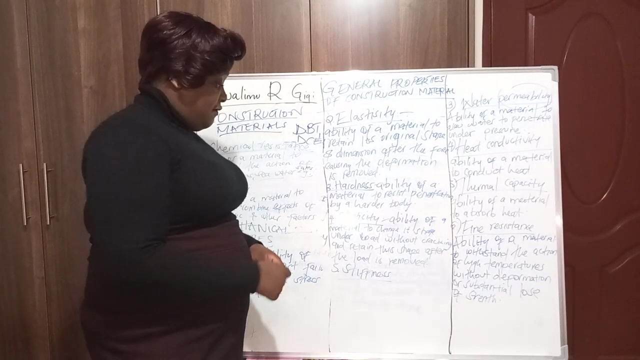 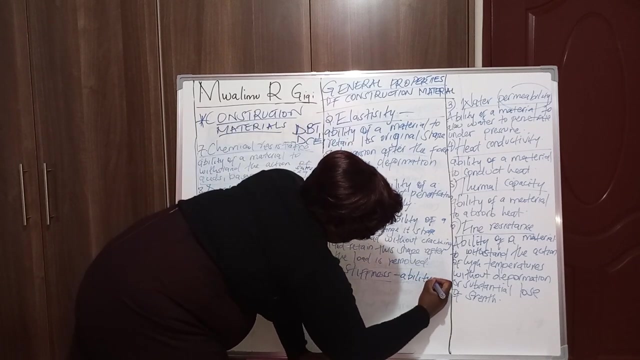 So, number five, we have stiffness, stiffness, stiffness, Stiffness is the ability of a material to resist elastic deformation or deflection. Uh-huh Stiffness: the ability of a material to resist elastic deformation. So the ability of a material to resist. 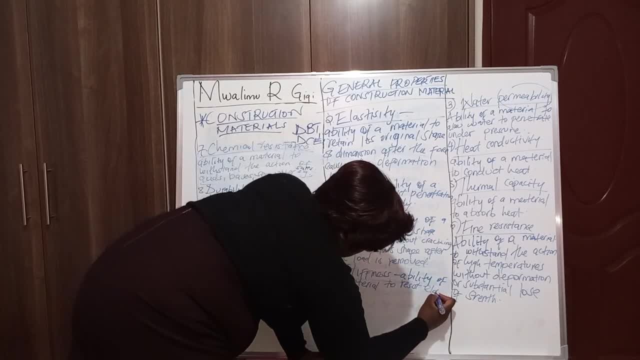 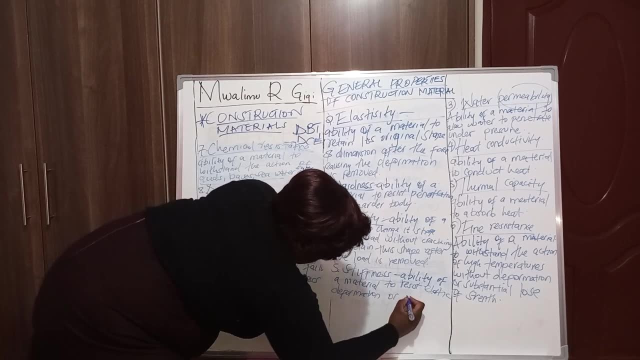 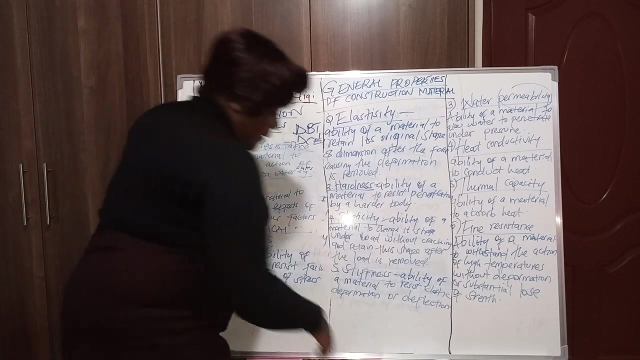 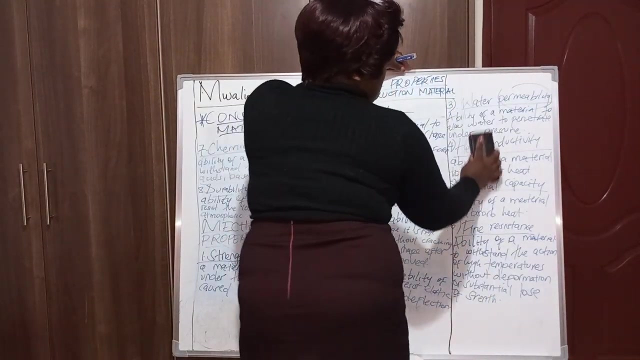 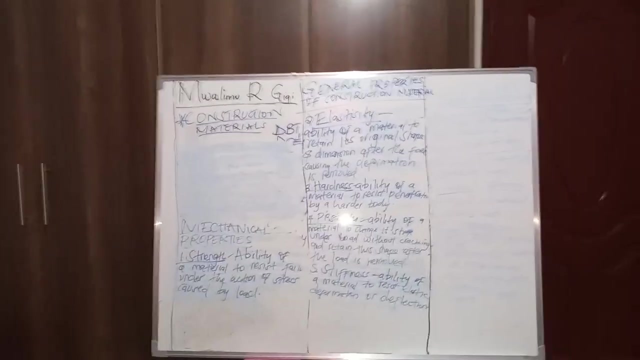 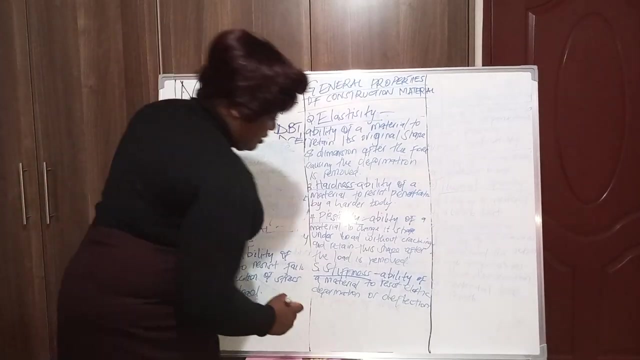 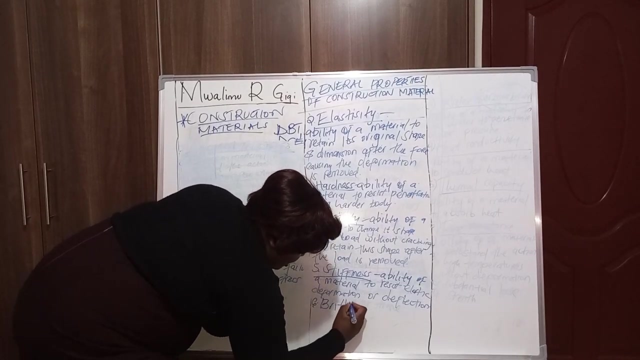 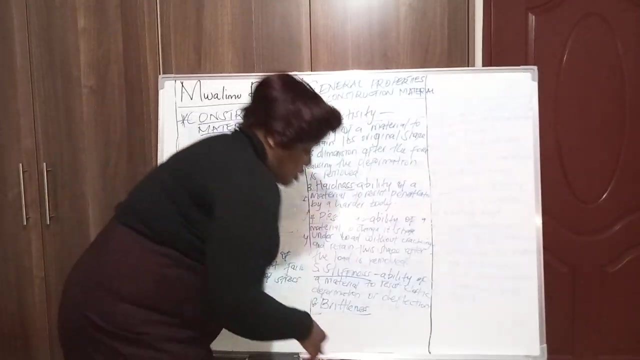 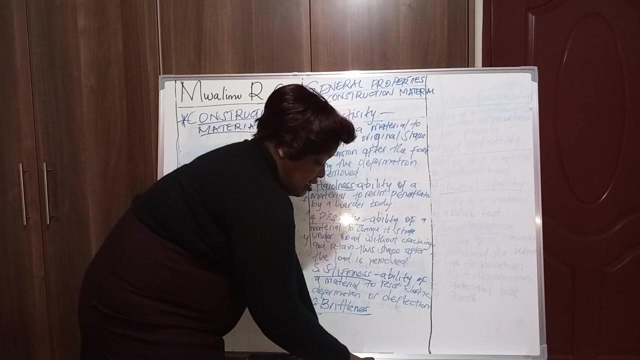 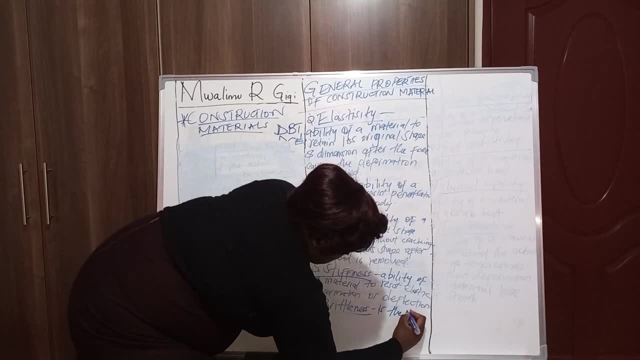 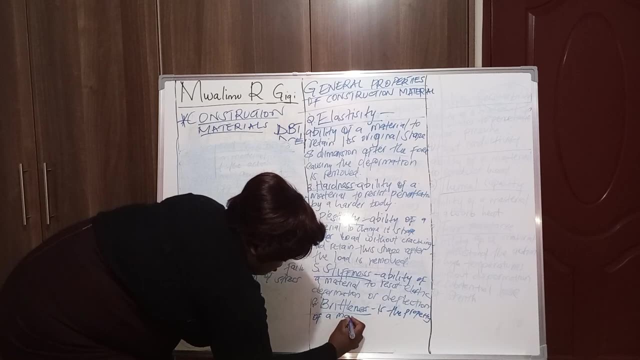 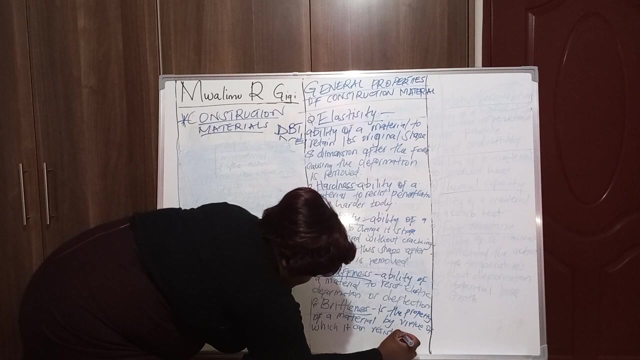 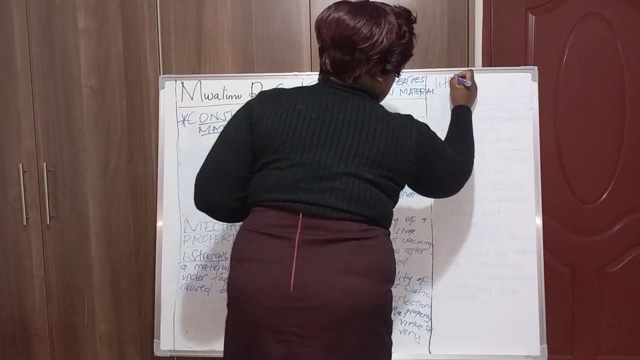 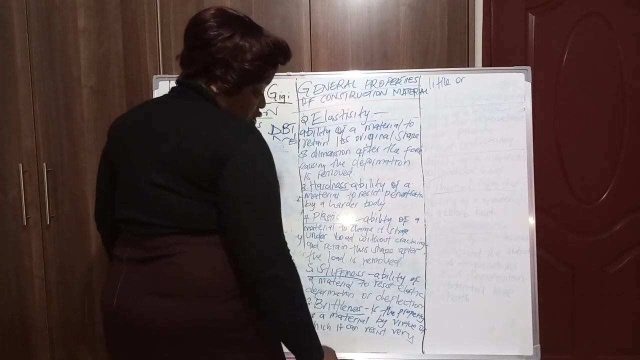 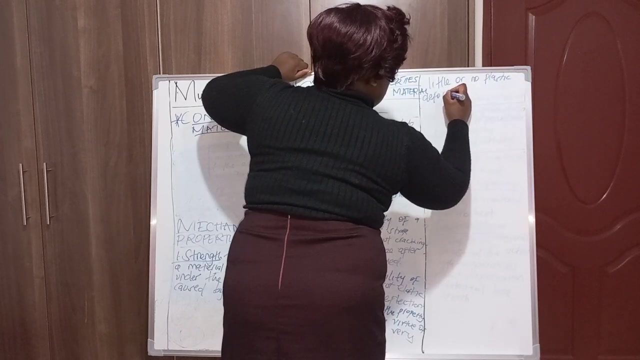 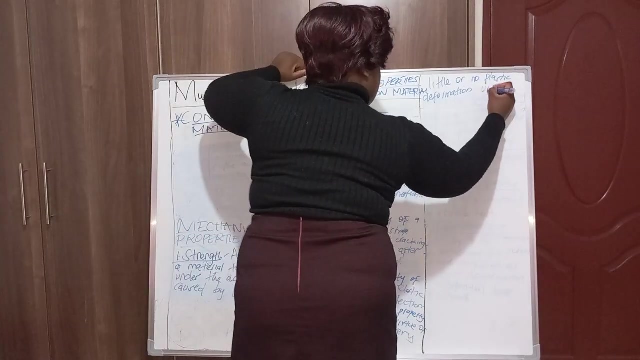 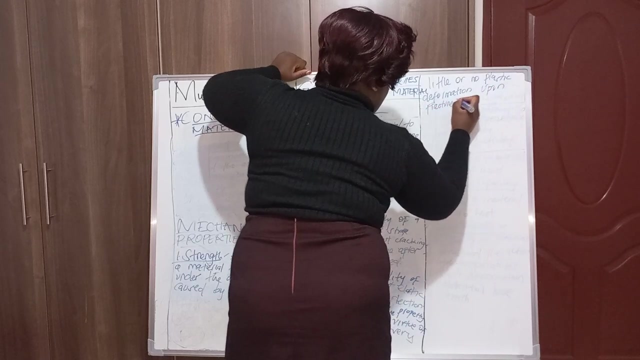 So we can write- is the property of a material by virtue of which it can resist. it can resist very- I can go to this side- very little or very little or no plastic deformation, no plastic deformation. no plastic deformation upon fracture, upon fracture. brittleness seven. 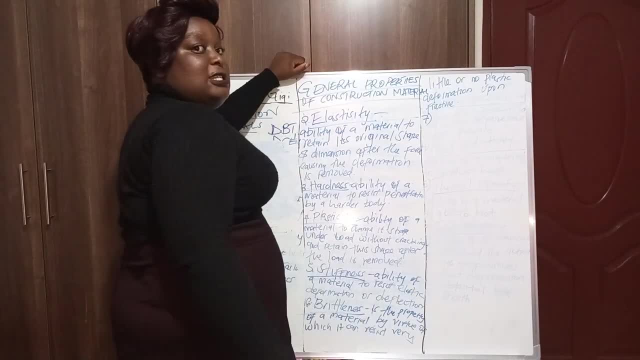 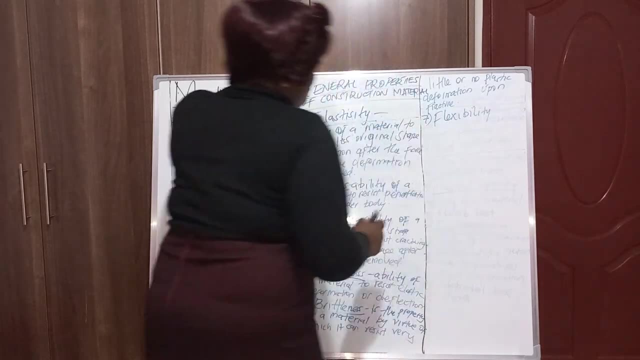 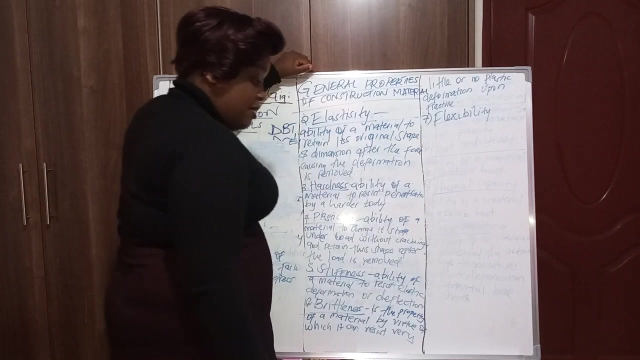 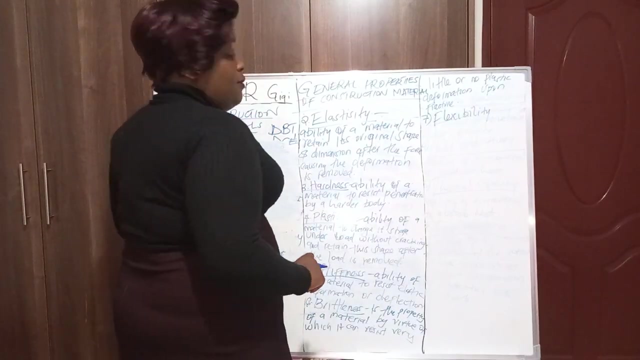 so number seven, we have flexibility, flexibility. flexibility from the word flexible, so flexibility. is the property of a material by virtue of which it can resist very little plastic deformation upon fracture upon fracture, a material of which it can bend without breakdown, so is the property of a 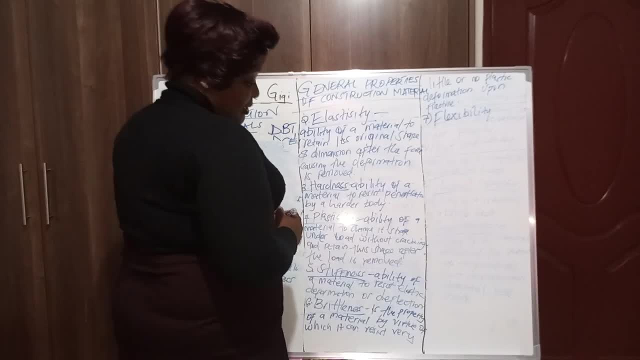 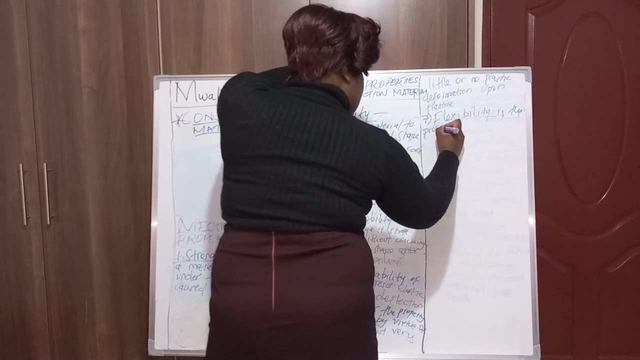 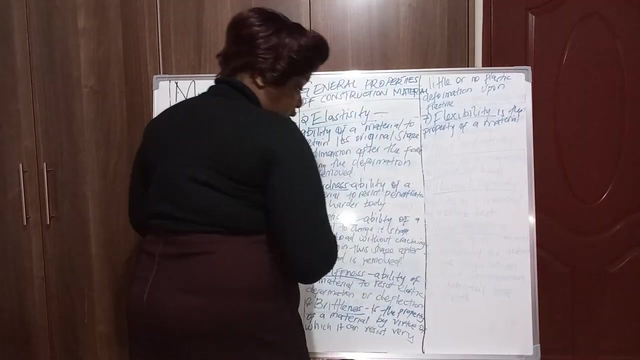 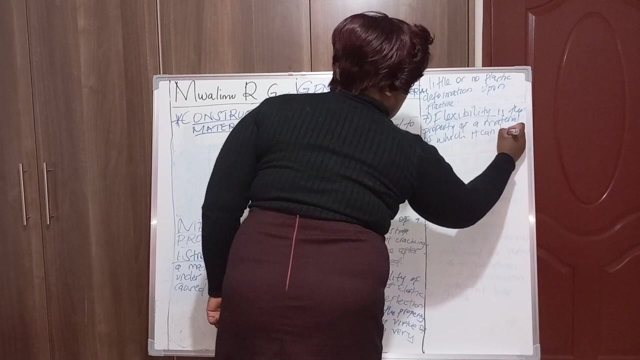 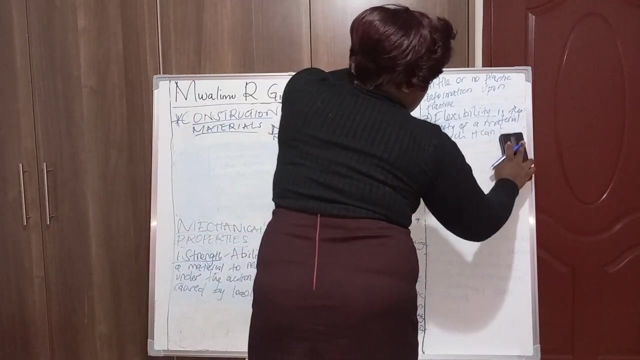 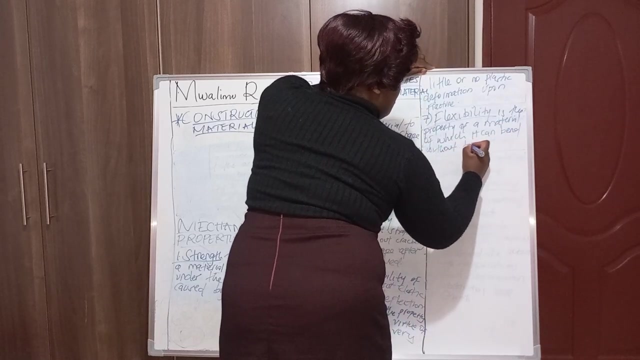 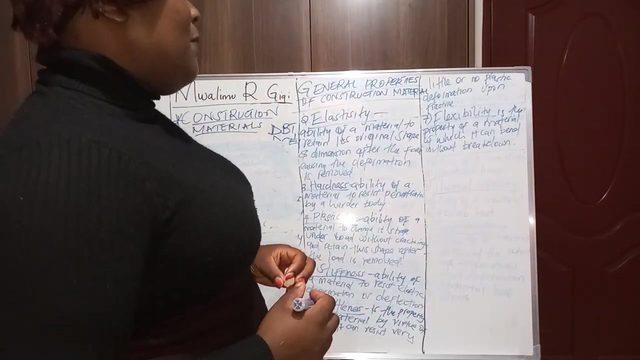 material of which it can bend without breaking. so is the property, is the property of a material. is the property of a material of which it can break, it can bend, sorry, it can bend without break down. it can bend without break down. hope you are getting something. so this flexibility is the property of a. 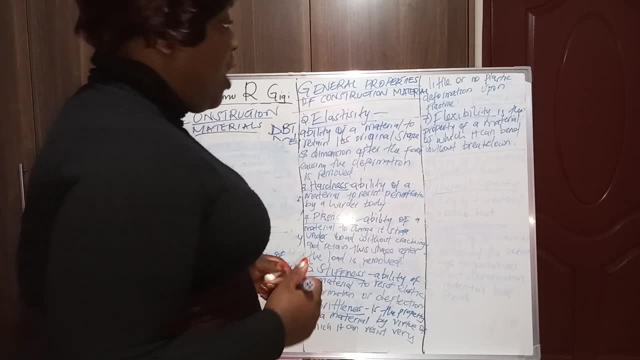 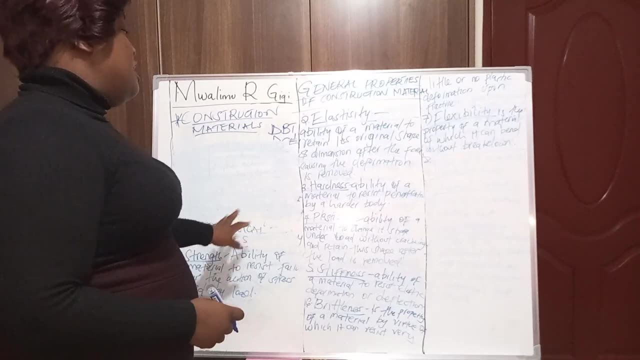 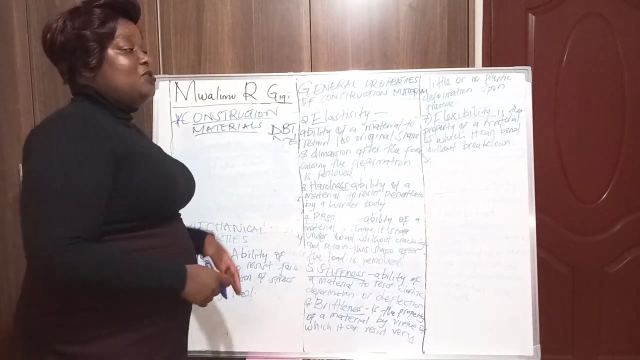 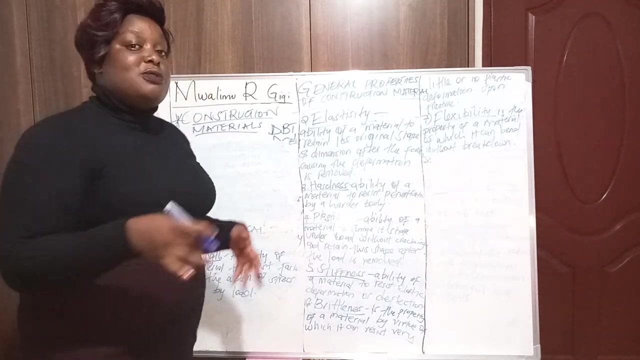 material of which it can bend without breakdown. number eight: number eight: we are talking about the mechanical properties of construction material. we have said that the mechanical properties of a construction material, they are just the behavior of a construction material under the action of laws or another information, plates of loads. are we together so we can continue? number eight: you can say toughness. 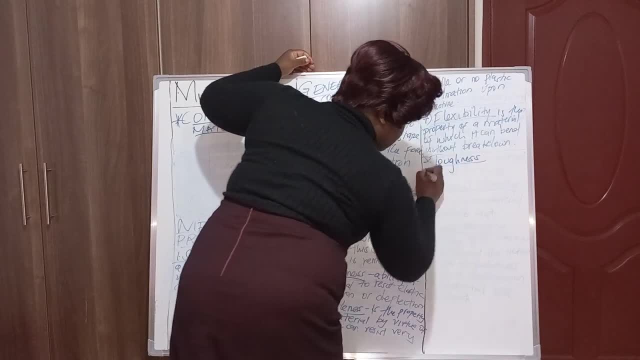 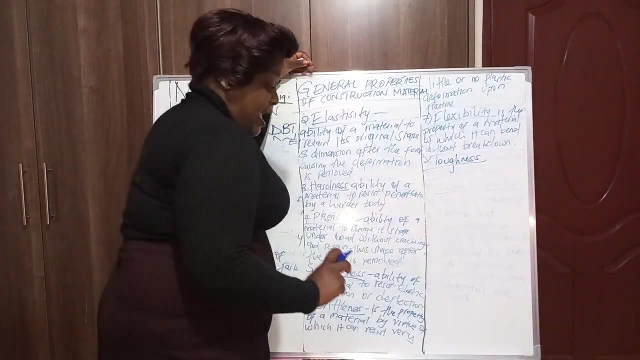 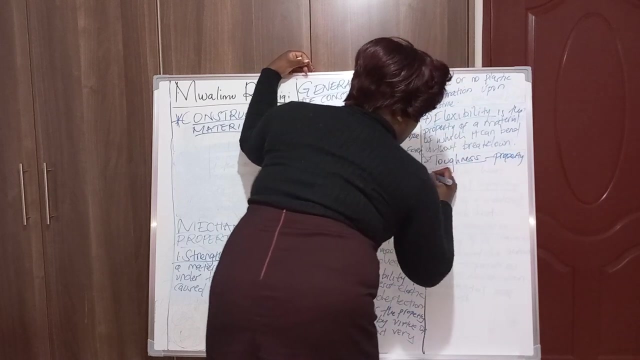 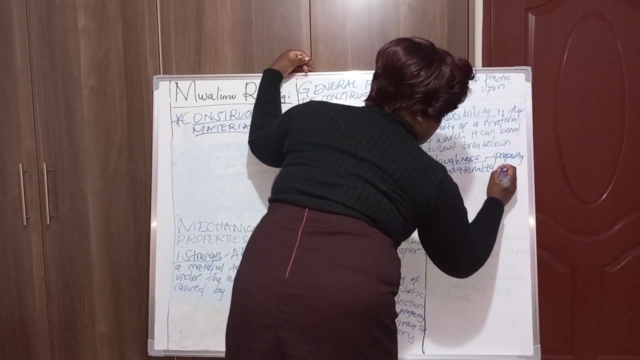 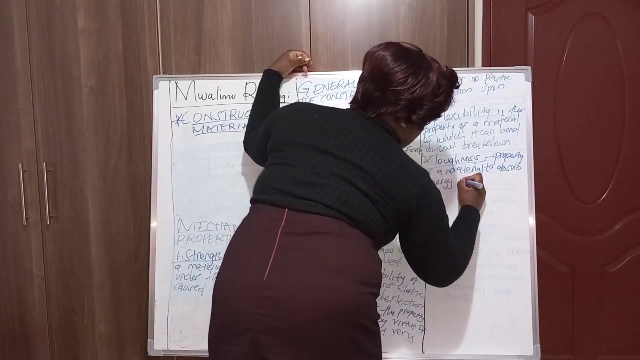 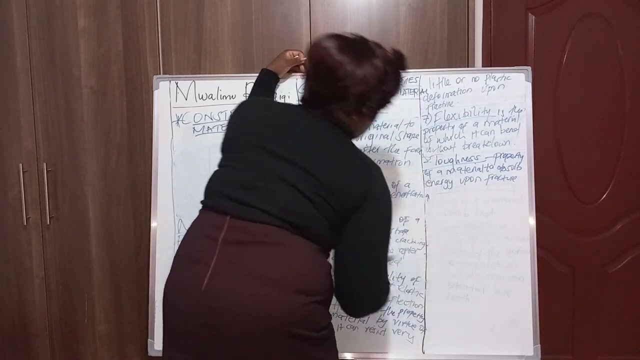 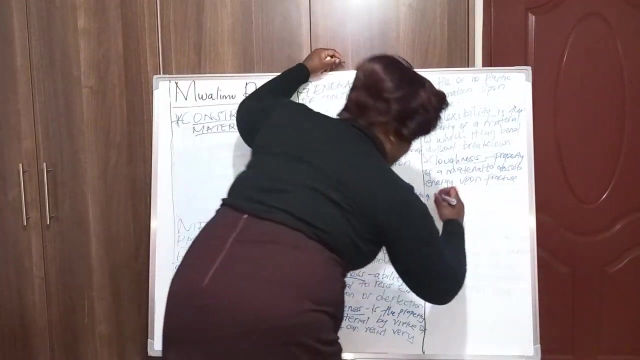 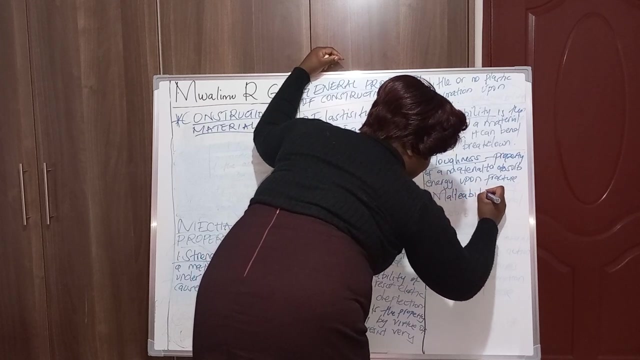 toughness. so a material should be tough. so toughness is the property of a material to absorb energy upon fracture. so it's the property of a material to absorb, to absorb, absorb energy upon fracture. the last one, lastly: we have malleability. this is just the ability of a material that can be shaped. 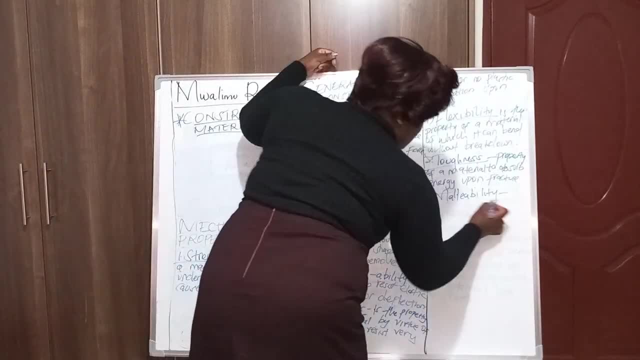 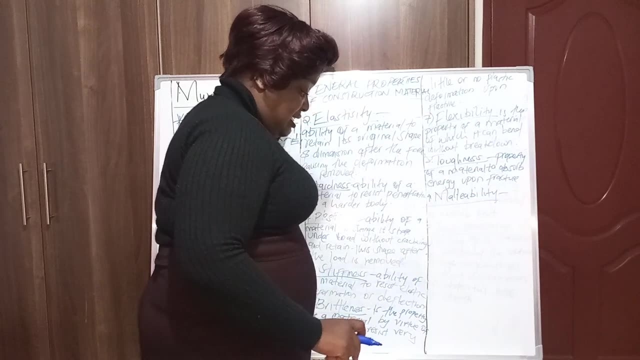 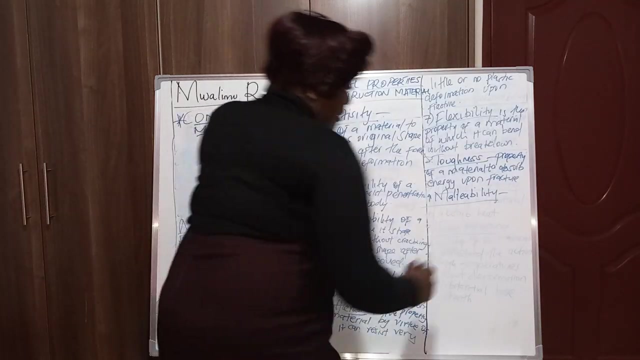 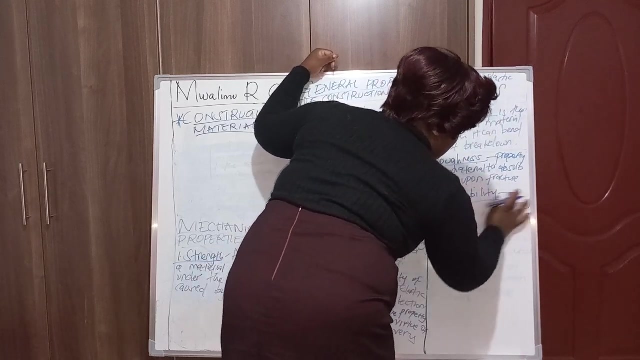 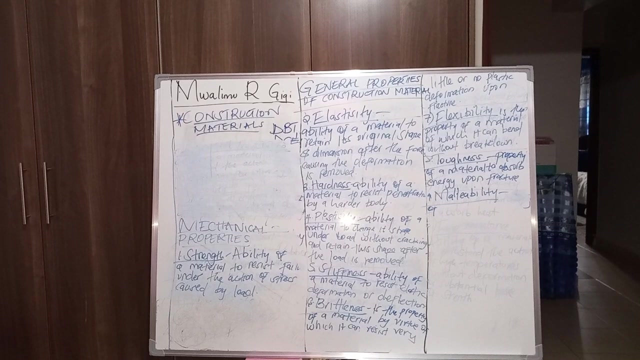 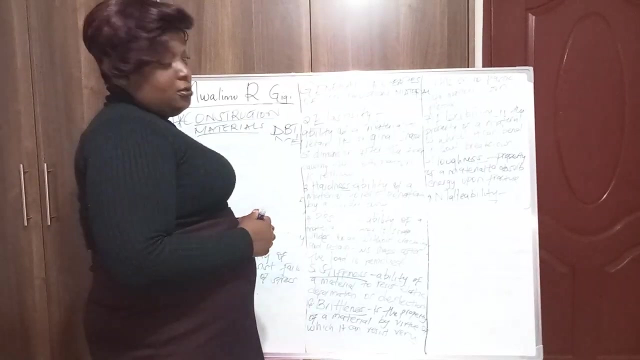 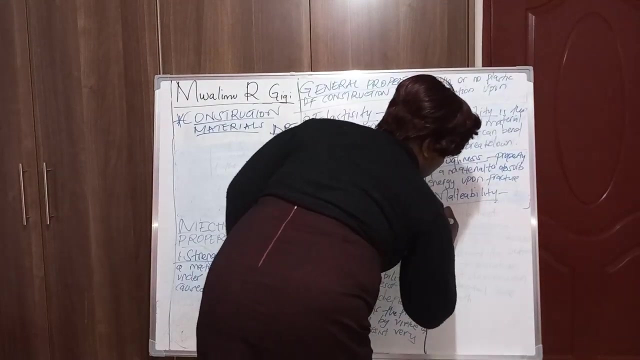 can be shaped to other forms without a bracket. so we can. we can write the ability of a material to be flattened into sheet without a rapture: the ability. The next property is malleability. malleability, we say, that is the ability of a material to 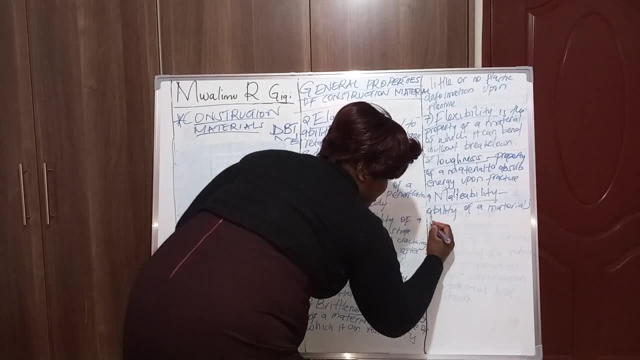 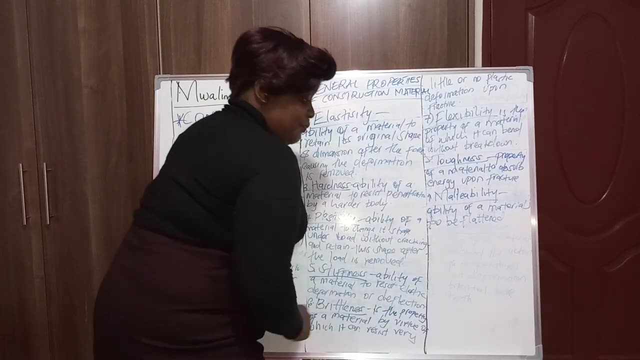 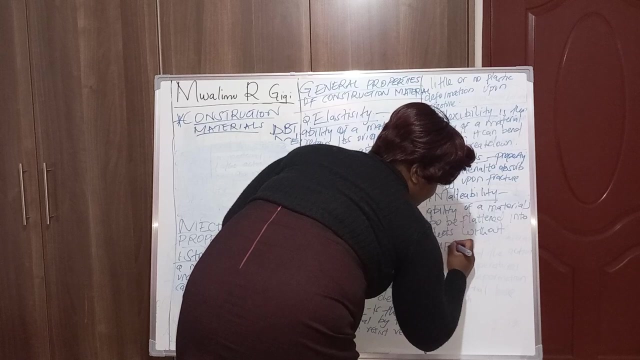 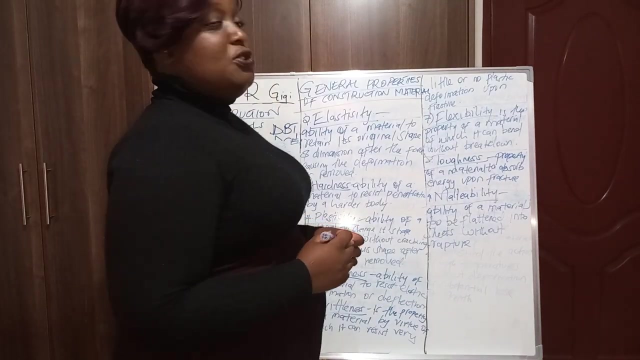 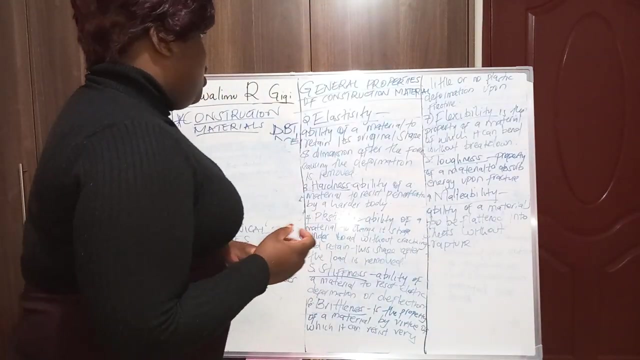 a material to be flattened, to be flattened, to be flattened into sheets, into sheets without rupture, without rupture. rupture, Rupture, Rupture. That is the ability of a material to be flattened into sheets without rupture. so that is malleability. 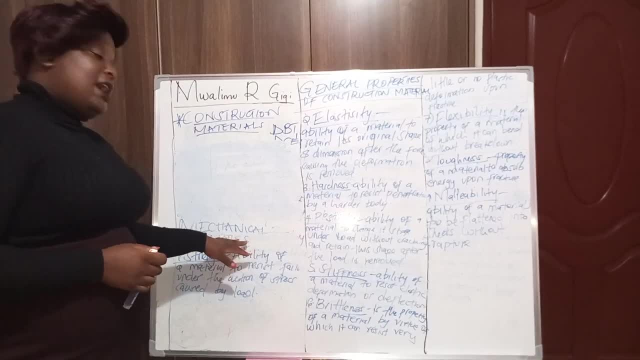 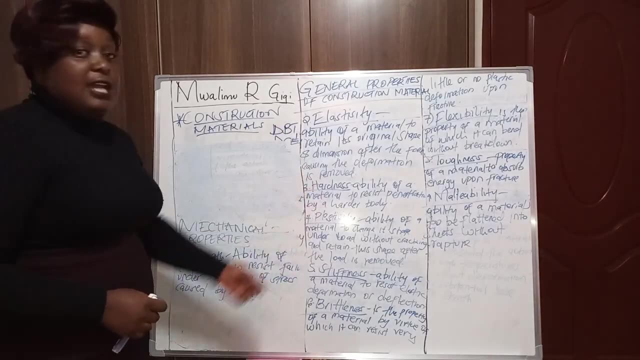 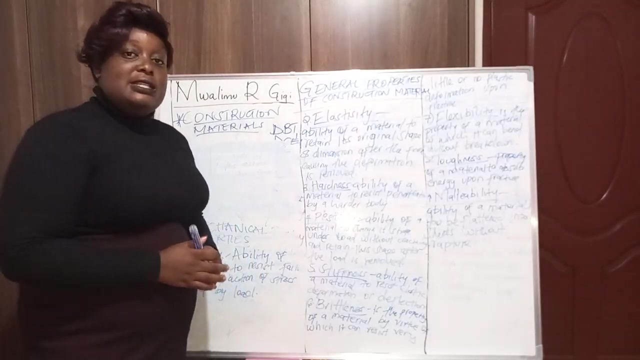 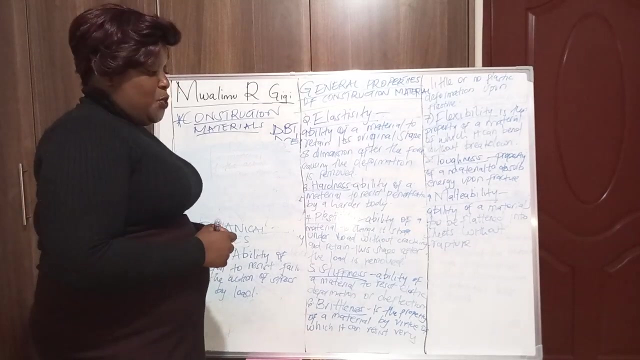 So that is the end of mechanical properties of construction material. We have strength, elasticity, hardness, plasticity, stiffness, brittleness, flexibility, toughness and malleability. So we will go to another subtopic, which is classification of construction material. 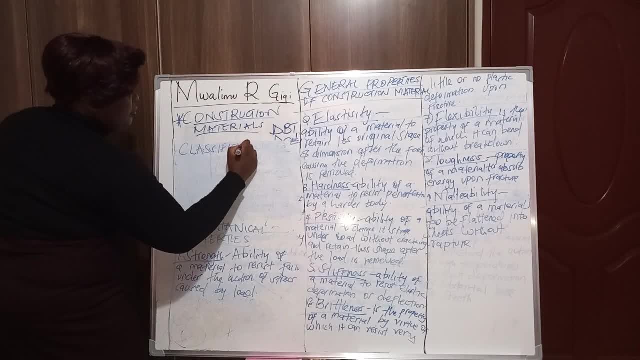 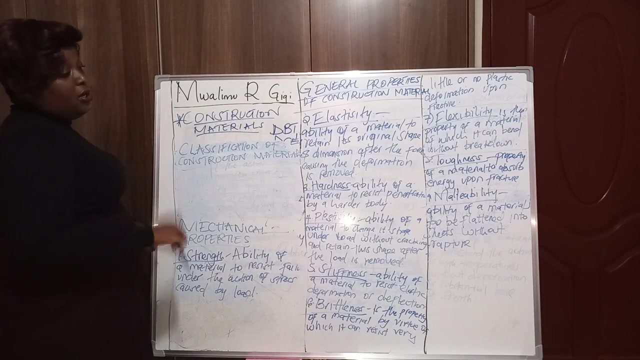 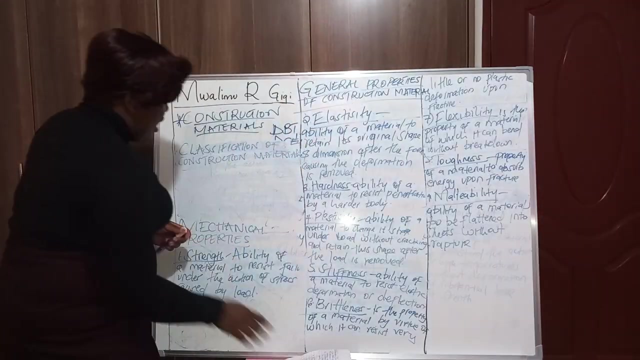 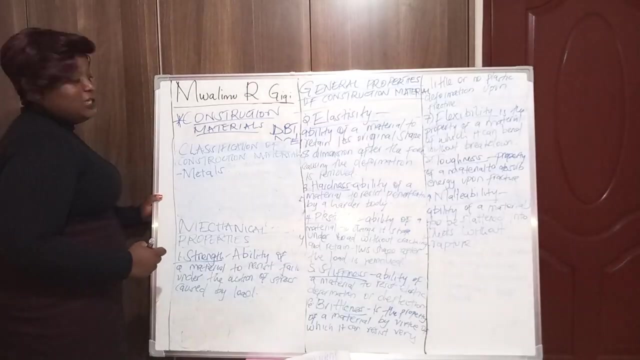 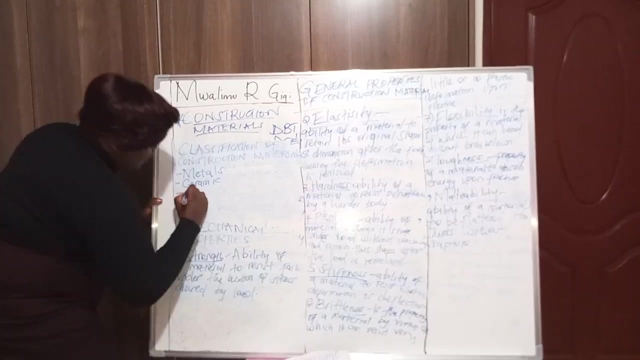 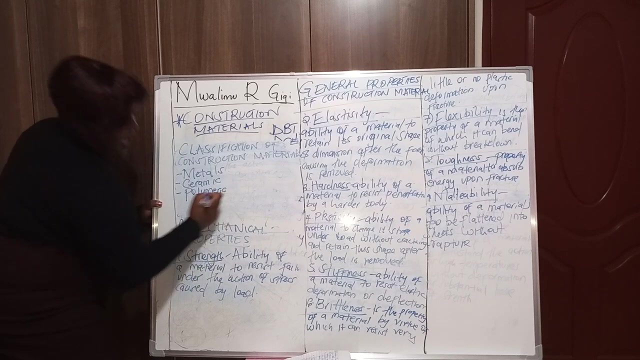 So classification of construction, Classification of construction materials. So materials are classifications classified into four. so we have metals, we have materials which are metals, we have materials which are ceramic and we have materials which are polymeric, poly polymeric, and we have materials which are composite. 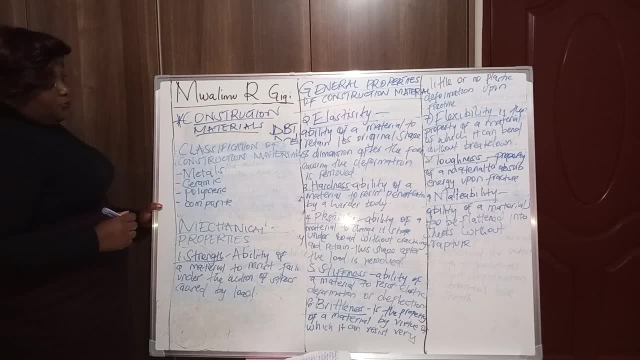 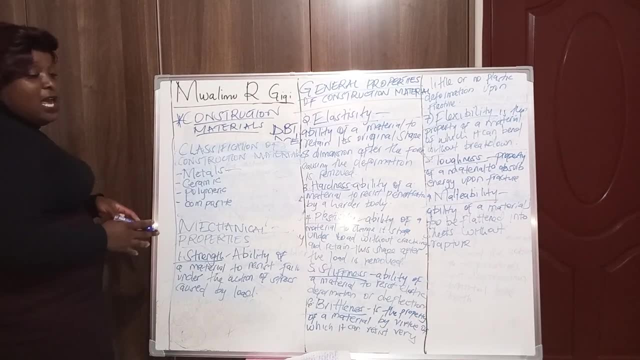 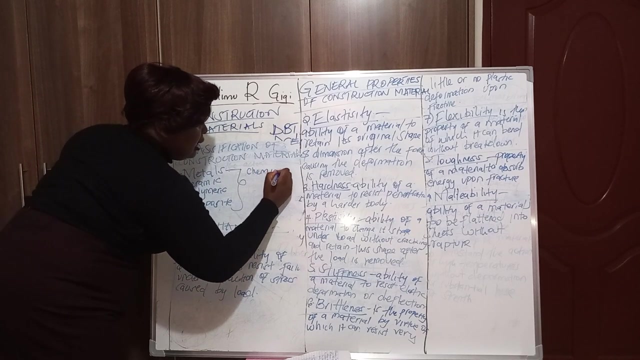 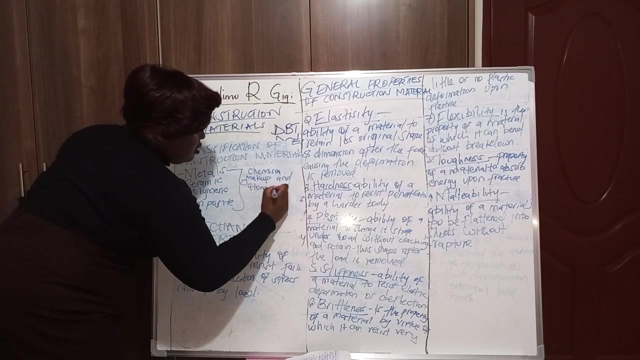 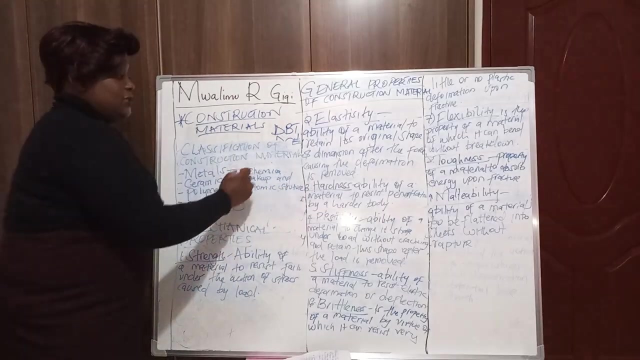 composite uh material. so uh for metals. uh it's also further classified, so this classification is based on the chemical makeup and atomic structure. so we classify material based on chemical makeup and the atomic structure uh. so when you classify materials- uh- based on chemical makeup and atomic structure. 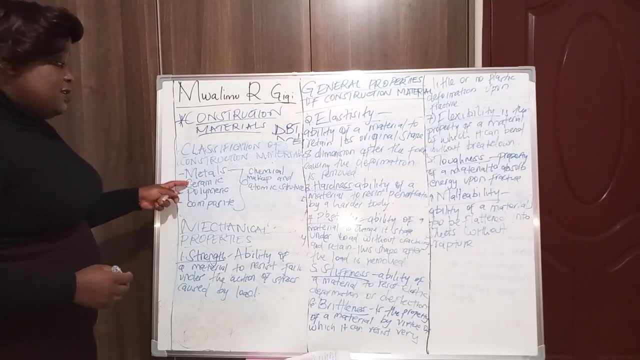 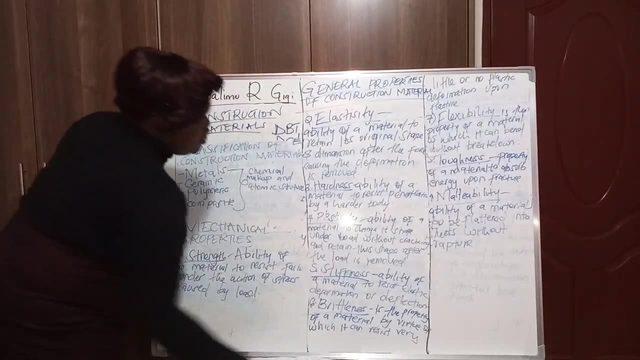 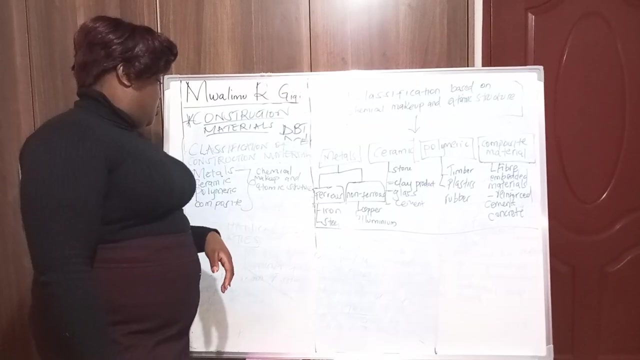 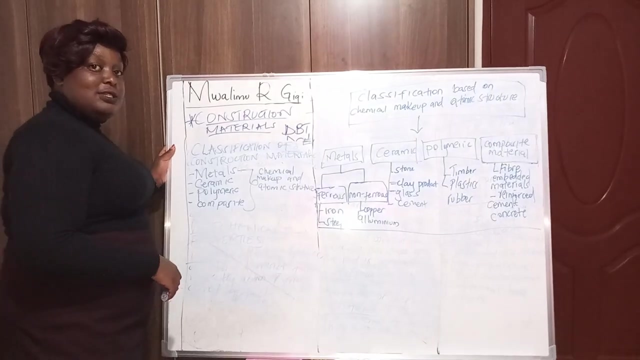 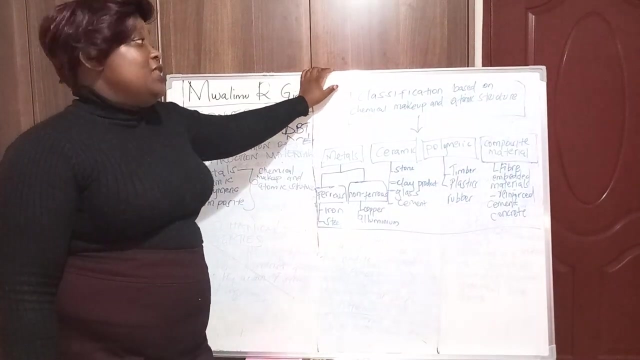 we have metals, we have ceramic, we have polymeric and composite material, so we can have a chart, we can have a chart, so we want to continue. we have said classification of construction materials. we have metals, ceramic, polymeric and composite material. so this is just a chart to show the classification of 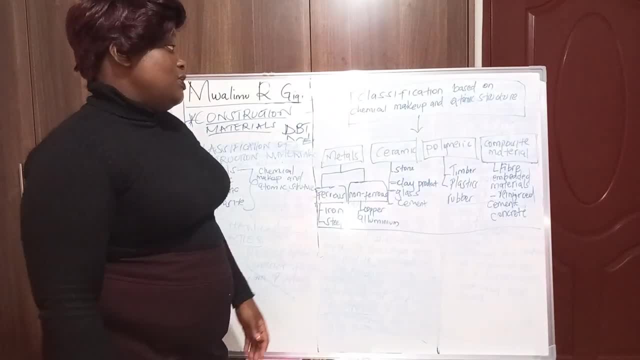 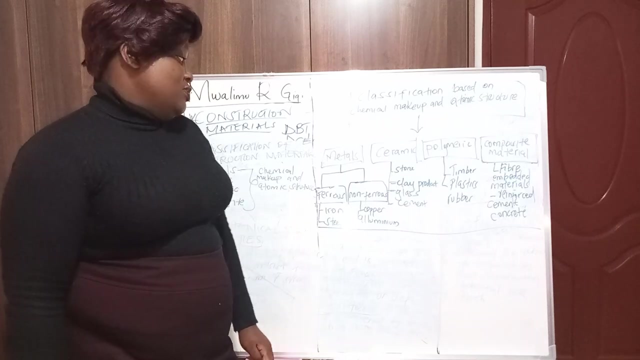 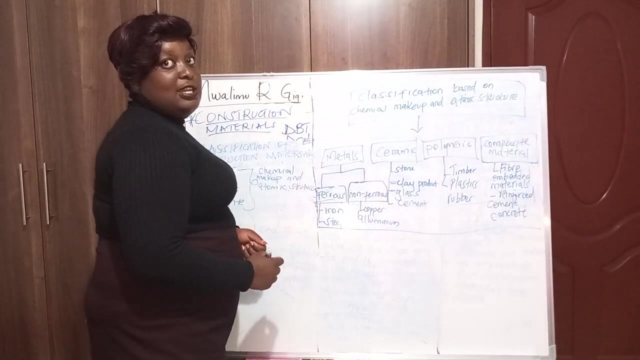 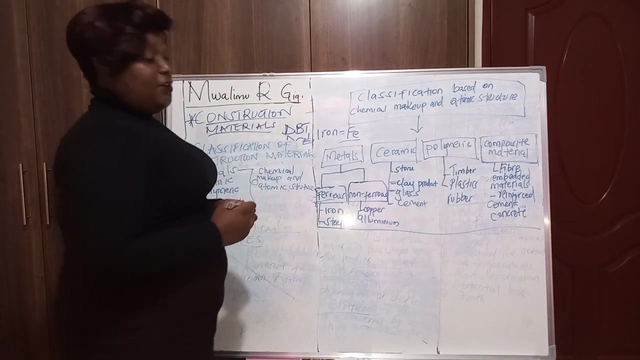 construction material based on chemical makeup and atomic structure. we have metals, ceramic, polymeric and composite material. so metals are further classified into two: ferrous and non-ferrous metals. so from the word ferrous there are metals that contain ion, because ion is written f? e. so ferrous materials, there are materials that contain. 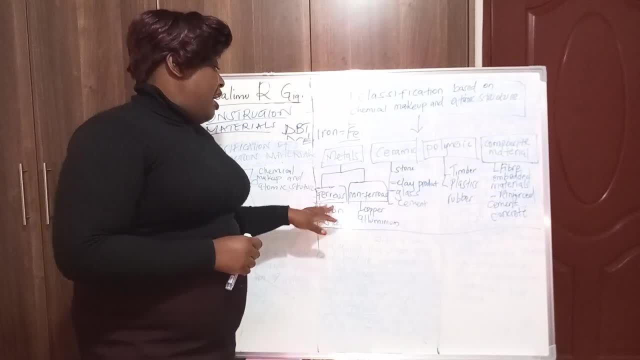 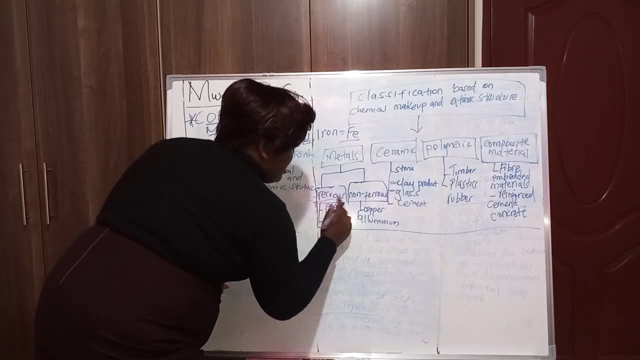 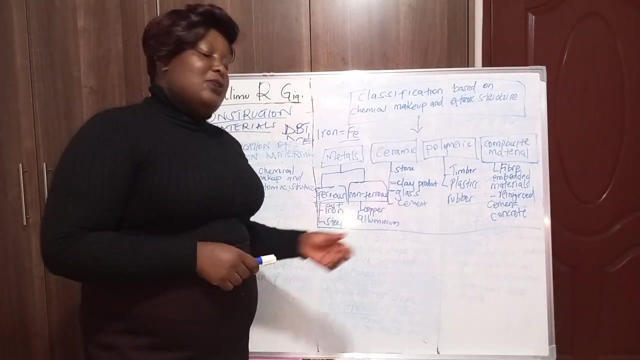 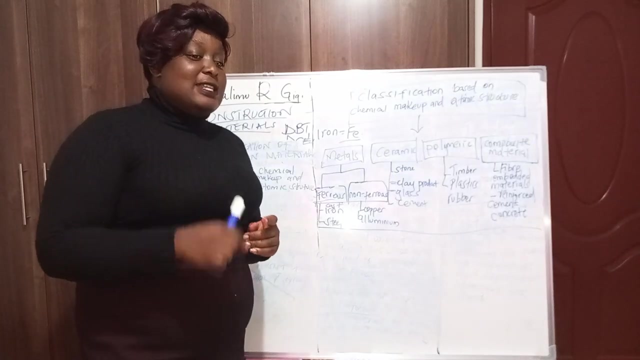 and there are metals that contain iron. examples of iron and steel. so here we can have cast, cast ion and steel. now for non-ferrous- uh, for non-ferrous material metals. there are metals that does not contain iron or it has very little. that is, uh, not recognized. 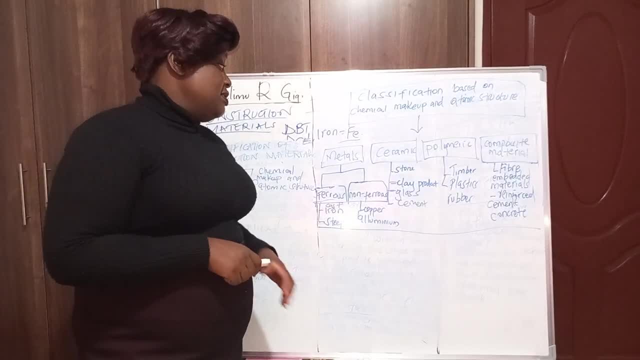 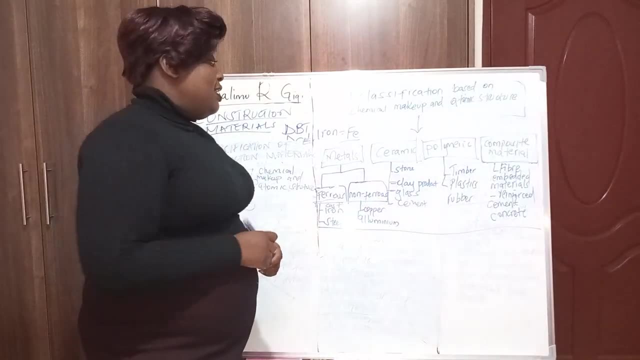 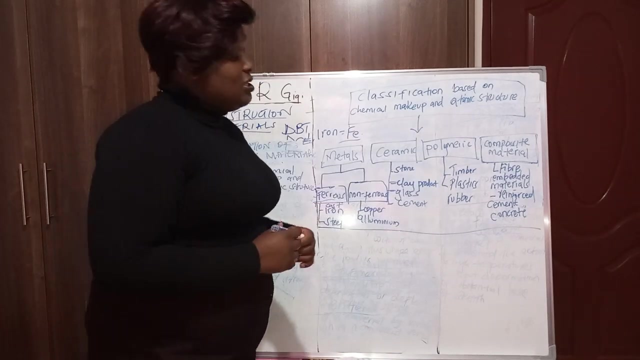 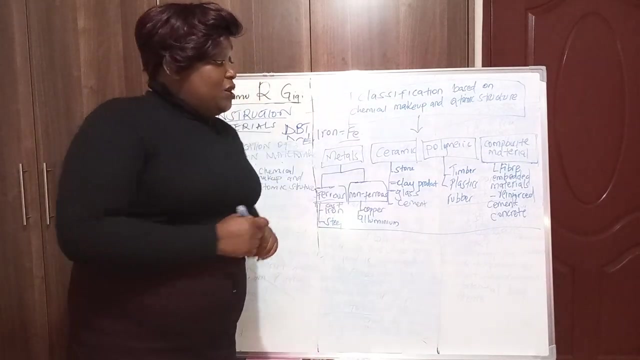 iron. so we have, example, we have copper and aluminium. so for ceramic materials, they are materials that are brittle, they break easily. so we have stone clay products, we have glass and cement. for polymeric materials, they are materials made from organic molecules, so we have timber, plastics and rubber and lastly, we have composite materials. 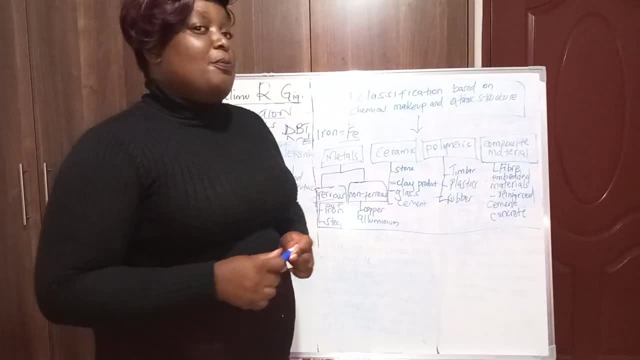 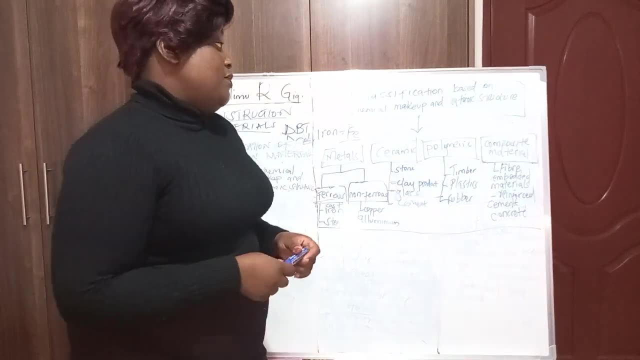 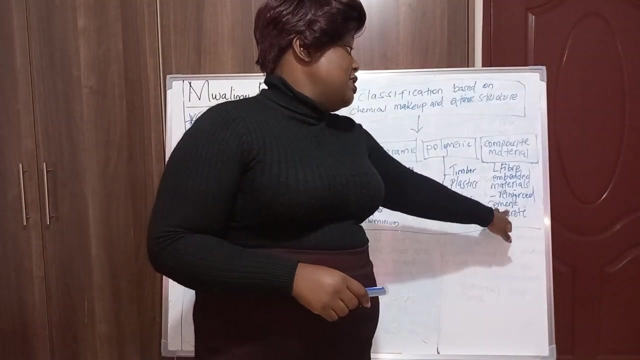 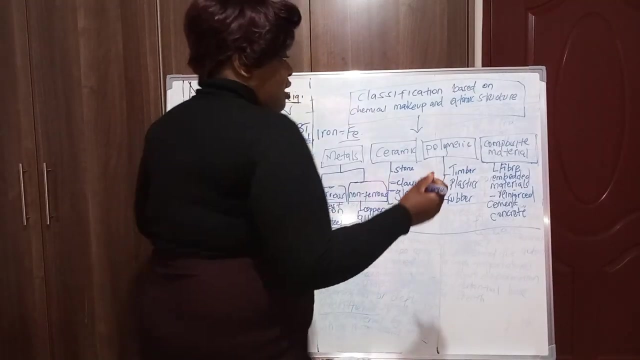 they are just materials that are formed out of a combination of all of the construction material. for example, we have fiber embedded materials and we have reinforced concrete, reinforced cement concrete. so example I can, I can give an example of a composite material: reinforced cement concrete. when you say 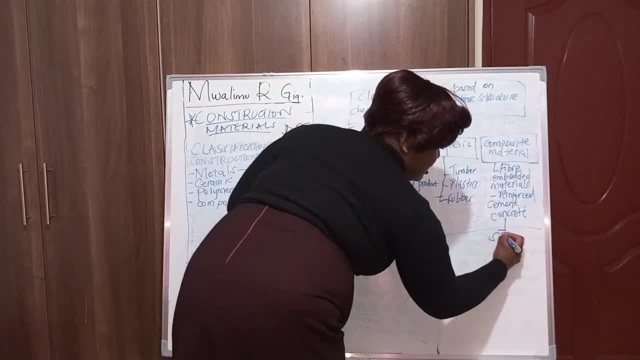 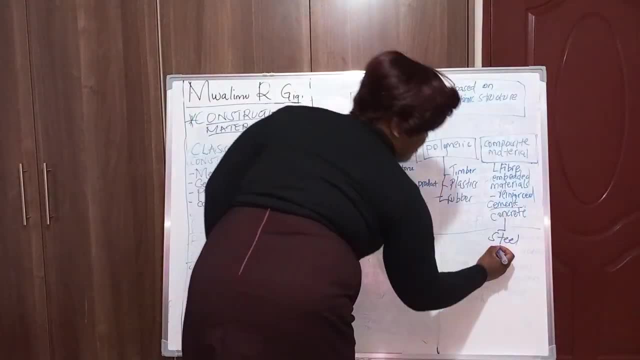 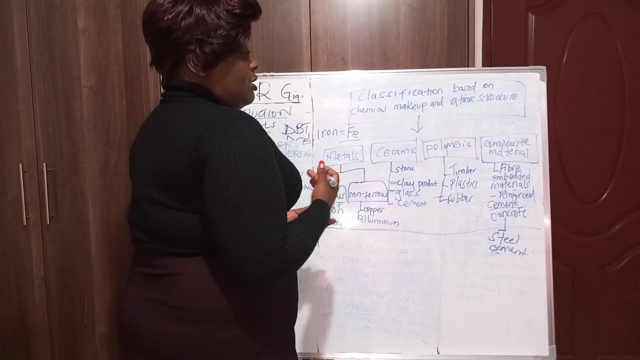 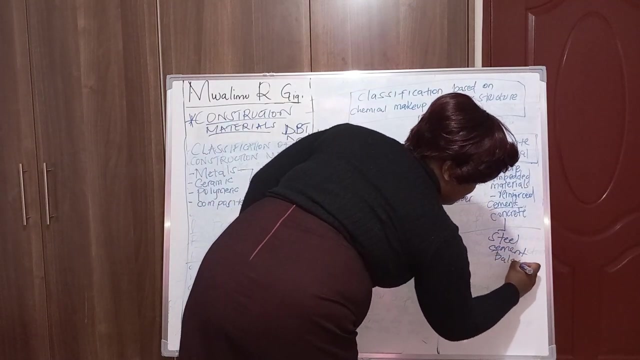 reinforced cement, concrete. we say that it has steam, okay, so it has steel for reinforcement, and then it has cement and it has concrete is a combination of cement and sand and ballasts, you know. so we can say ballasts because we have cement. so this is an 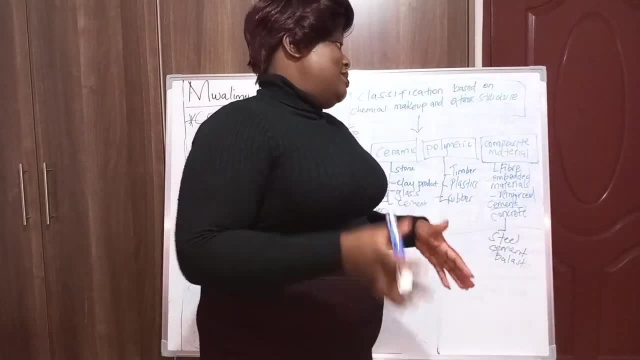 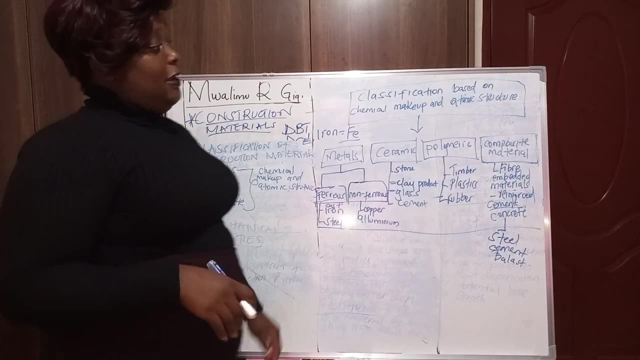 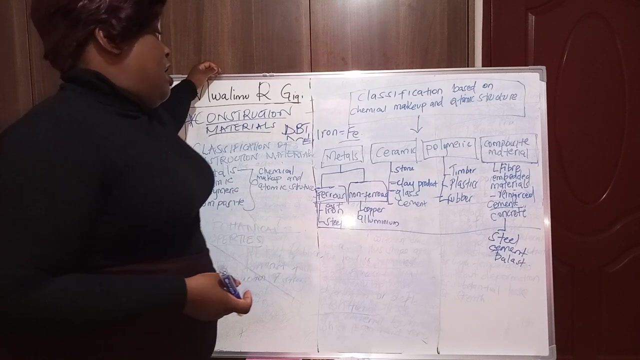 example of a composite material. it's just of concrete. we mild, a feel gaseous or thermos skimpers, and we have marble board which are used in lot uh sized ık combination of other construction materials. so this is basically a classification of construction material. for metals, they're just metals. we have two, ferrous and non-ferrous ceramics. 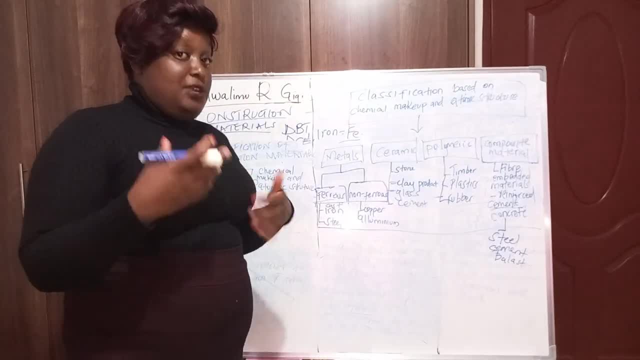 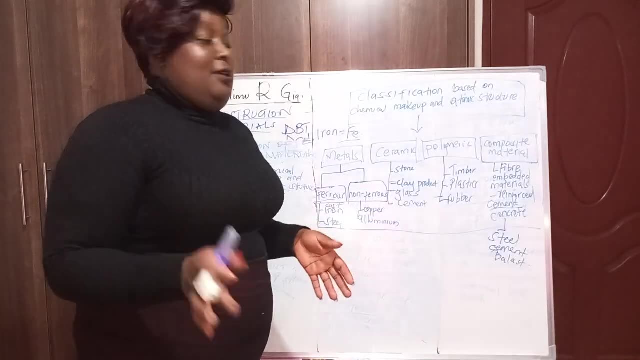 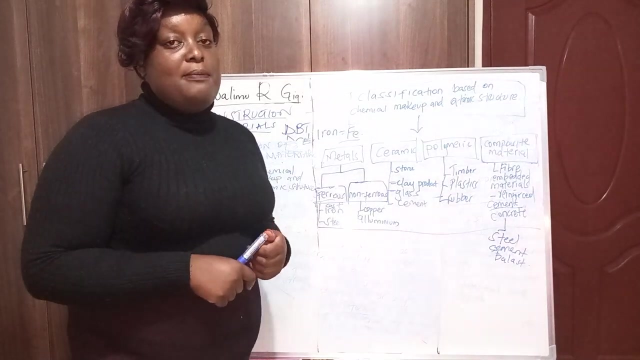 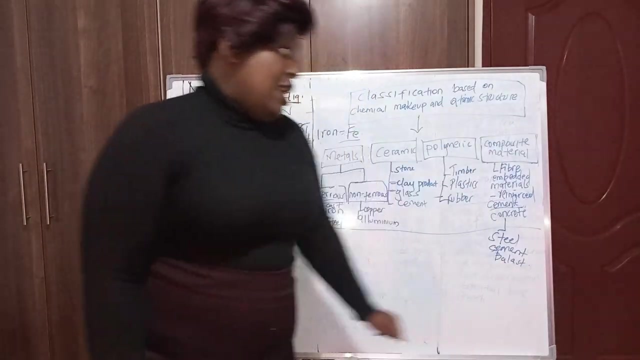 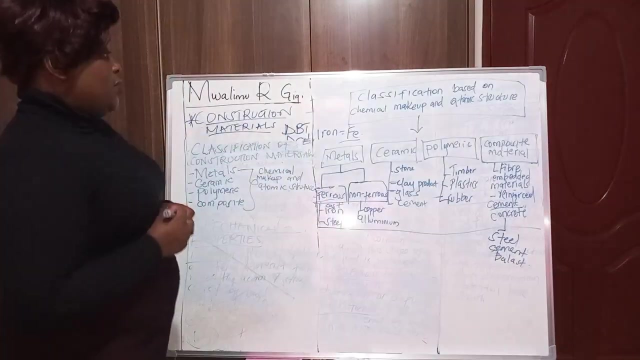 they admit their materials that that are brittle, they break easily. so, like stone, clay products and glasses, they break easily. and for polymeric materials, they are materials made out of made up out of organic molecules. and for composite material, they are material com a combination of construction materials. hope we have understood that. so we go to our next. 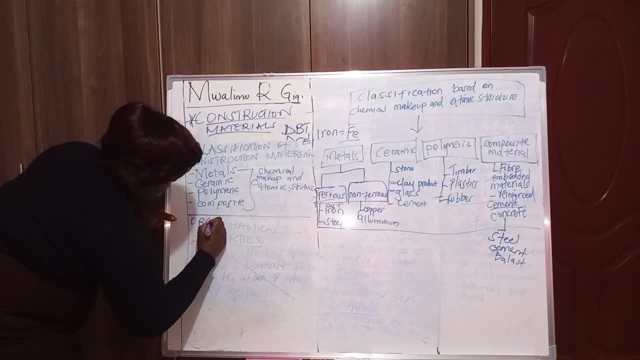 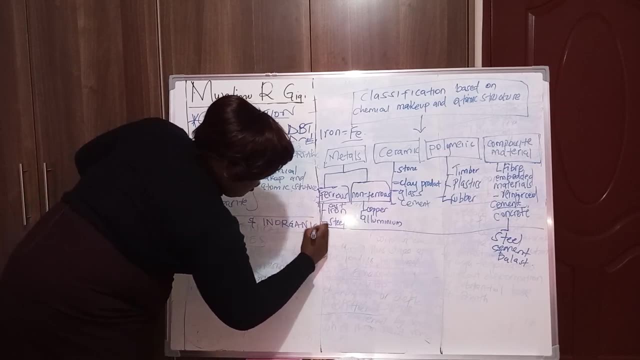 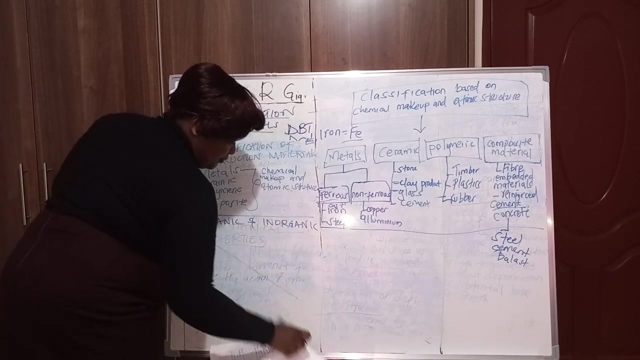 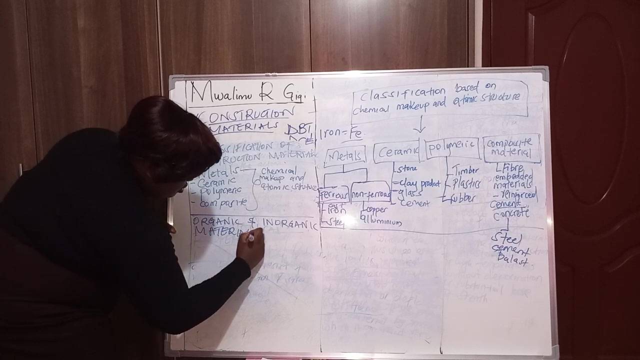 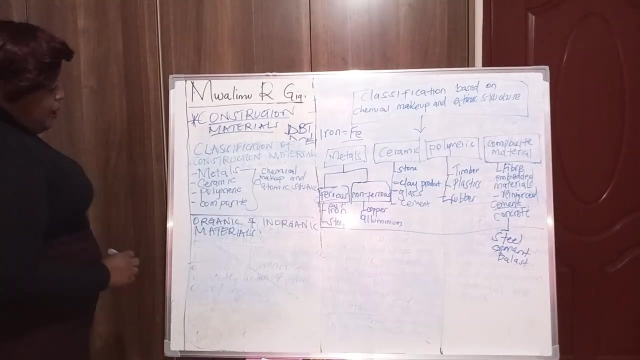 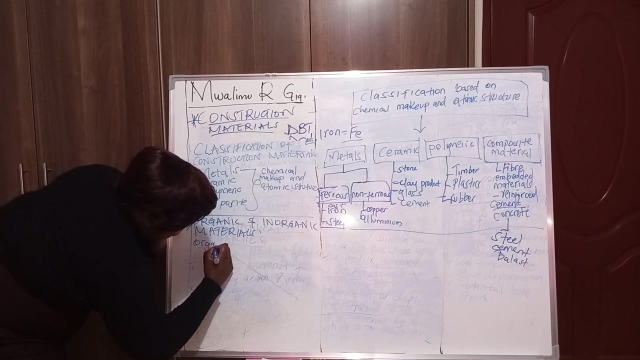 our next subtopic is our organic, organic and inorganic, organic and inorganic, organic and inorganic materials. so we want to differentiate between organic and inorganic materials. out of our knowledge we know that organic material we can start with organic, organic material. they are, they are basically natural. they are natural. 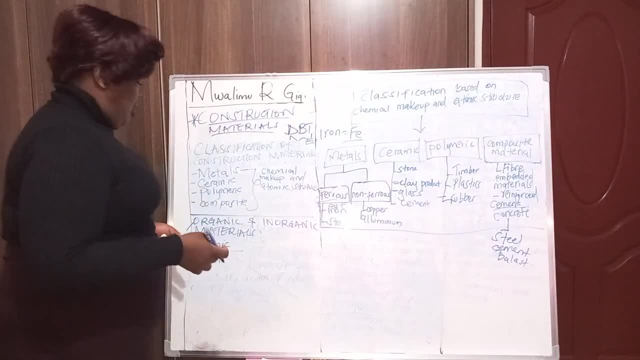 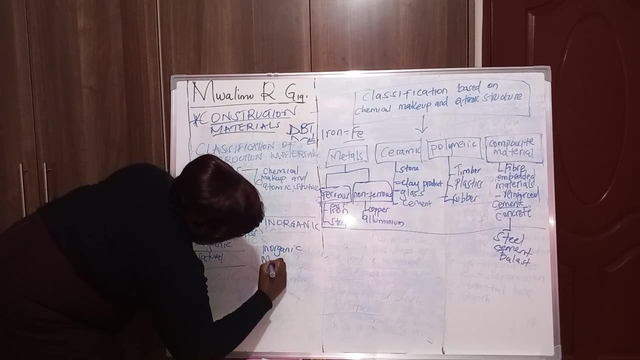 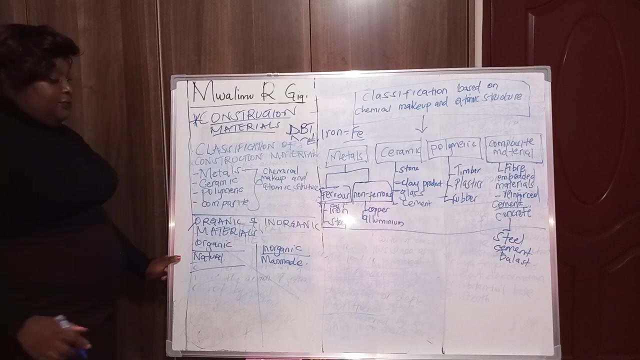 materials, they exist naturally on the earth surface and for inorganic materials they are, they are man-made. okay, so it's like natural and man-made. so organic materials, they are natural materials, they exist naturally on the earth's surface. and inorganic material, they are actually man-made materials. so we can list examples, examples: you can draw a table like that and 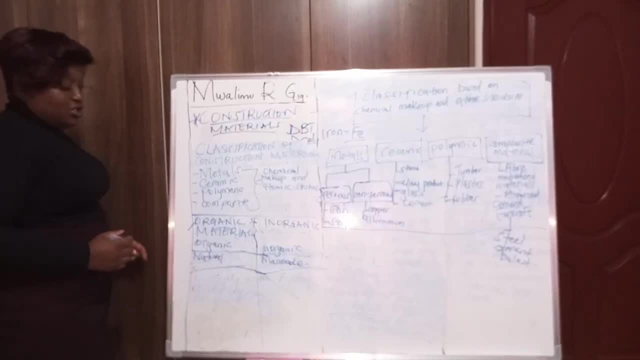 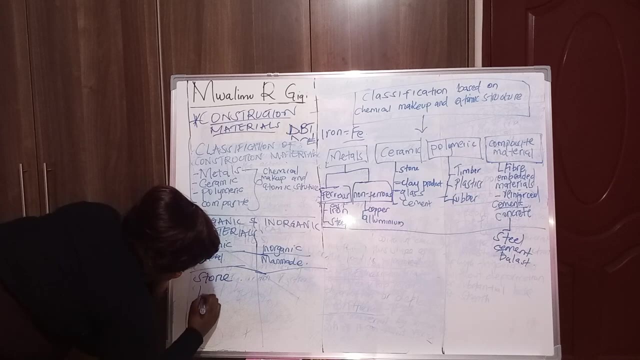 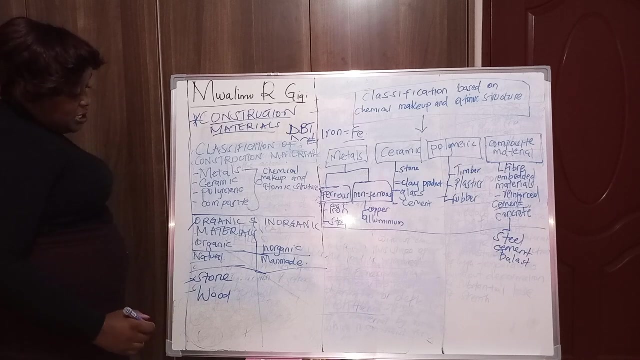 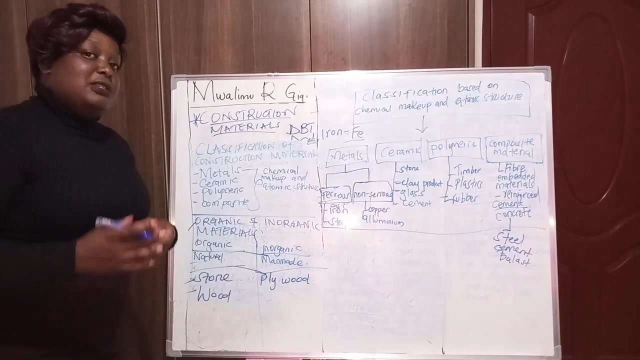 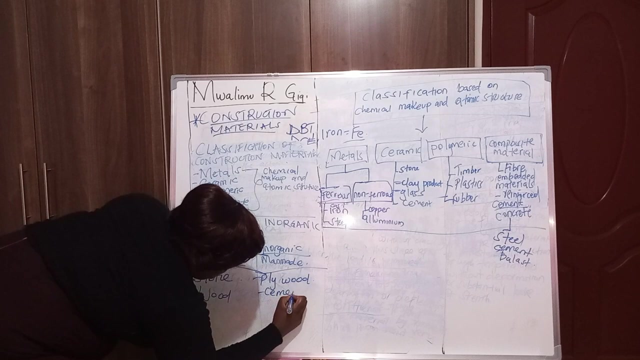 and differentiate some of them. so, organic material: we can have a stone and wood, wood, stone and wood. and for inorganic material- an example- we have plywood. this is wood that has been taken to the factory and we have made plywood, and then we can have a cement, uh-huh. 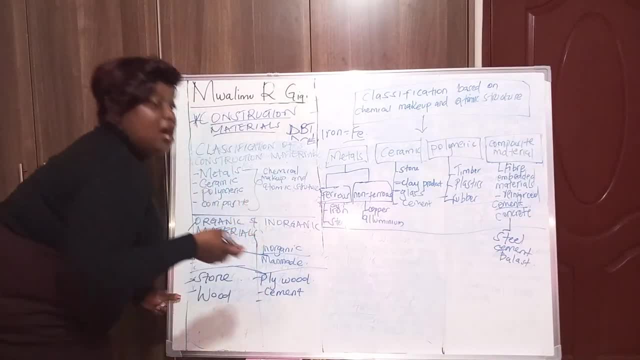 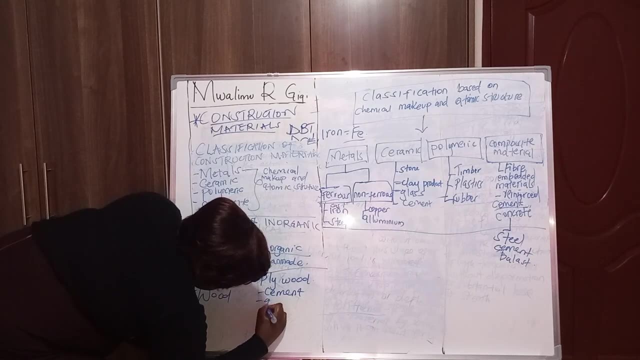 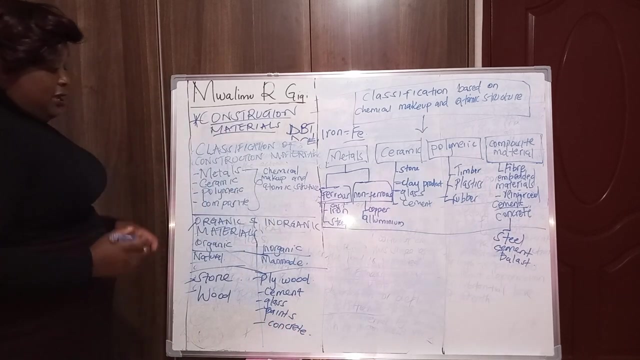 this is man-made cement. we have like baburi cement. we have a factory for making cement. we have our glasses. we also have glasses. we have companies that make glasses. we have paints. we can have concrete. we make concrete each and every day: a mixture of sand, cement and water. 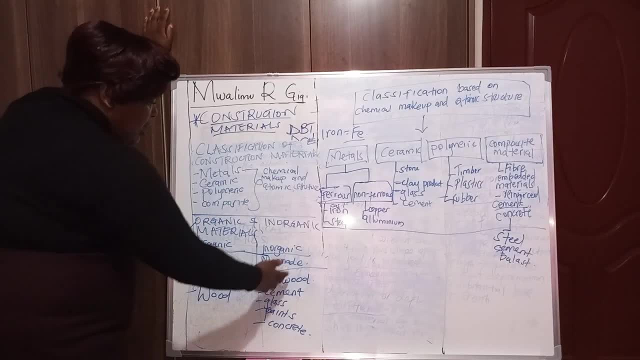 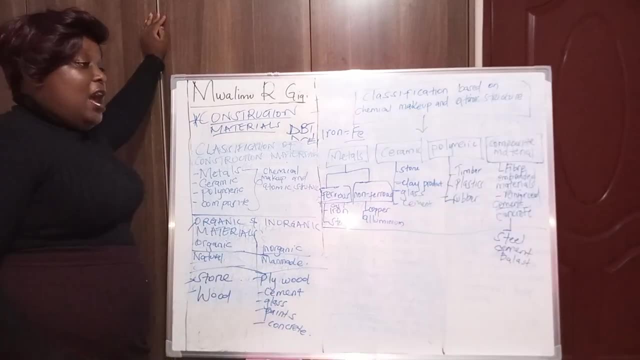 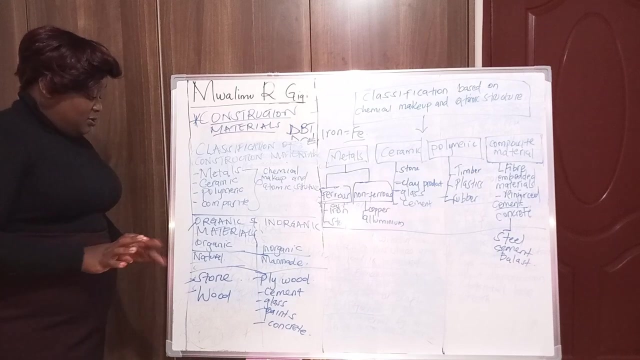 and some ballast. so these are just examples of inorganic materials which are man-made. we have plywood, cement, glass, paints and and many, as the list is longer. but for natural they exist naturally on the earth surface. so we have stone and wood. so the last subtopic we are going to, 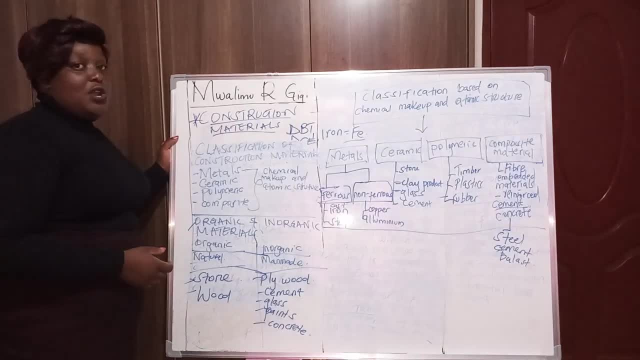 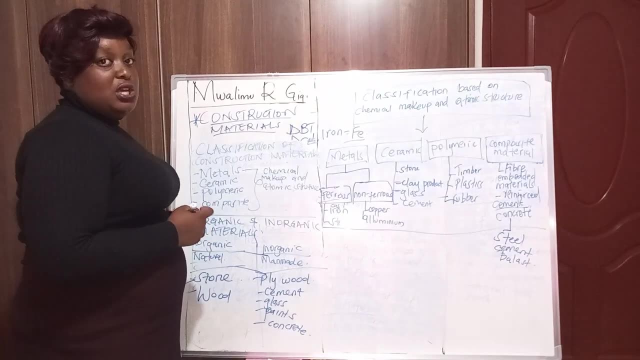 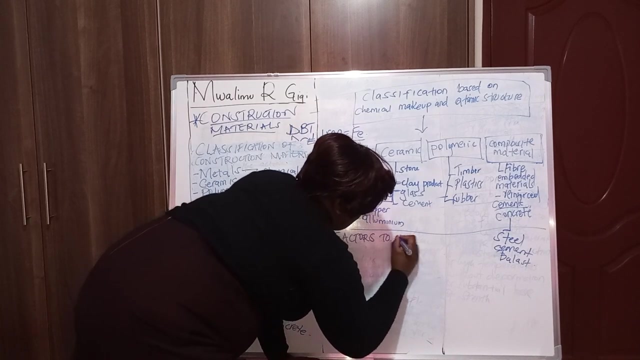 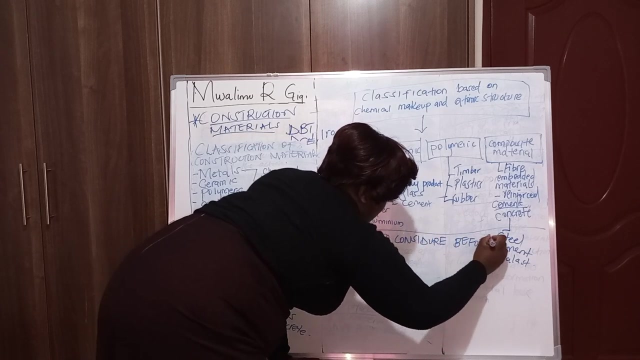 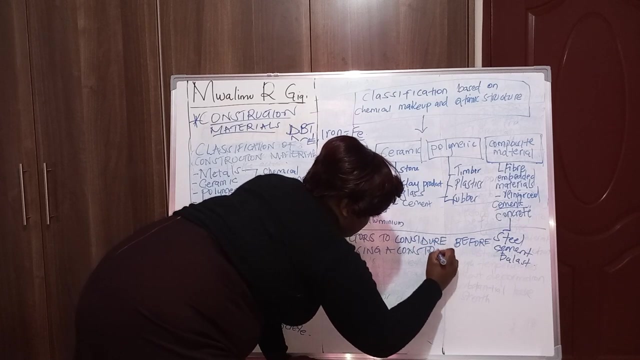 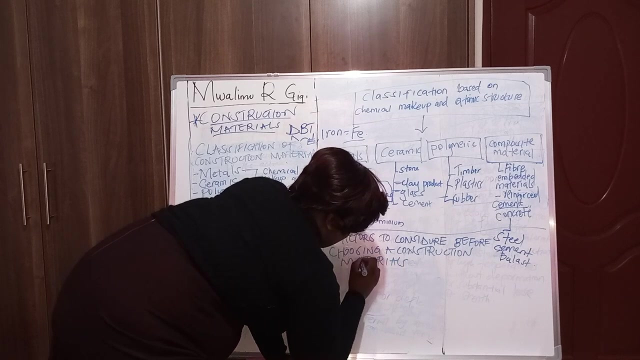 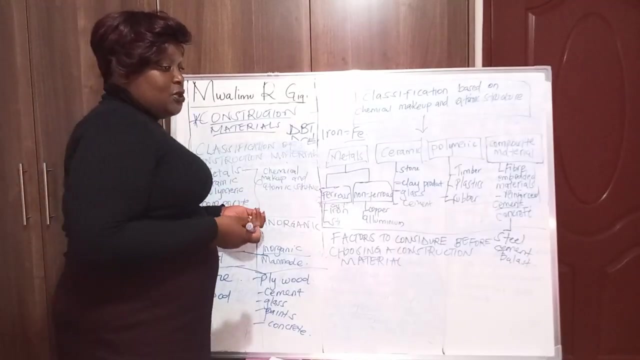 look at. in this topic of introduction to construction material, we have factors to consider before choosing a construction materials. so factor factors to consider before choosing a construction, a material. so what are these factors before choosing a construction material? so what are these factors? so we can have the first factor as 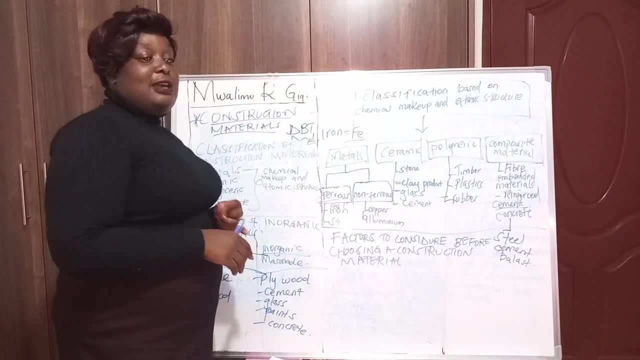 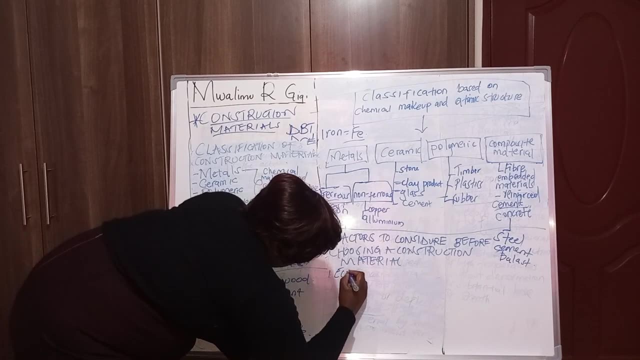 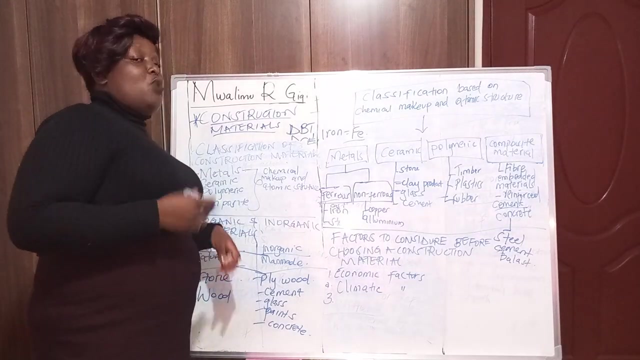 the economic economic factors. is there the capital? yeah, uh-huh. so the first one, we can say economic economic factors. number two, we can say climatic. number two, we can say climatic factors. climb uh clay matic factors. climb uh clay matic factors. is the climate suitable for our material to? 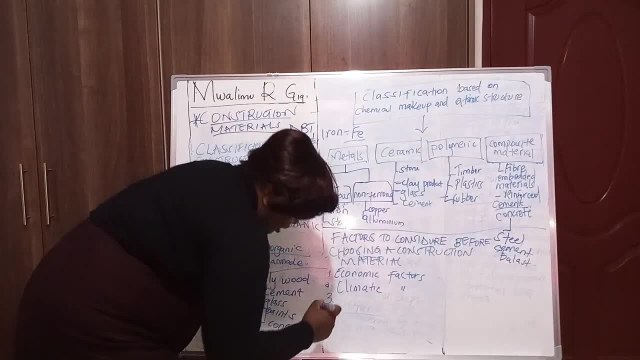 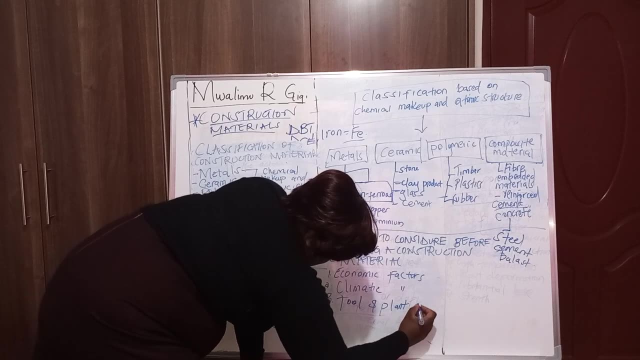 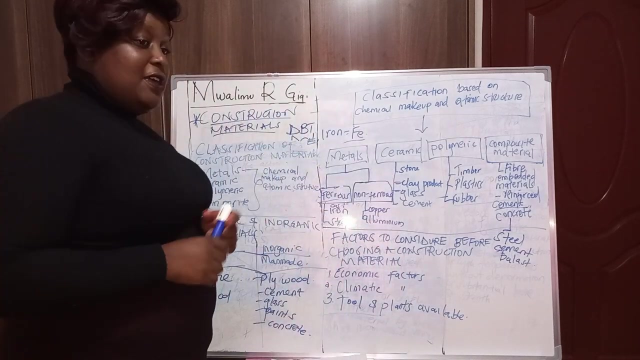 is the climate suitable for our material to work well, work well. so, uh, we can look at climatic factors and so, uh, we can look at climatic factors, and we also have. we also have tools and plants. are available tools and are. we also have tools and plants are available. you have the necessary tools. 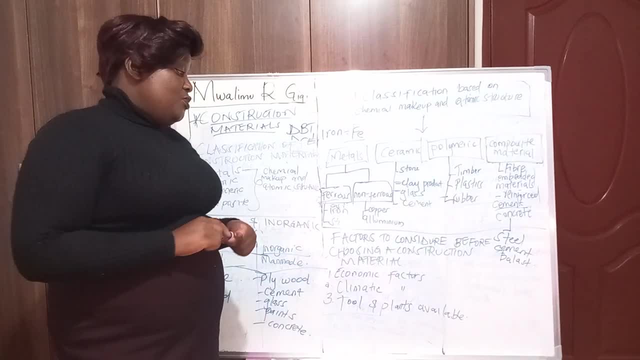 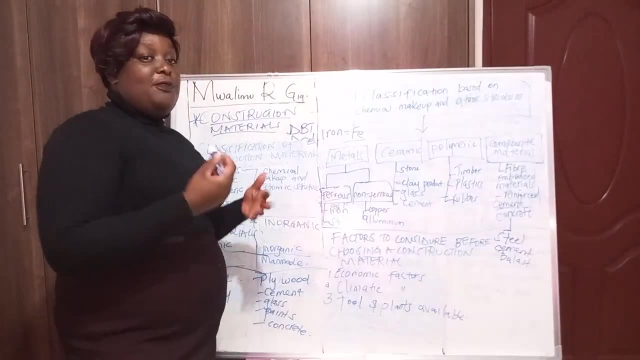 available. you have the necessary tools or the required tools or the required tools for uh for choosing that type of, for uh for choosing that type of construction material, and the list is construction material and the list is normal. we can also say that the type of normal. we can also say that the type of building or the type of 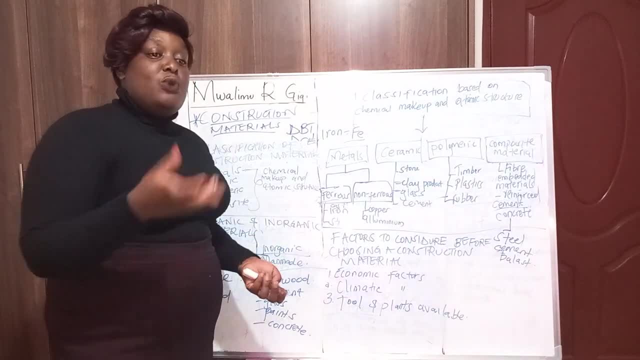 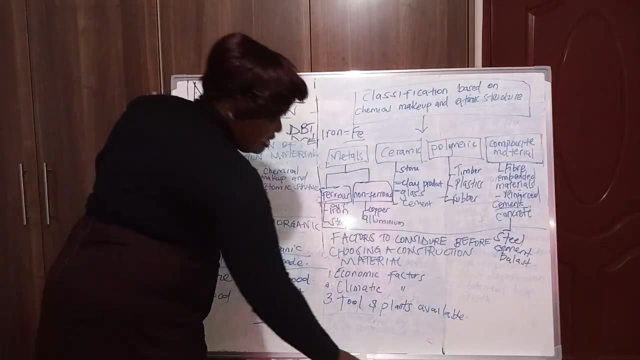 building or the type of work that you want to do. if it's for work that you want to do, if it's for railway works or uh, for road work, so railway works or uh for road work. so we also have many things. so we also have many things. so those are just uh, but i'm just going to